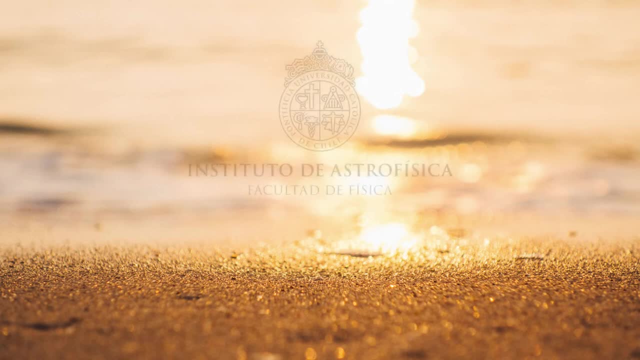 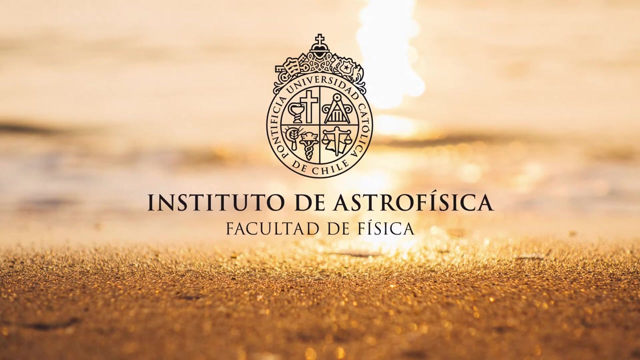 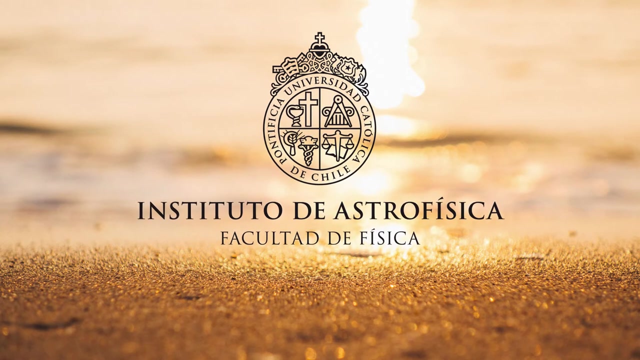 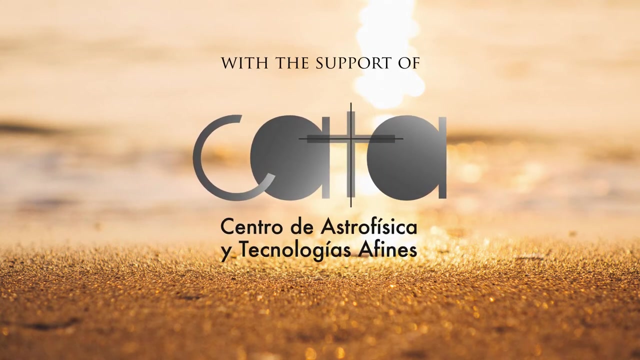 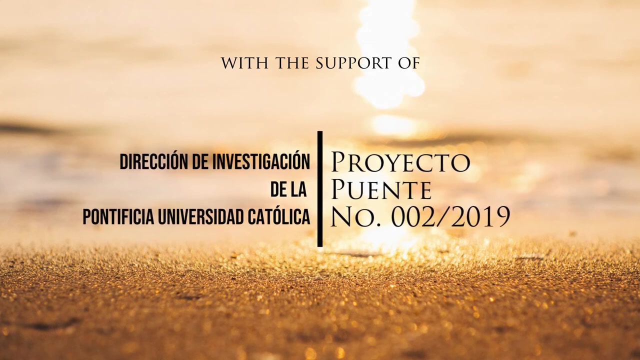 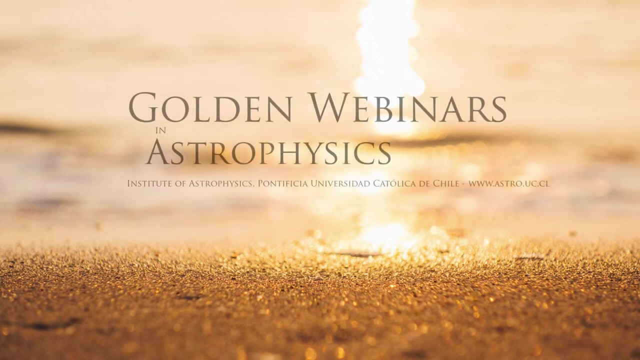 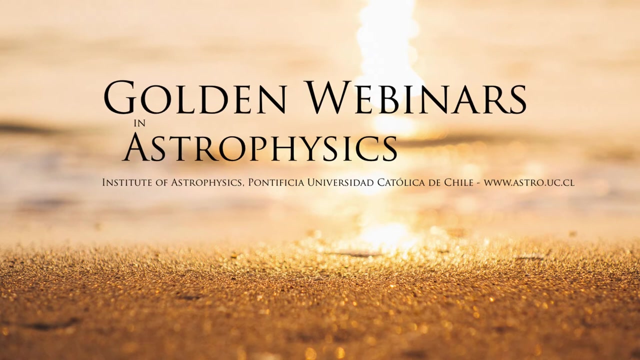 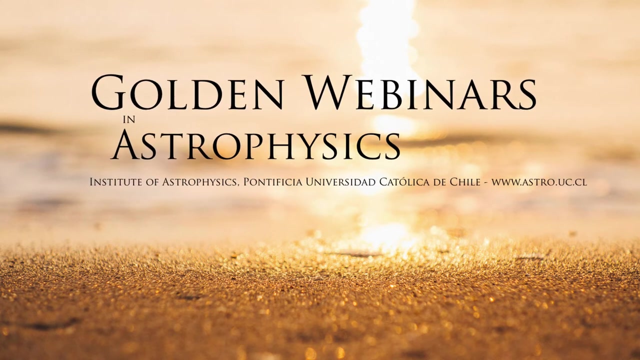 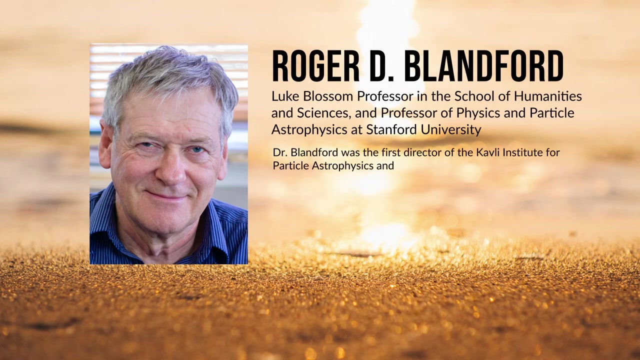 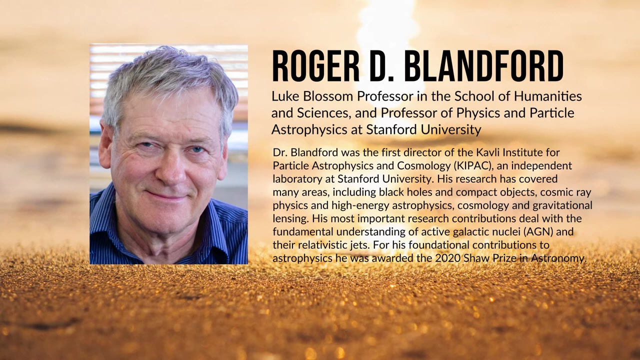 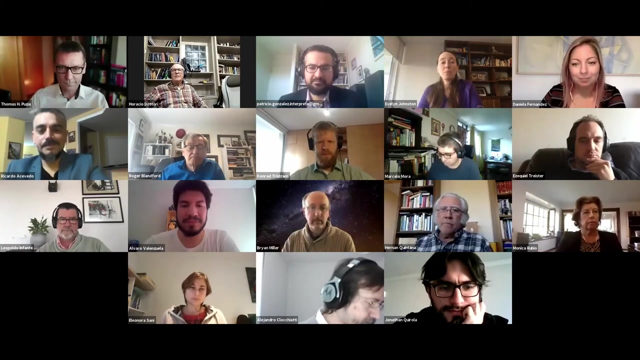 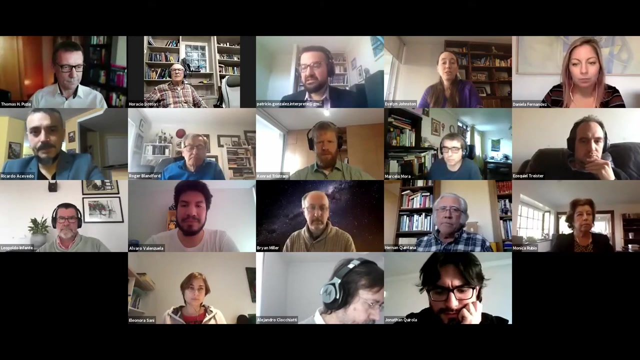 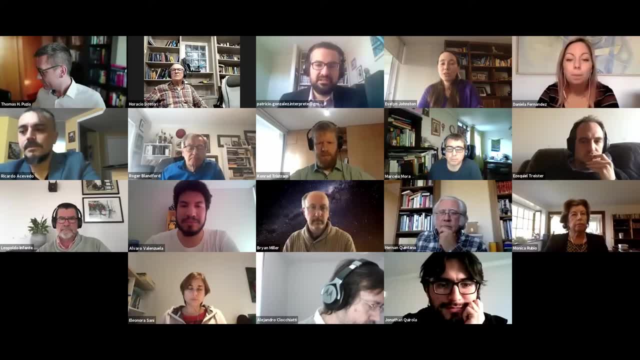 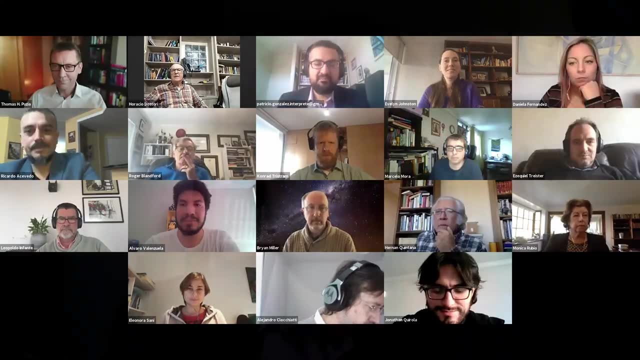 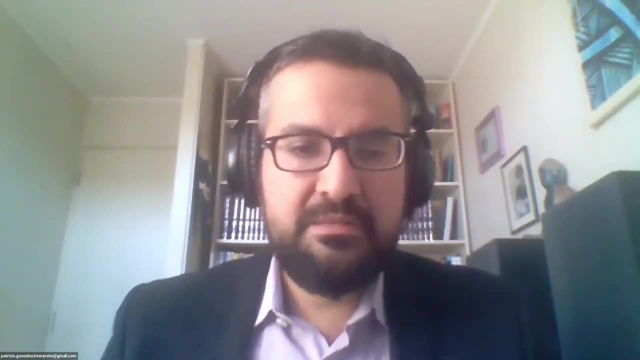 the English and Spanish to English directions. He will now give a brief explanation in Spanish as to how to change the language for this talk, and then we'll enable the interpretation option. Okay, Así que bienvenidos todos. Para poder escuchar la interpretación al español, hay un botón en la parte inferior. 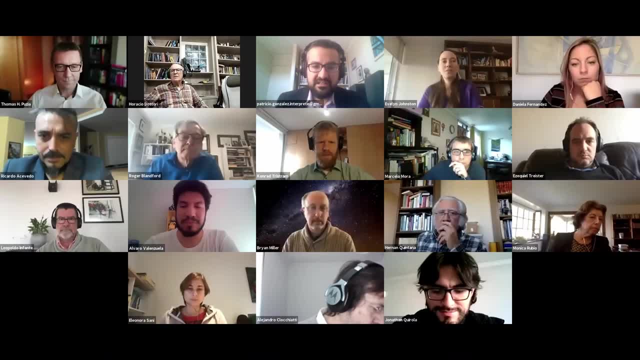 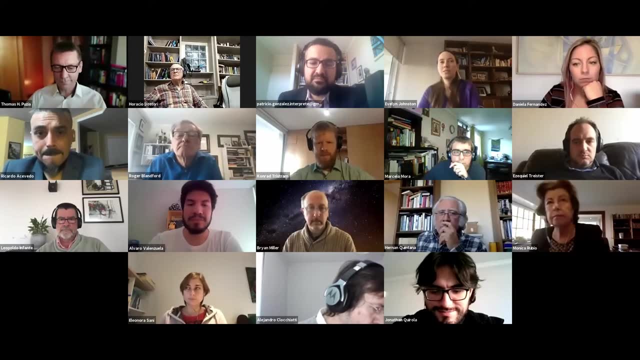 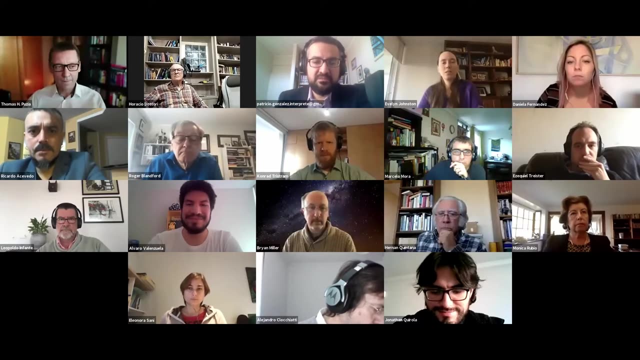 derecha de Zoom, donde lo presionan, y de esta forma pueden seleccionar la interpretación pinchando el botón español. Esto además le permite cambiar la pista de audio de la conferencia entre inglés y español. Desafortunadamente, la opción de interpretación en vivo no está disponible para las personas. 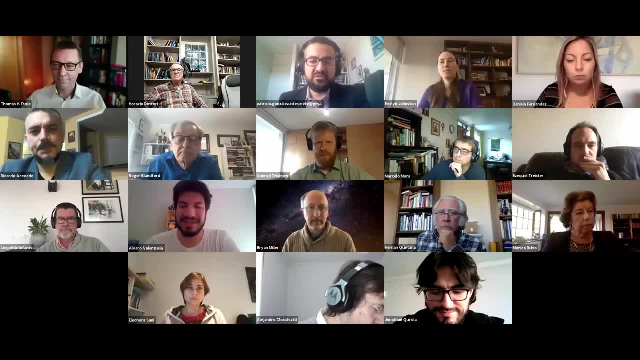 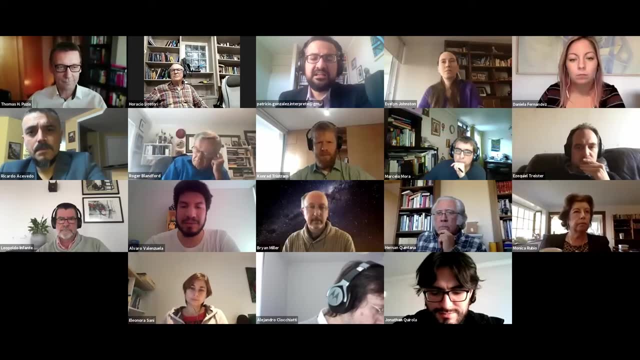 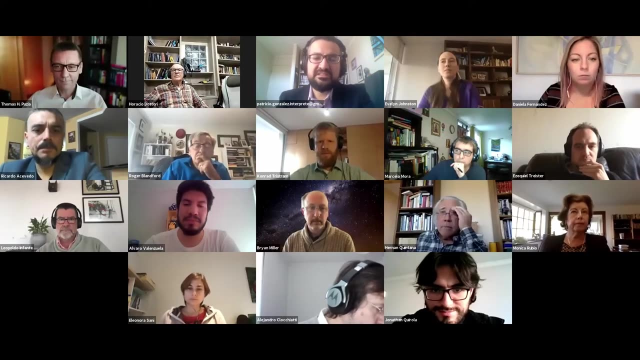 que utilizan Zoom en el navegador o las computadoras con Linux. Les pedimos disculpas por esto y pronto publicaremos las versiones en inglés y español de la charla en el canal de YouTube. También sabemos que algunos participantes no pueden silenciar la pista del sonido original. 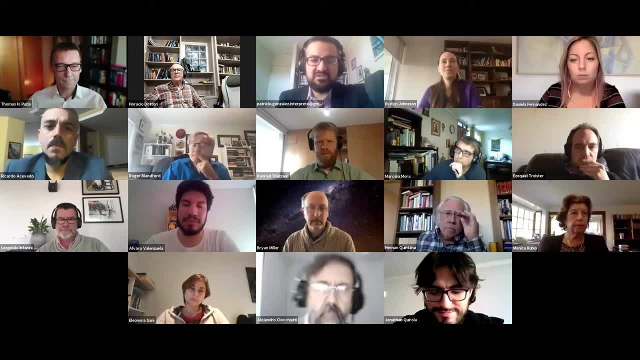 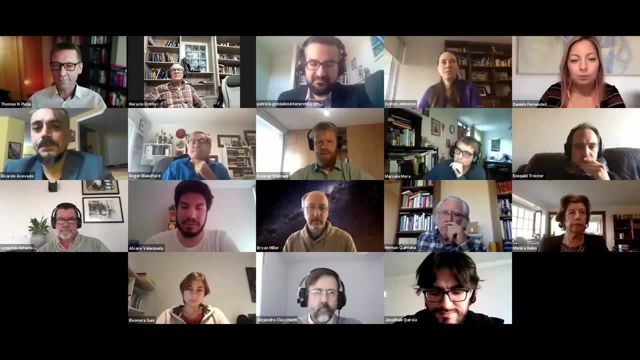 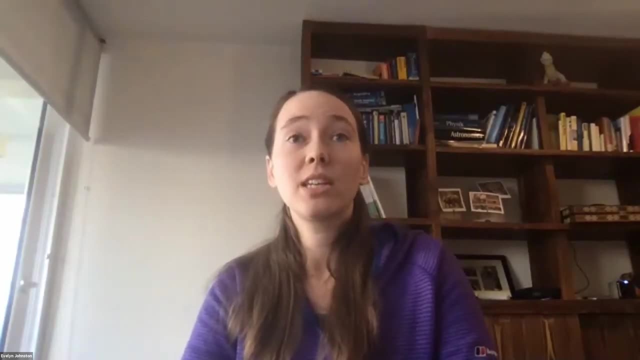 al escuchar la traducción al español. Esto es un error en Zoom, por lo que al salir y entrar nuevamente a Zoom, se arreglaría el problema. So welcome again. My name is Evelyn Johnston. I'm a postdoc at the Institute of Astrophysics at the Pontifico Universidad Católica and 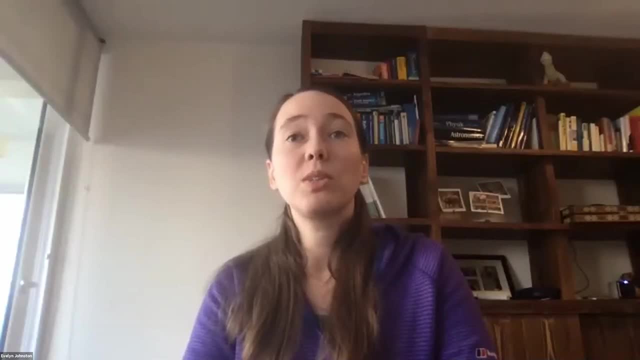 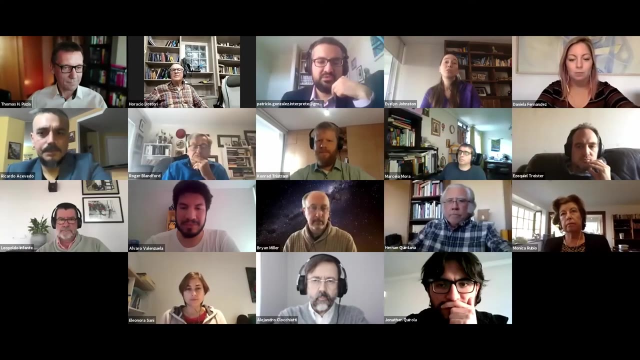 together with Thomas Puzia, a member of our faculty and head of outreach. we will keep organising this series of talks for as long as we can. First of all, we'd like to thank you all for the overwhelming response and encouragement that we have been receiving. 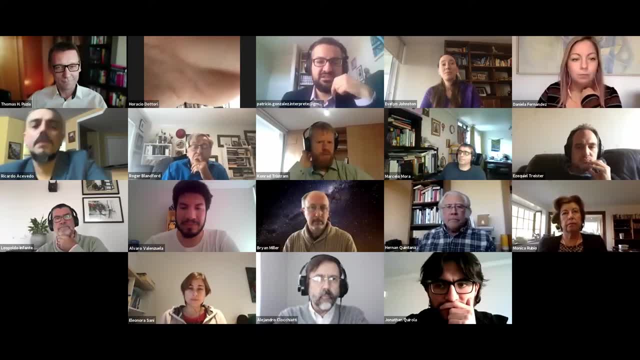 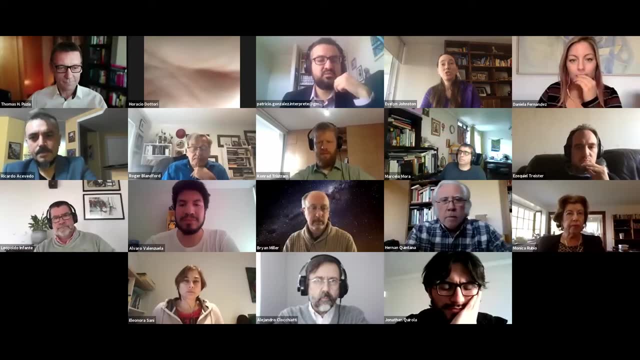 We really appreciate your comments and suggestions, so please keep them coming. We will continue to bring you these talks in the original English and with simultaneous Spanish translation, without any registration fees. This has been made possible by the generous support for the Centre for Astrophysics and 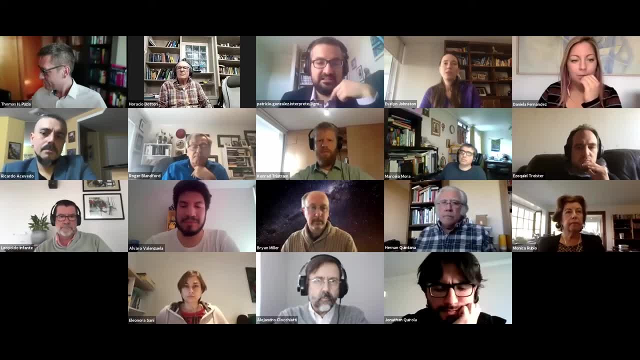 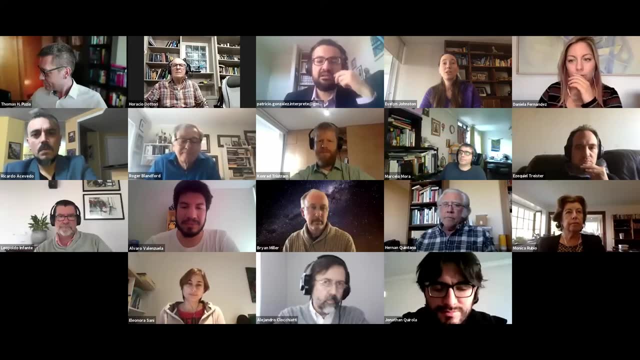 Related Technologies, also known as CATA for its Spanish acronym. Our talk this evening will be given by Roger Vazquez. Thank you very much. Roger Vazquez is the director of the Capley Institute for Particle Astrophysics and Cosmology. 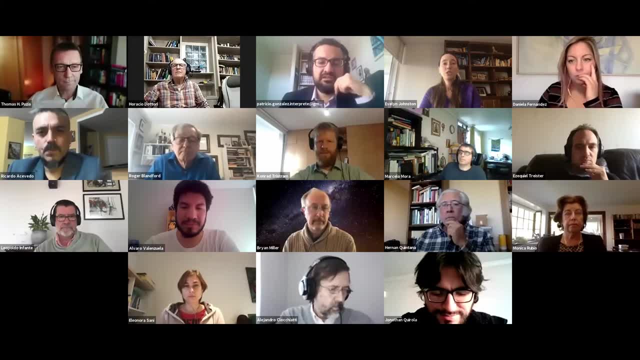 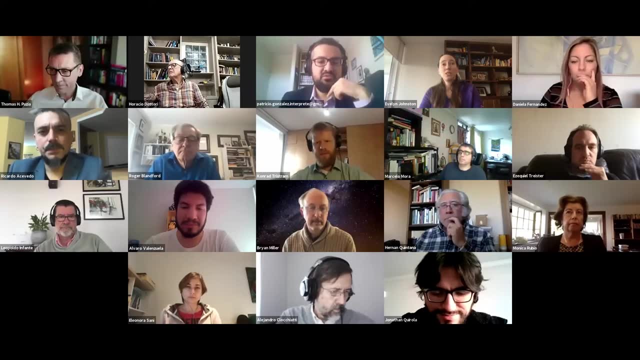 called CAIPAC at Stanford University. First, though, we'll give a brief introduction as to how the webinar will run. If you have any questions during the talk, please type them into the Q&A window. All viewers will be able to upload questions and comment on them, and we have a team of 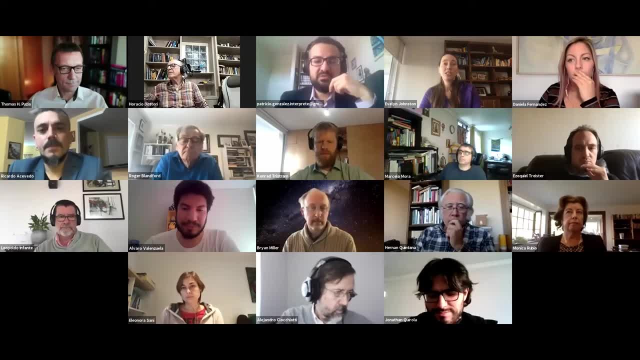 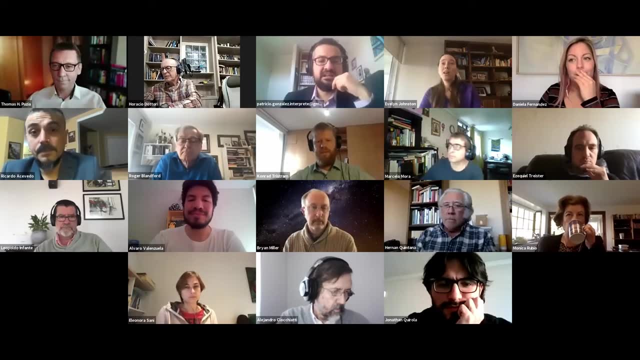 astronomers and journalists working behind the scenes, who will be monitoring your questions and will select the best questions for the discussion after the talk. The talk is expected to last for around 45 minutes and we'll have time for questions at the end. The questions from the audience will be selected only from the Q&A window and not from the 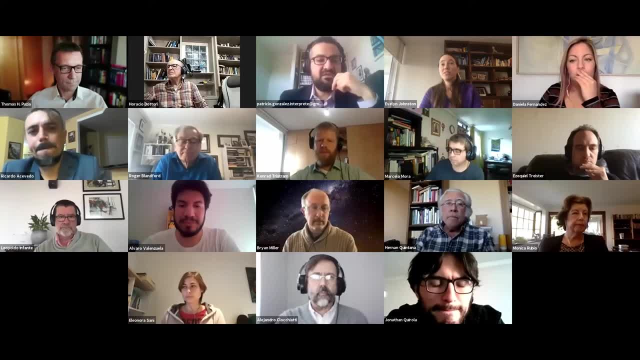 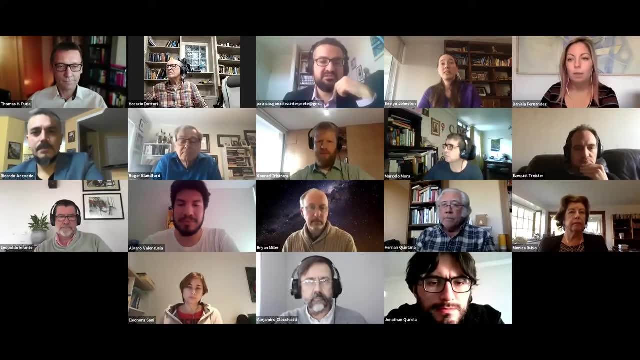 live stream on YouTube. Before we begin, I'd like to briefly introduce our other panel members who are with us today. We have Patricio and Thomas, of course, From our faculty at the Instituto d'Astrophysica. we have Ezequiel Treister, Alejandro Claciati. 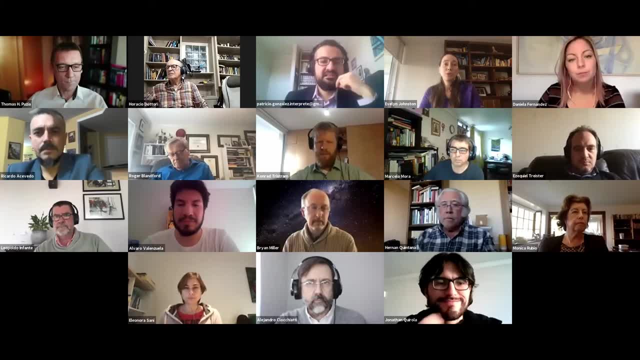 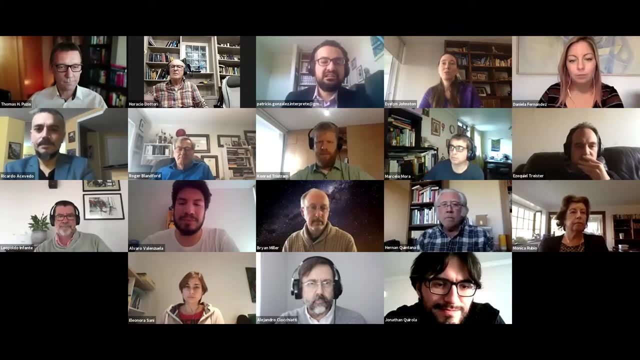 and Hernán Quintana. We also have some of our students and postdocs. These are Marcelo and Daniela. Thank you very much. Marcelo Moura, Jonathan Quirola and Alvaro Valenzuela. We also have the great pleasure to welcome our guest panelists this evening. 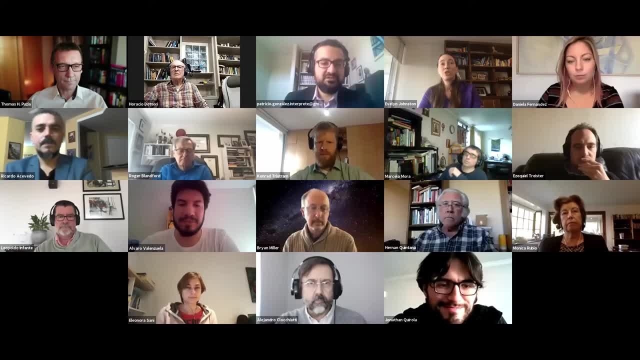 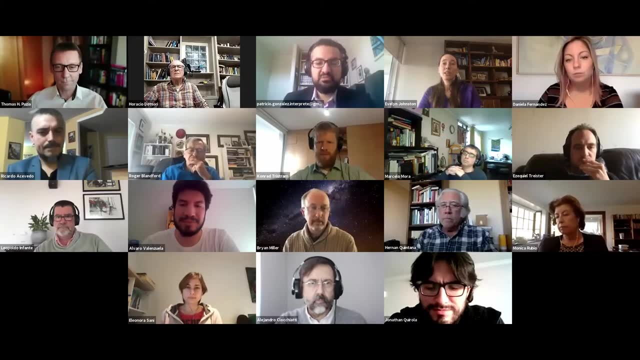 We have Monica Rubio, who is a professor at the Department of Astronomy at the Universidad de Chile. Brian Miller, who is an astronomer at Gemini Observatory. Leopoldo Infanta, who is director of the Las Campanas Observatory, again here in Chile. Horacio Dottori, who 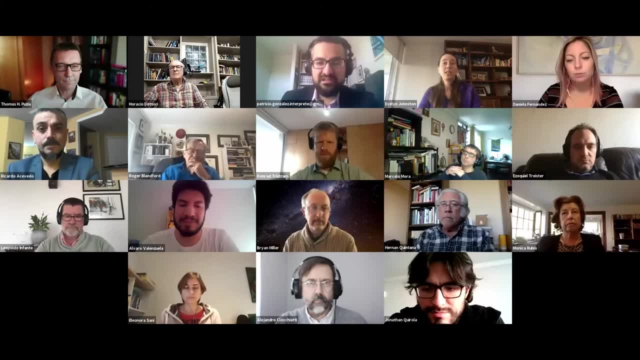 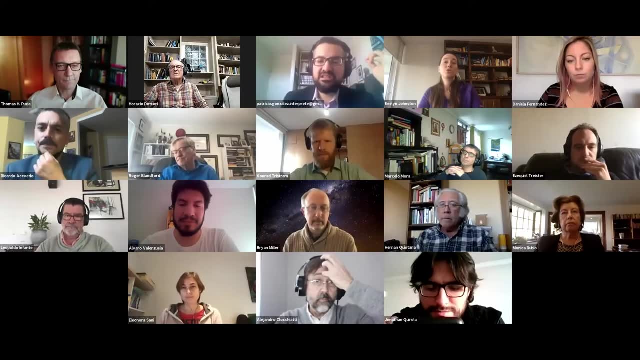 is Professor Emeritus at the UFRGS in Porto Alegre in Brazil. and finally, we have Conrad Lindström and Elia Norrissani, who are joining us as astronomers from ESO, the European Southern Observatory, who both work at Cerro Paranal. and, of course, we have our usual. 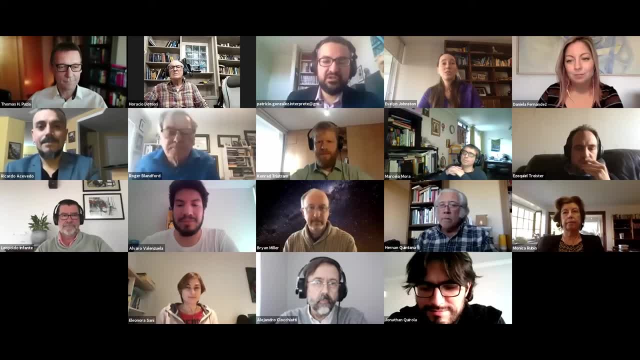 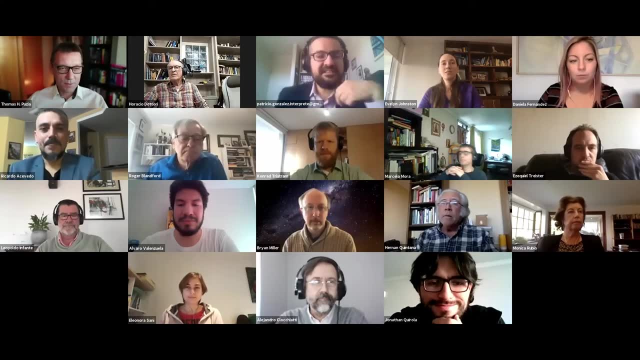 excellent team of Q&A managers- Ricardo Acevedo, Daniela Fernández and Carol Rojas. So it is our great pleasure to introduce Roger Blanford as our speaker this evening. Roger carried out his undergraduate and PhD studies at the University of Cambridge. 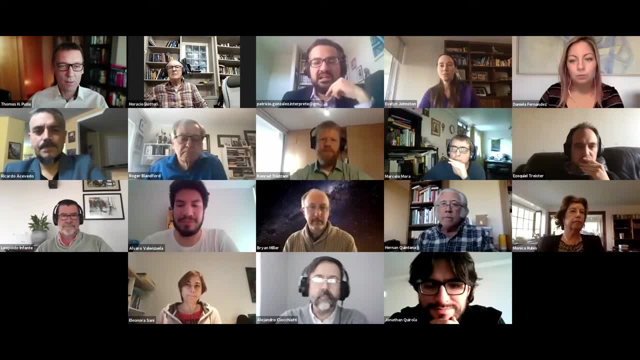 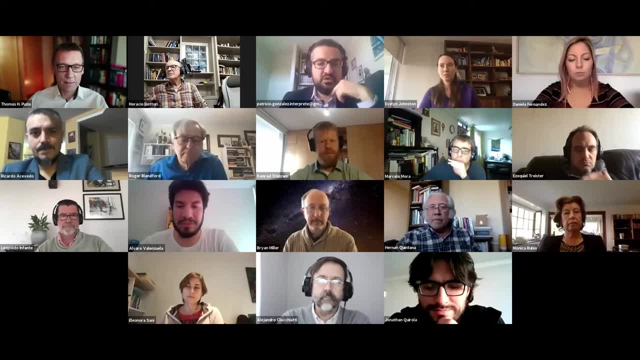 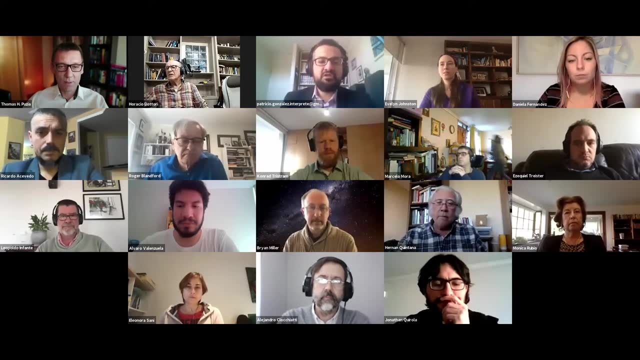 He joined the faculty at Caltech in 1976 and moved to Stanford University in 2003,, when he was appointed the first director of the Kavli Institute for Particle Astrophysics and Cosmology. He held this position until 2013.. 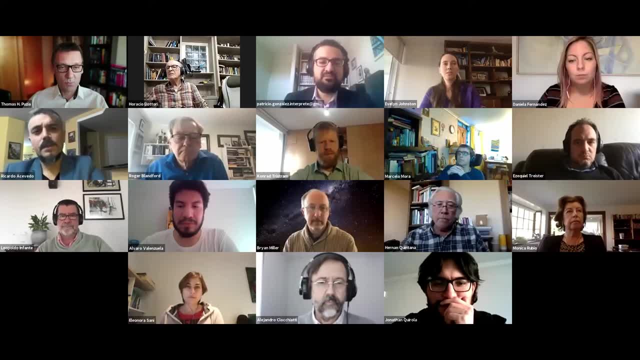 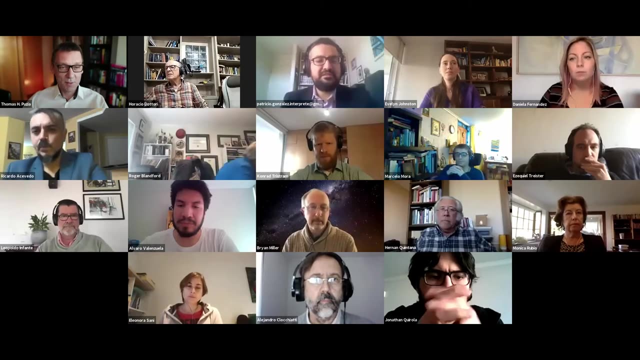 He is now the Luke Blossom Professor in the School of Humanities and Sciences at Stanford University. He has vermilion-rich expertise on the field of quantum mechanics and, moreover, a brilliant colleague for the Department of Physics. His research interests within astronomy and astrophysics are extremely wide and during. 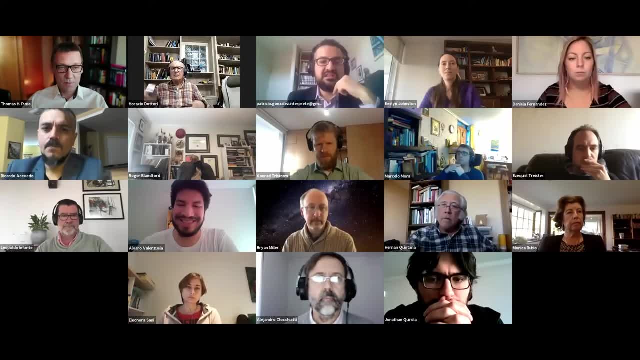 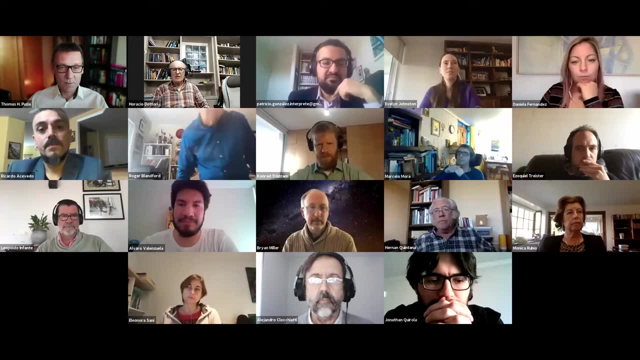 his career, he has focused on areas such as black holes, compact objects, cosmic ray physics and high-energy astrophysics, cosmology, gravitational lensing and gravitational waves. He established the Blanford-Znayek Process, which he, which is the leading model to explain. 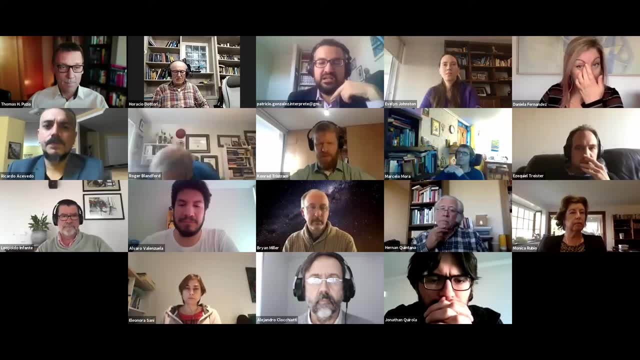 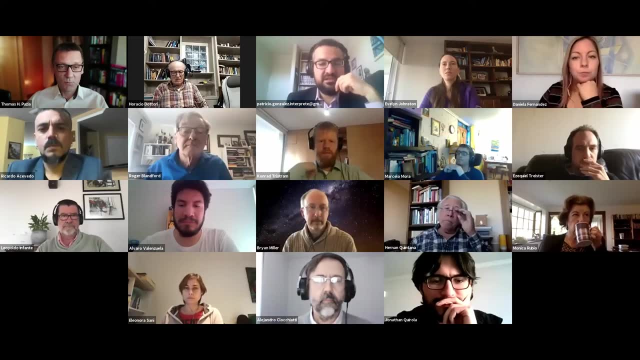 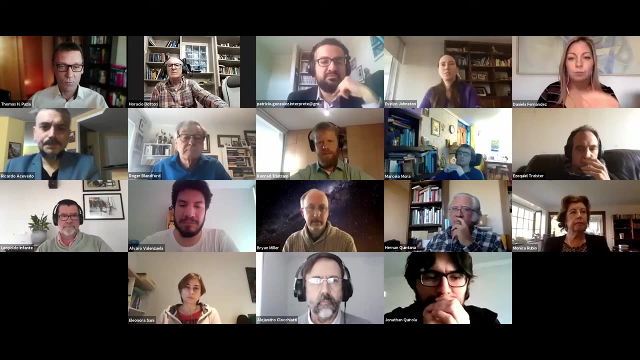 how energy can be extracted from a rotating black hole- The Black Hole. So this is the Black Hole: the production of jets of plasma that travel near light speed. Throughout his career, Roger has received many awards and distinctions, including, very recently, the Shaw Prize in Astronomy in 2020 for his foundational contributions to 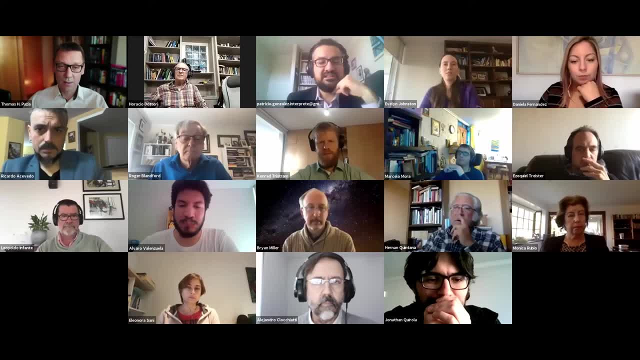 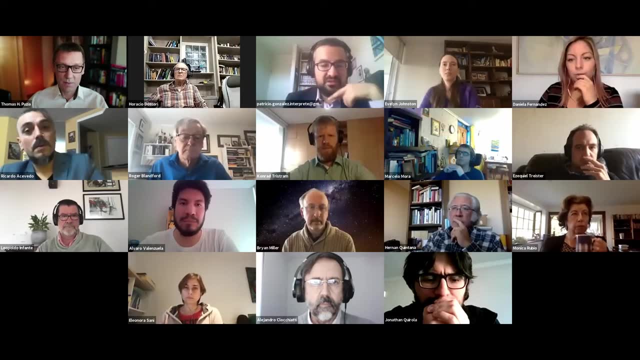 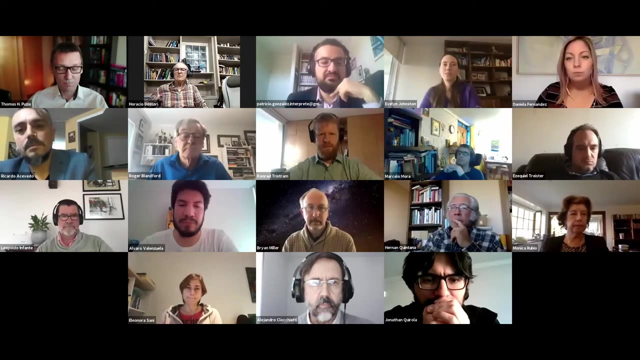 theoretical astrophysics, especially towards our understanding of active galactic nuclei, the formation and collimation of relativistic jets and the energy extraction mechanisms from black holes, as well as the acceleration of particles and shocks and the relevant radiation mechanisms. So we would like to 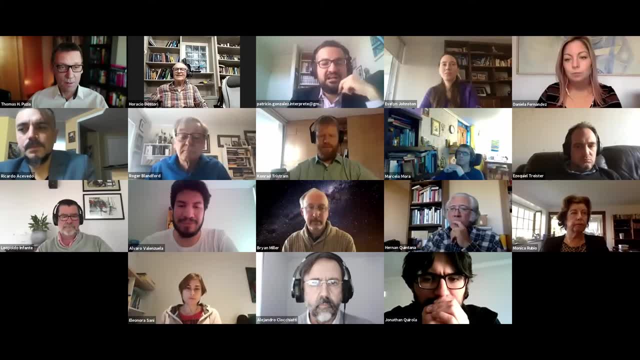 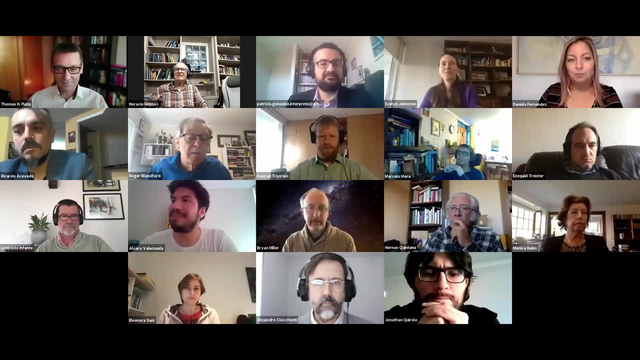 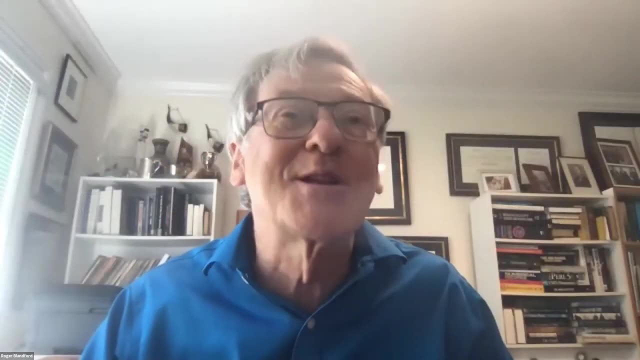 invite Roger now to tell us all about his work on the rotating black holes. Roger, please go ahead. Hi, can you hear me? Yes, I think the first task is to try and share the screen and I'll see how that works. 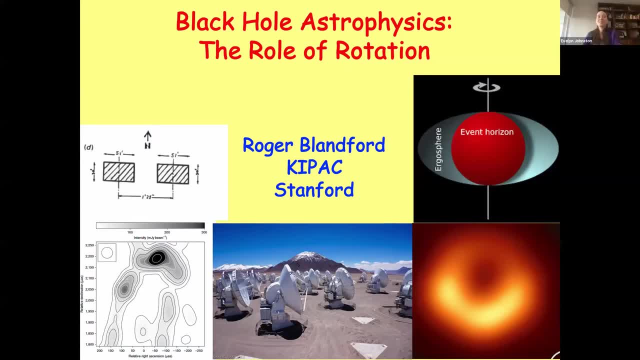 Can you see a PowerPoint slide? Yes, we can. Wonderful, Thank you very much. I have to start by saying how honored I am to be giving this talk and I'm very excited by the opportunity of talking to a large audience in this slightly strange. 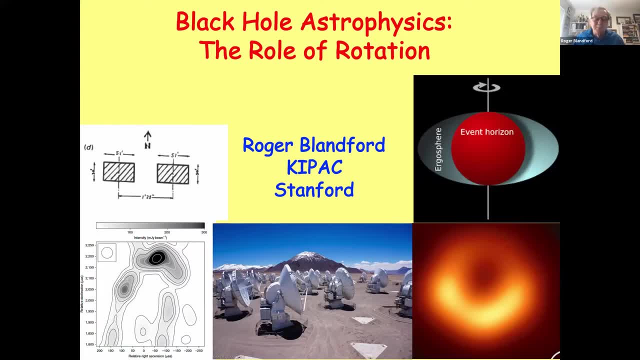 fashion- and I know your earlier talks have gone very well and I've been watching a few of them and I only hope I can get some of them right in the form of a press conference- can match up to the high standards that have already been set. 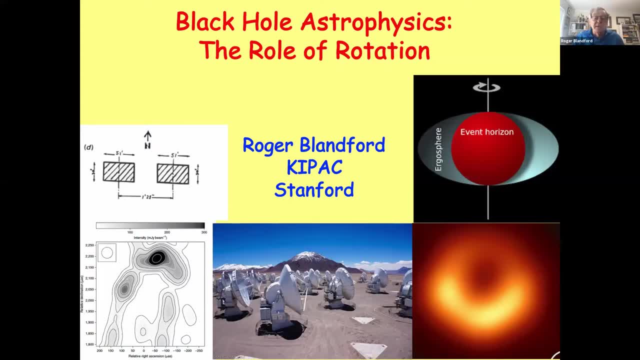 The topic that I want to talk about is black hole astrophysics and, in particular, the role that rotation of the black hole may play in what we observe, And I'm going to really specialize this further to talk about active galactic nuclei. 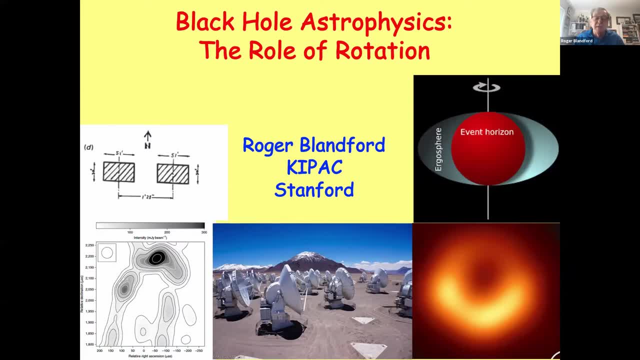 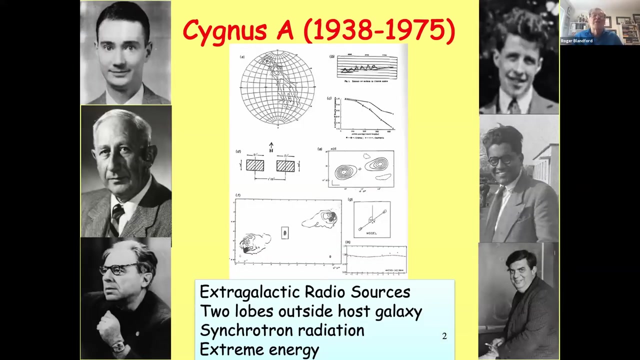 although I'll try and give some indication that I think these topics are actually much more generally applicable in modern astronomy. So let me move on, perhaps, to the first slide. Okay, so I'm going to start slightly historically, because the story really begins in the late 1930s. 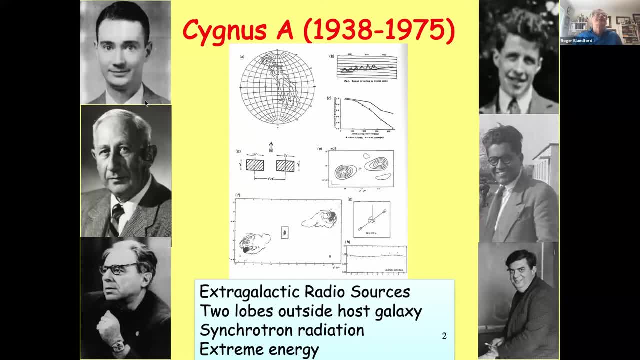 when this gentleman here, Grote Reber, I don't know. can you see my cursor on the screen? Yes, we can. Excellent, okay, so that'll have to be my pointer. He was an amateur astronomer in the United States. 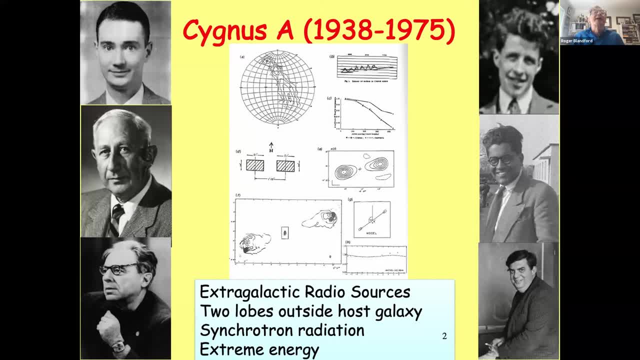 and he more or less developed the start of radio astronomy, and one of the brightest sources, which passed in fact overhead for him, was called, became known as Cygnus A. it's a radio astronomer, An extra galactic radio source. 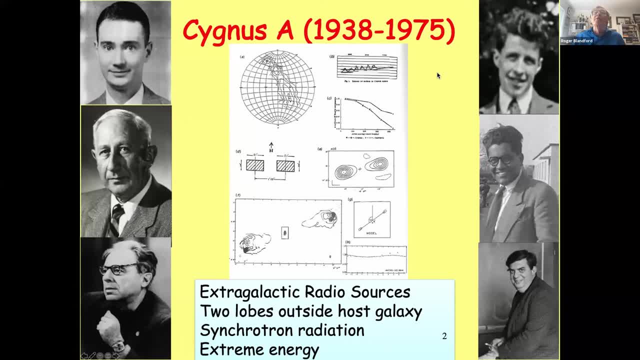 the techniques for radio astronomy developed during the Second World War and in particular, several people, including James Hay here, developed this further and were able to locate the source, and then it was eventually identified with a galaxy by Walter Barter and others here. 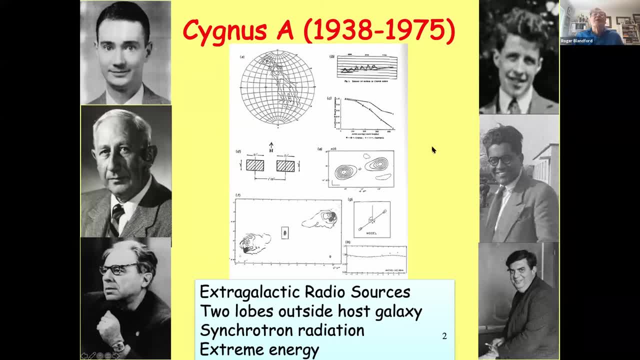 And then, in an early attempt at doing radio interferometry. this is a technique of using, you know, radio interferometry- more than one telescope to make an image of a source: Jenison and Dasgupta. and here's Dasgupta, here. 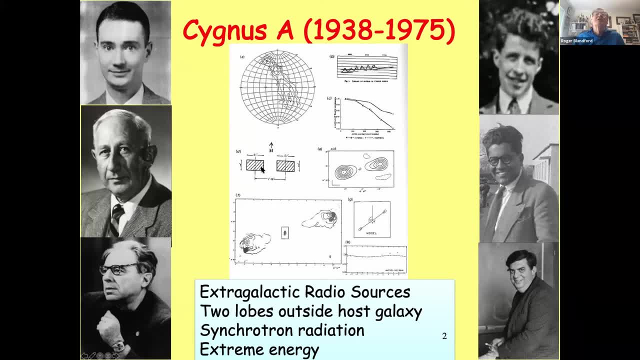 this is actually. they were able to show that this Cygnus A source was in two parts, and then eventually it became clear that the parts were on either side of the galaxy, and you'll see more of that As the years went by. the techniques of radio astronomy: 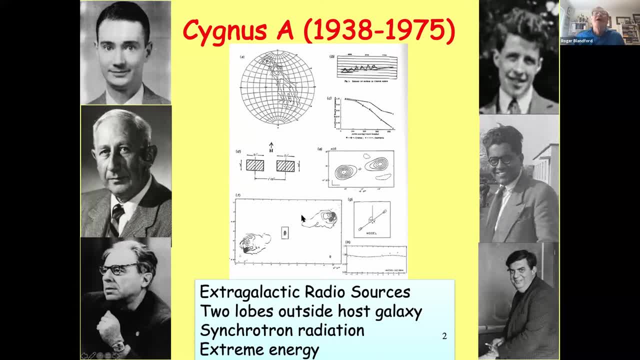 became more developed and the maps, as you can see here and you'll see further, became more and more sophisticated and before long we knew that not only were these two lobes of emission here, of radio emission here, but right at the center of the galaxy. 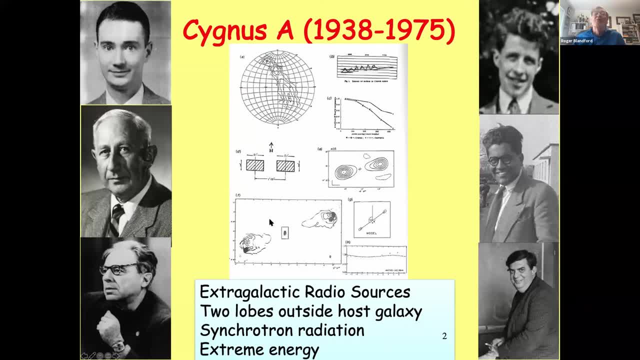 was also a compact radio source, and we'll see more about that. Meanwhile, the theorists got involved and there are many people who actually figured this out, but one of them is Igor Ishkovsky here- and he, amongst others, realized that the mechanism 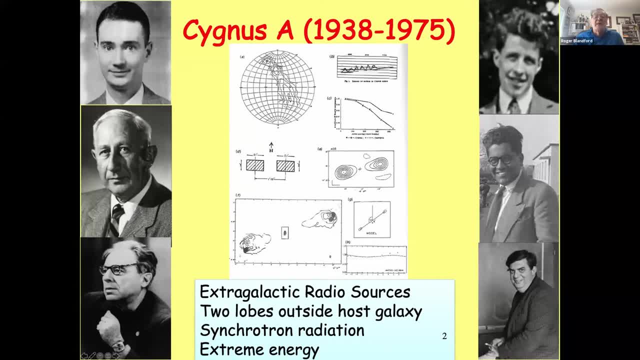 for making the radio waves was synchrotron radiation caused by relativistic electrons sparring in a magnetic field. and then Jeff Burbage here, an Englishman, was able to deduce a minimum value for the energies involved, and it was clear that the energies were at least as much. 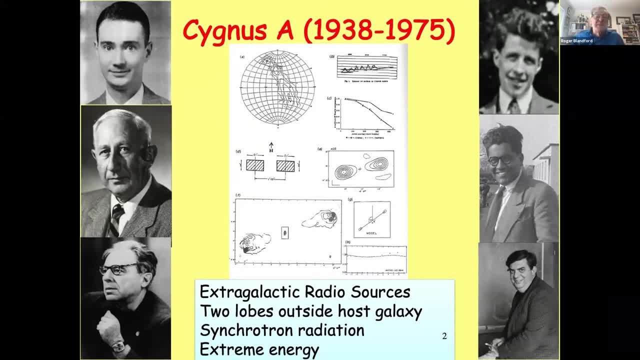 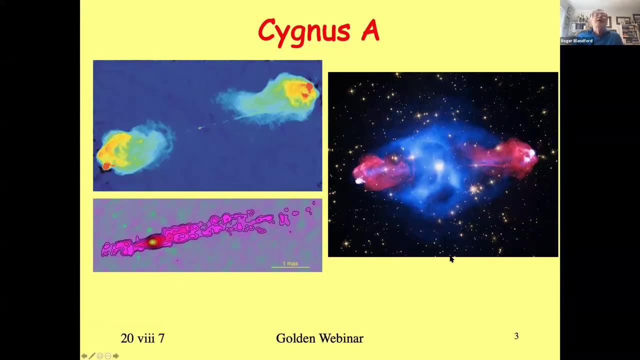 as you would get from the rest mass of, say in these big sources, 10 million suns. So they were hugely energetic and there was synchrotron radiation involved. So let's just move on to the next slide. Here's slightly more modern pictures of Cygnus A. 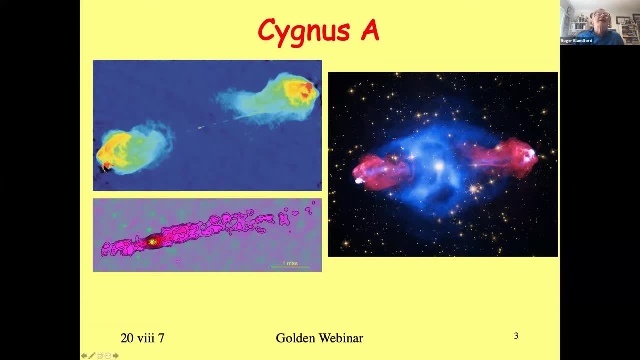 and one of the things you can see here, amplifying what I said before, is that there is actually a galaxy in the middle there, what an optical astronomer would call a galaxy, and then squirting out at the center. the very nucleus of this galaxy are two linear features. 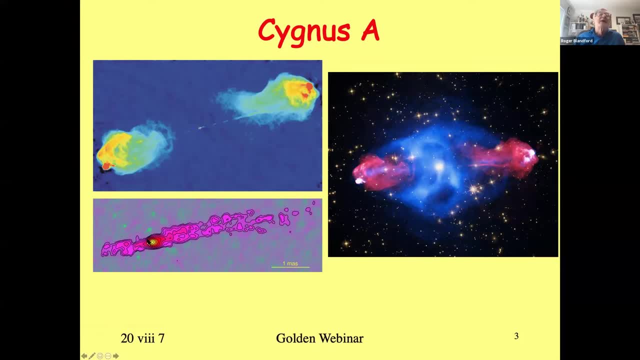 which we call jets. If we look at these jets with better angular resolution using the techniques of very long baseline interferometry- so this is using telescopes scattered around the world- then you can see these jets emanate from a source on a very, very small scale. 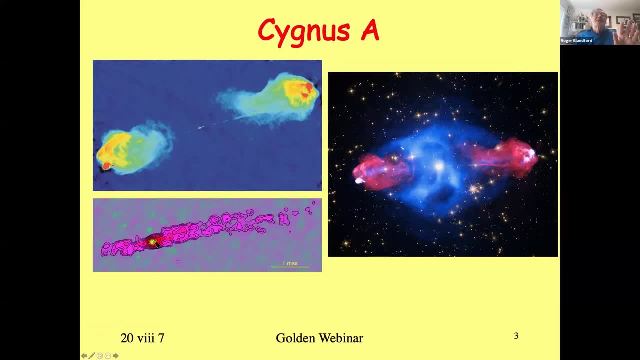 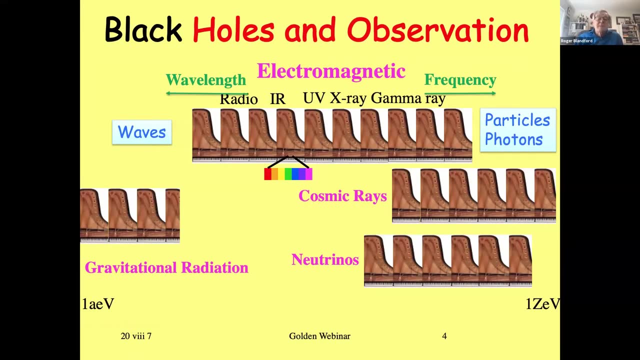 and we'll come back to that again. I interrupt this description of Cygnus A just by making one point that I always like to make in a talk like this: that what one has learned about these sources is not really just the gift of radio astronomers. 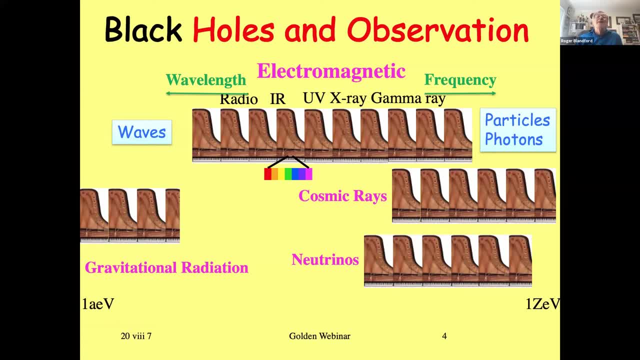 or the gift of optical astronomers and so on, but it's astronomers working together using the whole electromagnetic spectrum And, as I'm sure you all appreciate, they have at their disposal radio waves to gamma rays and, for some circumstances, neutrinos, gamma rays and cosmic rays. 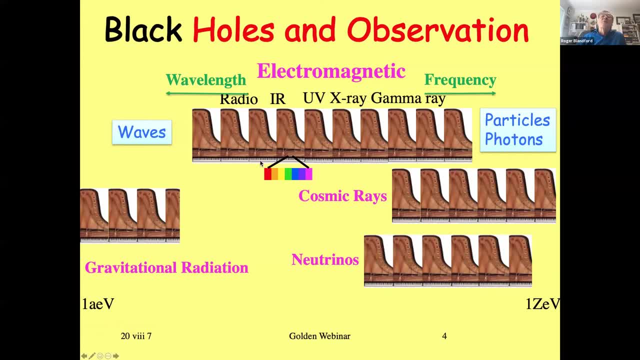 These are all part of my story here And what we see with our eyes is just one octave of grand piano, but we've got 140 octaves in total to explore and pretty well all of them are actually nowadays used and they're part of the story. 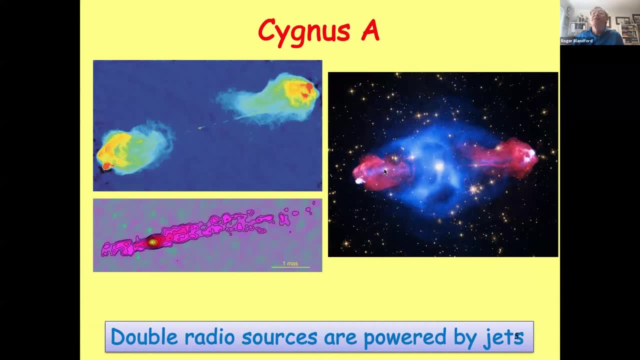 So let's go back to Cygnus A. Here we have Cygnus A again, and here we see another image, here in the red, Or you see the radio emission and then around it you can see in the blue. these are the x-rays. 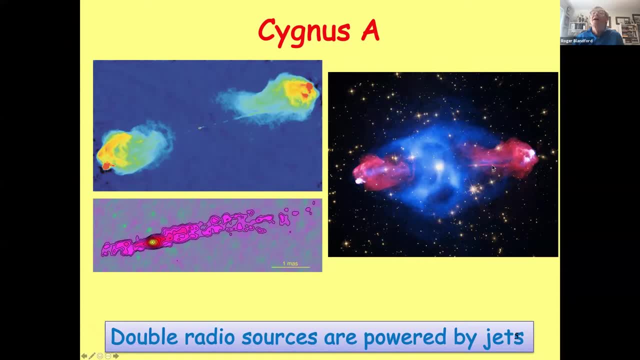 And then here in the white there's the optical galaxy and you can see the jets that come out of the middle, the center of the nucleus of this galaxy, and then power these enormously energetic lobes of radio emission on either side of the galaxy. 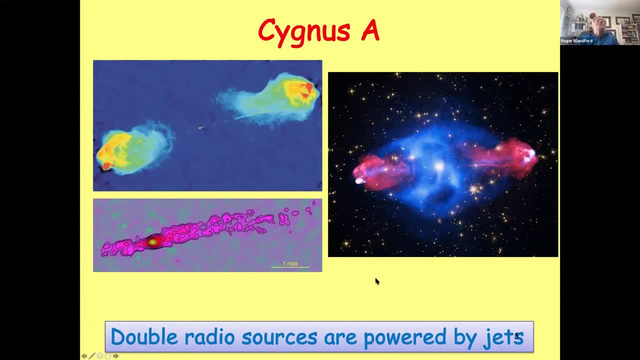 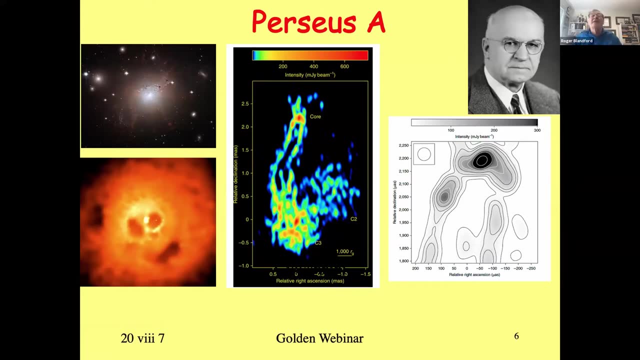 Moving onwards, here's another source famous in the history- And I've given a nod to Edward Fath, who was actually a student, I think in 1908, was one of the people who realized that those spiral nebulae. 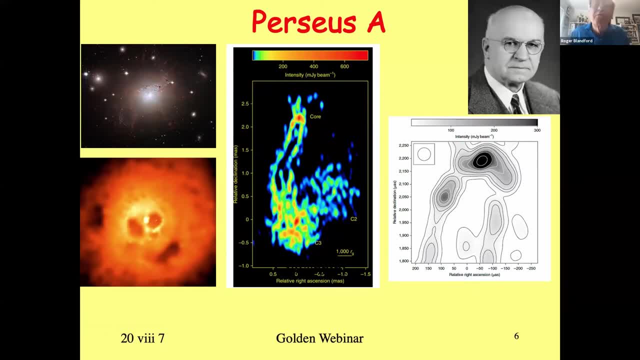 were in fact other galaxies containing stars, but also discovered that they had nuclei that, from an optical astronomer's point of view, had emission lines. So clearly there was something exciting going on in the nuclei of those galaxies, And one of the ones that he looked at. 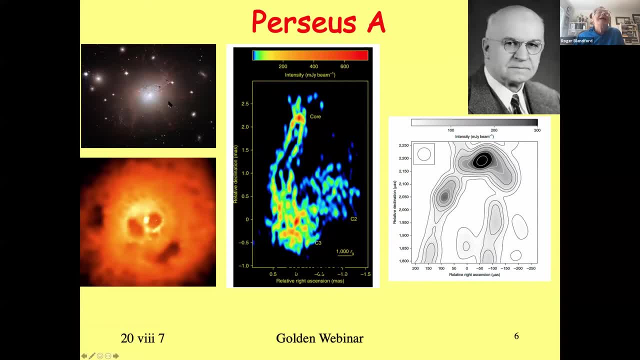 was not actually Perseus A, but it's another source that's very similar to it And, sorry, let me just go back that way And I want to show you some relevant observations, contemporary observations, from Perseus A, because they again are going to be part of our story. 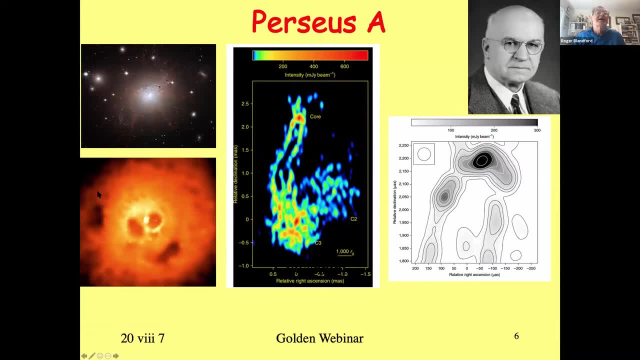 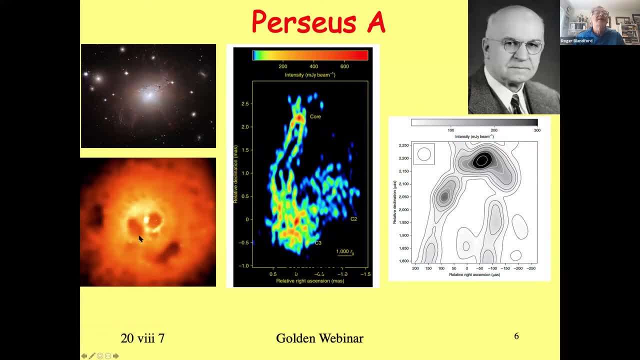 Some people say that this looks like a a star, but it's not. But what these dark features here are are the lobes of radio emission that have been inflated by activity in the nucleus of the galaxy, and those lobes of radio emission. 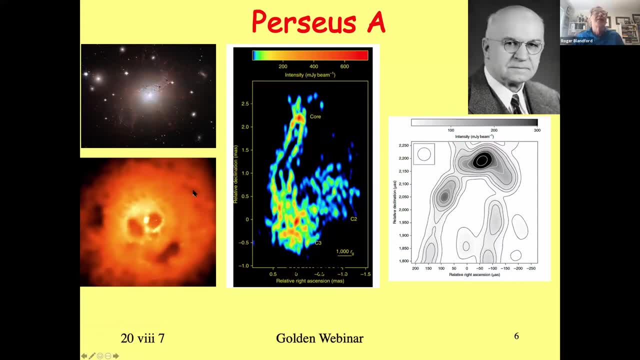 eventually become buoyant bubbles and they float upwards in the hot gas that's in the cluster of galaxies. And if we look on the smaller scale and try and understand the properties of those radio emissions properties and the imaging of the jets themselves. So if we start looking again, using very long 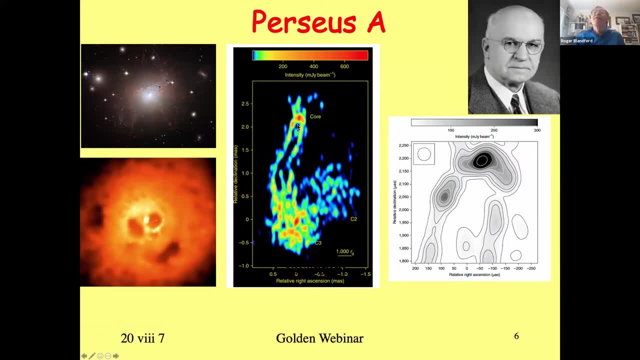 baseline interferometry including. in fact, in this case, some of the observations come from space. then we are able to see the nucleus of the galaxy- here, in this case, not so resolved- And then we're seeing the structure in these jets And one of the key things is that these jets 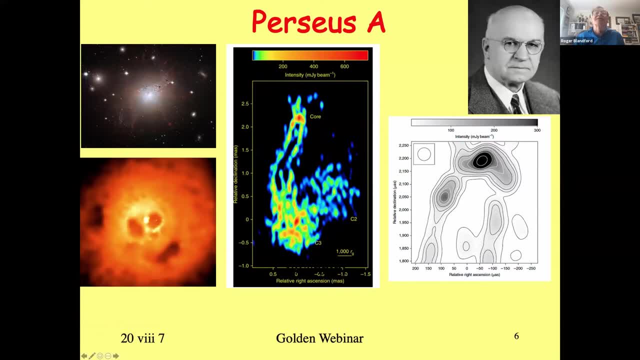 themselves. most of the radio emission shown in this image here seems to come from the walls of the jets. It's like an interaction or a boundary layer, that where this jet squirting out of the nucleus of the galaxy is interacting with its surroundings And it's that interaction. 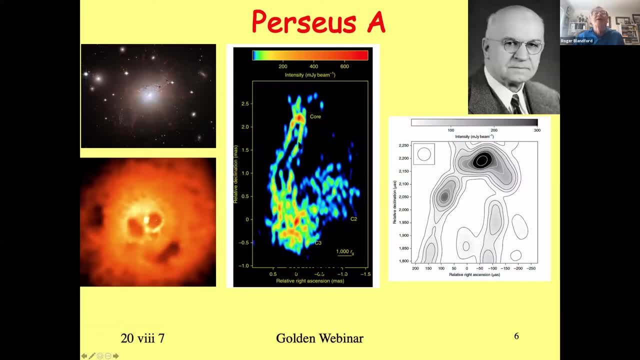 that is, giving you the relativistic electrons that are radiating, synchrotron radiation, for the gratification of radio astronomers. And so we have here the inner parts of one of these jets, And if we look on the very smallest scale, here too we can see these features here. And 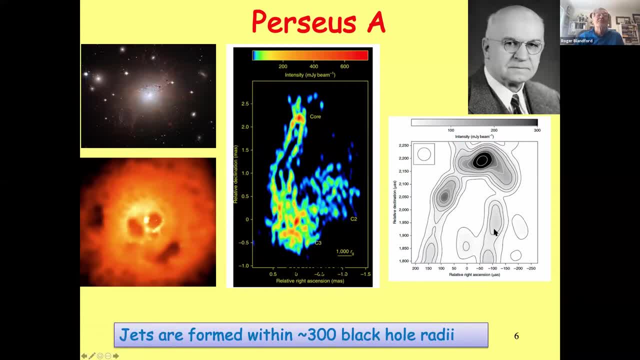 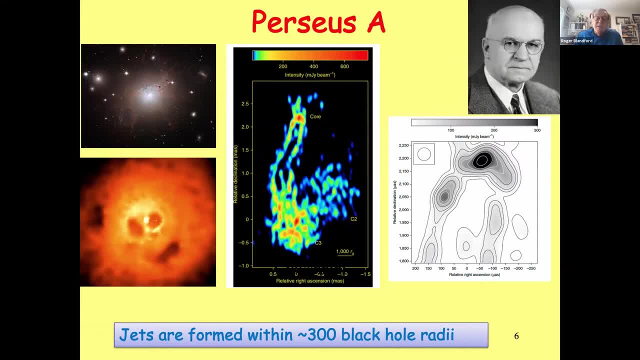 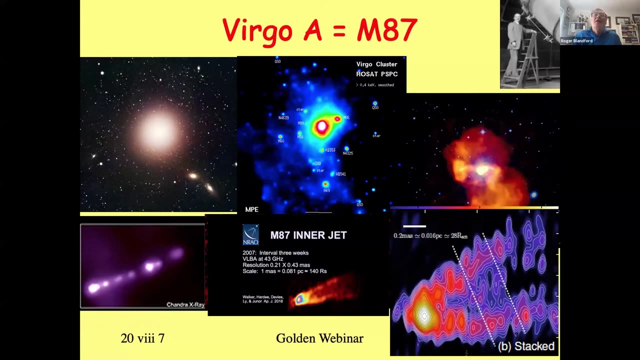 So really tiny structure. So I'll say a little bit more about that in a moment and talk about another source that is famous in the history of astronomy And that is Virgo 8, the old radio transmitter, sometimes nowadays called M87, more commonly, or M87 or 3274.. It has lots and lots of. 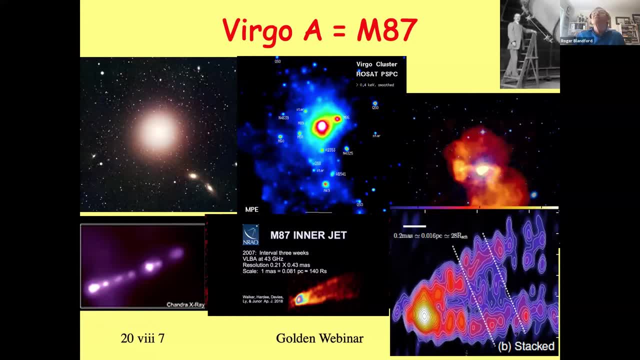 names, And this has, of course, been extremely famous for reasons that you know. In 1917, Heber Curtis, working using the same telescope, the Lick Reflector, as Edward Fath, discovered the first jet, And you can see it here in an optical image there. Well, this isn't his image, obviously. 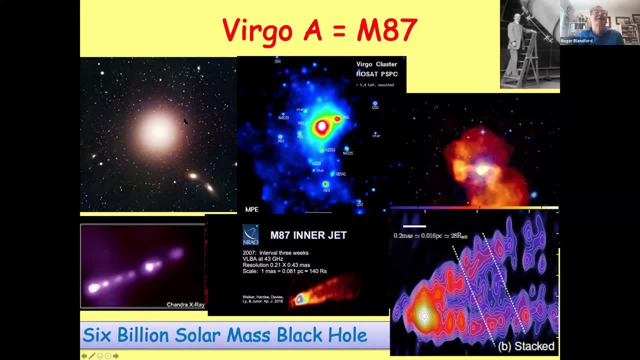 but he actually referenced it And this is the first jet that was discovered in the history of astronomy And he recognized the jet And this, in 1917 and 18, was the very first observation of such a thing. Again, we have the same pattern. It's in the clusters and that cluster gas is. 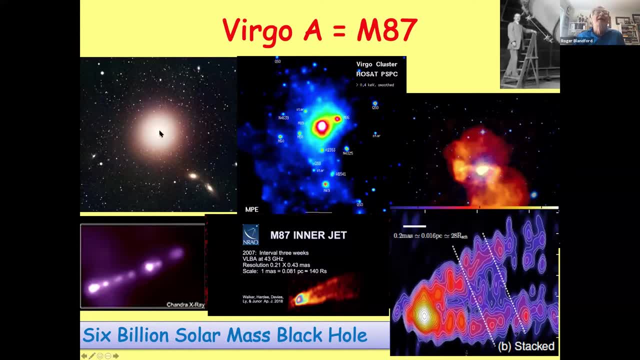 being kept hot by the, by the, what comes through this jet here in the from in M87.. So if we look on at x-rays imaging on the small scale, we can make an image of this jet with features in it. Again, if we look. 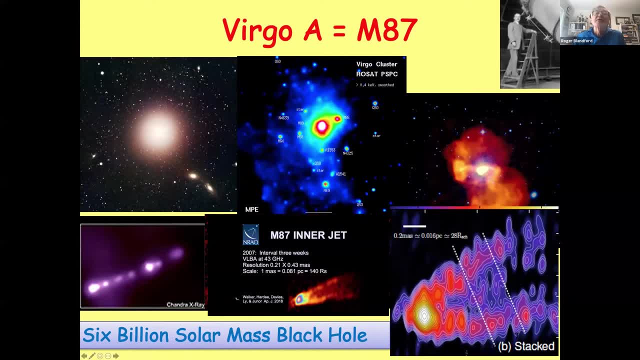 with radio imaging. I don't know whether I can, whether this will work or not. May do, Okay. Oh, this is. this is time-lapse photography done using by radio astronomers And you can see, if you like, the outflow along the jet. And then here is looking on a smaller scale And again you see. 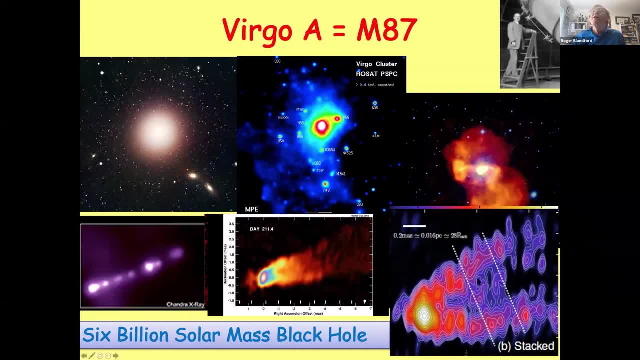 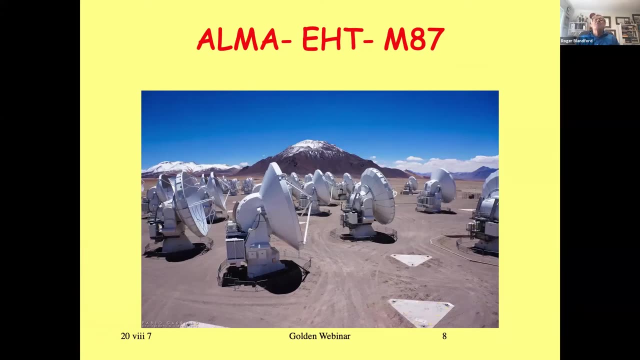 this edge brightening or interaction with the boundary layer Here. So again, this is M87.. Now M87,, of course, is very famous now because it was the source that was observed using the Event Horizon Telescope to show the famous black hole shadow. And let me just 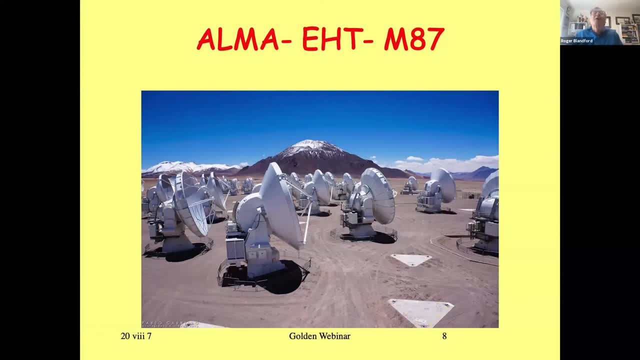 say, as I'm sure everyone on this call is very keenly aware, that the Event Horizon Telescope is anchored by ALMA. ALMA has been a glorious telescope. It's a huge international endeavor involving very actively South Americans, particularly Chileans, And it is certainly far outperformed by very high expectations from the 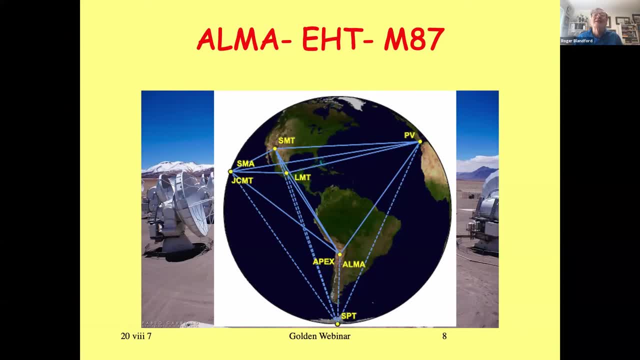 start of it And, to be blunt here, it is in the EHT here And it is. I just learned about a new discovery it made this morning And it's been a wonderful instrument. So if you know anybody who worked on building this telescope, 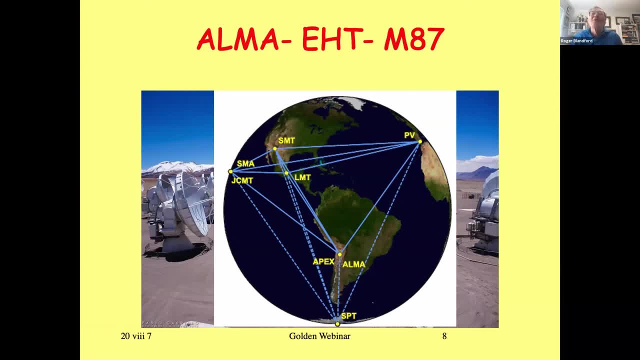 please express the thanks of so many astronomers for all the wonderful things it is continuing to discover. This is the Event Horizon Telescope. These are the combinations of telescopes that were used in the initial observations, going from Antarctica and different continents and so on, And that gives us the fine image. 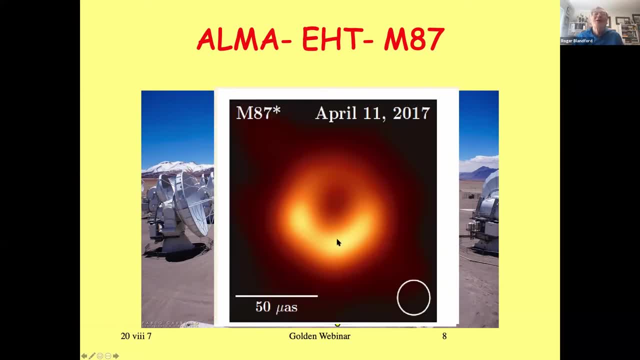 And this is the one that's been famous and in all the newspapers and so on, And what is believed to see here is essentially the shadow of the black hole in there. The actual size of the black hole is a little bit smaller than this. 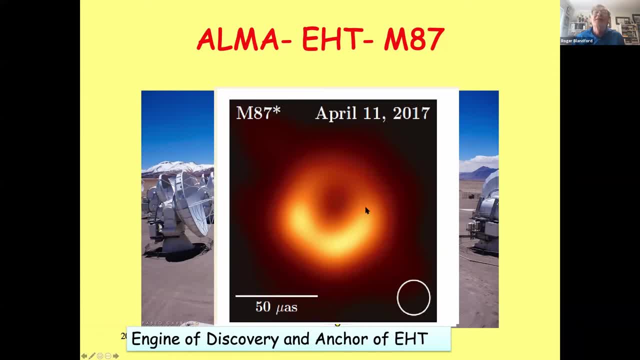 but because of the bending of light you get a large shadow And then there's this bright ring of emission here around it, And this is the best evidence of all that it's black holes that are fueling these, these jets and these giant double radio sources. 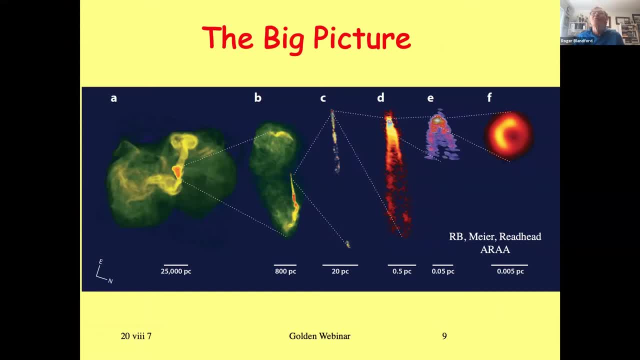 So if we look at this in the big picture point of view, so here's M87 and here's the black hole shadow And we get to larger and larger scales And if we actually go larger than the scale of the X-ray emission in the cluster of galaxies, 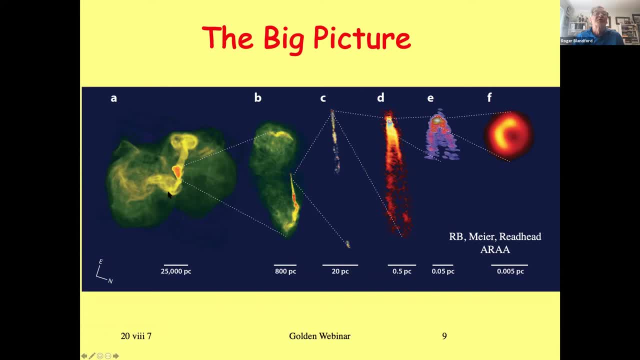 then what you're seeing is this tiny black hole in the nucleus of the galaxy. no big deal. It's bigger than the solar system in its physical size, is influencing its surroundings on scales up to 10 billion times larger than some of the sources. 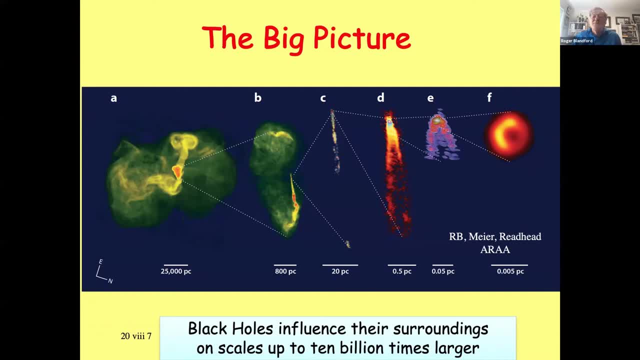 In this source. it's only about a billion times larger. It's influencing its surroundings. So this tiny, tiny structure in the middle, which I'm going to call a black hole, is influencing all that's going on around it. It has an enormous environmental influence. 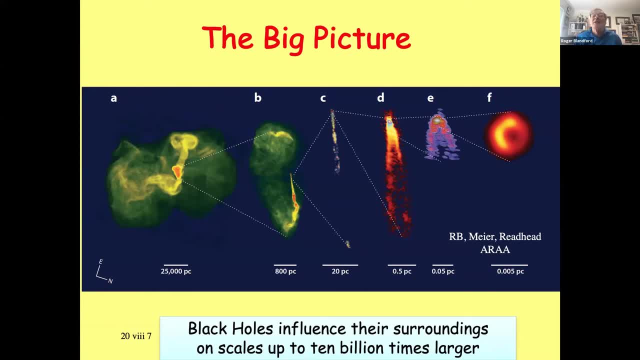 and is a major part of the story of galaxy formation, These, These very active galactic nuclei, these active black holes in the centers of these galaxies. Let's move on. Let's talk next about another important source. The last one I said was 3C274 was one of its names. 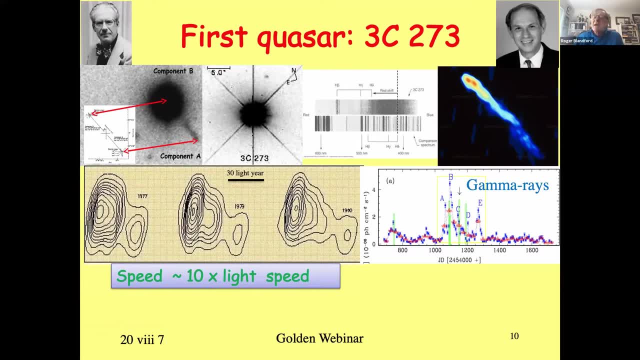 This one is the first quasar that was discovered, and it's 3C273. And it was identified as such by teamwork, essentially bringing in this multi-wavelength idea. Here's Martin Schmidt, who took the position created by Cyril, a radioastronomist working in Australia, Cyril Hazard. 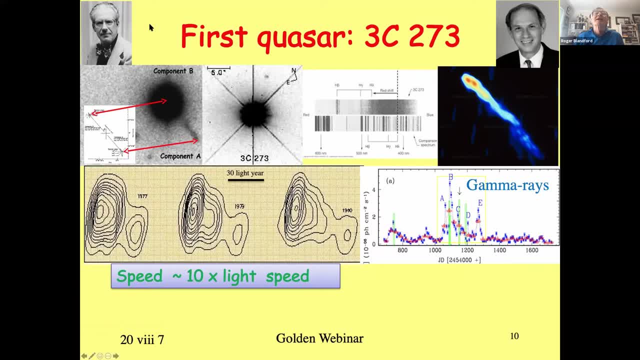 took that position, found the source and then realized it was a cosmologically distant source And therefore, what was being observed was it prodigiously luminous, several hundred times the luminosity of the associated galaxy, And this was the very first quasar. 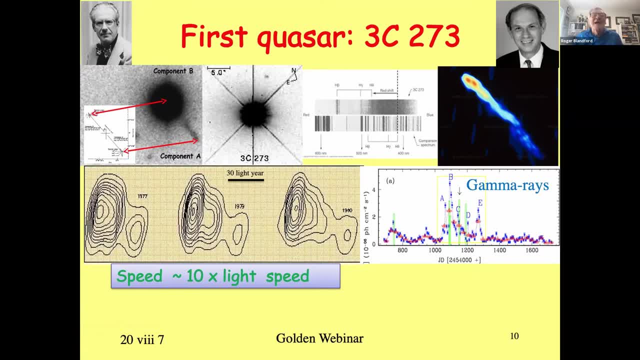 And this is, if you like, one of the powerful types of active galactic nucleus. Many of these quasars have powerful radio sources, and this is no exception. Here's the jets shown here at optical wavelengths, but we also see it on the small scale using BLBI. 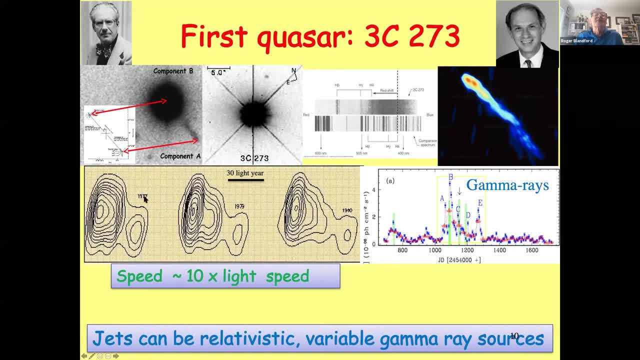 And this is the jet observed in the 1970s. We, of course, know a lot more about it than them, but this is a lovely historical demonstration that inside this jet seen at radio wavelengths, there is radio emission. Here is the, if you like, the stationary part. 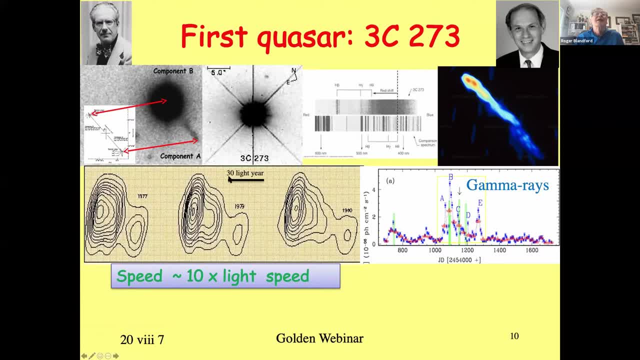 And then this feature here you can see is moving outwards. And if you say that size is 30 light years and you know the time, then you can quickly infer from this piece of paper that the feature here is moving 10 times faster than the speed of light. 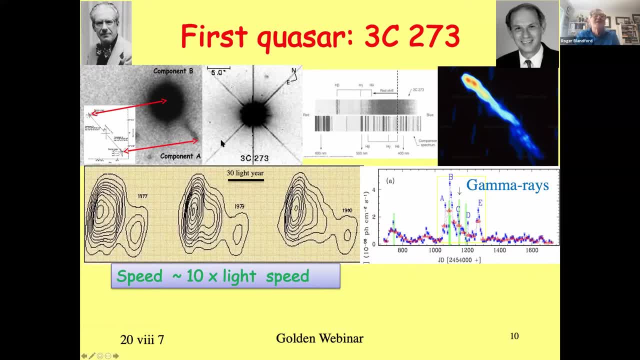 And this is not a violation of Albert Einstein's special relativity. It's really a consequence of simple kinematics. what happens is that this feature is coming almost towards us at nearly the speed of light, And if we work out the math, then it appears to cross the sky faster than the speed of light. 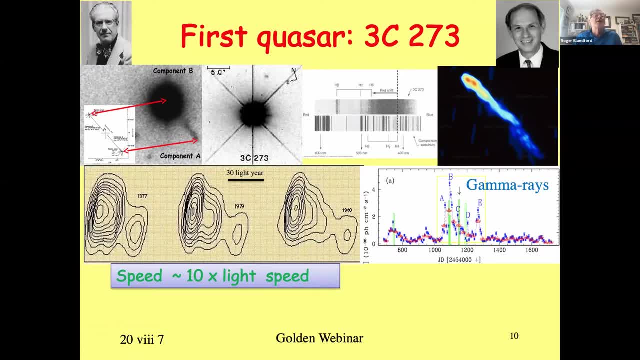 And, furthermore, is very much brighter than if we were looking at it from the side, And this is just a simple consequence of special relativity, not a negation of it, And that means that we are likely to see preferentially those sources that are pointed in our direction. 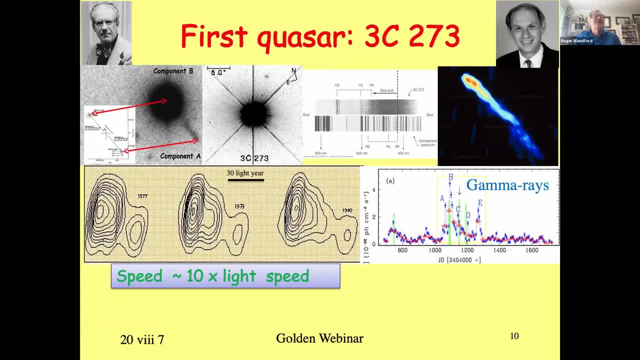 There is no need for paranoia Here. it really is a physical effect. Those sources where the jets are pointed towards us and have material that is flowing outwards at the speed of light are preferentially bright, and therefore they're the ones that the astronomers are going to fixate on. 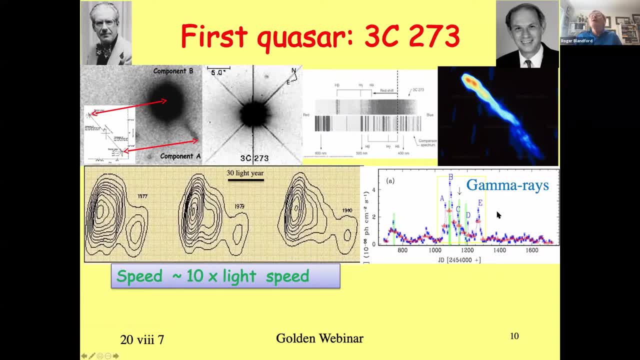 Here's the spectrum from 27A, And one thing I will point out is that this is also a powerful gamma-ray source, And many of these sources, with these jets that are pointed towards us, many of these sources are also powerful gamma-ray sources. 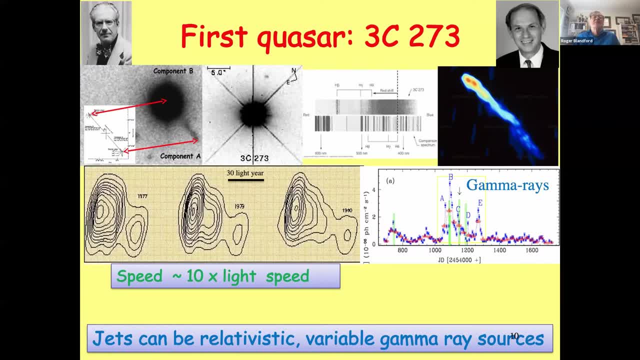 And I'll come back to that point a little bit later. So just to drive home the point, the jets, the outflows, if you like, are relativistic, more circumstantial evidence that there's some relativity involved in the source of these jets. 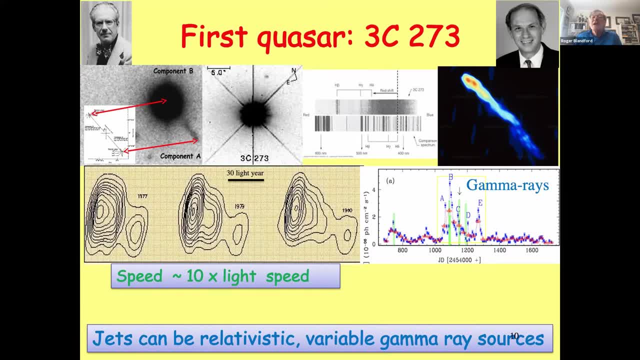 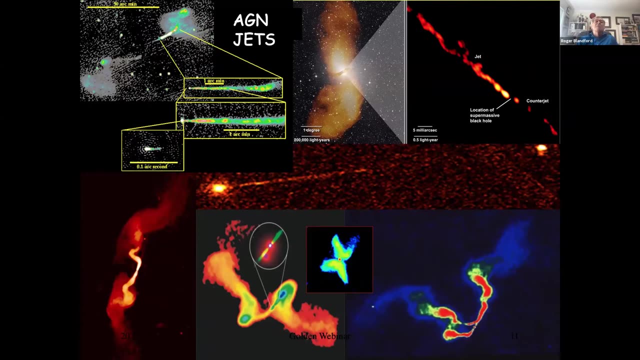 And what better relativity can we have than the black hole? And they're also, in practice, rapidly variable gamma-ray sources. Again, I'll return to that point a little bit Now. there are many, many jets out there. Here's just a few, you know, of thousands and thousands of them that have been imaged. 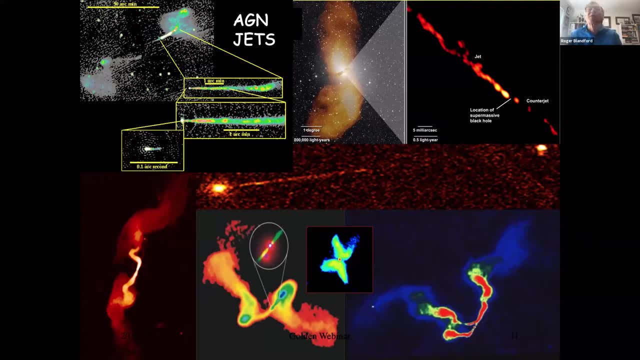 I'm not going to go through all of these, but be rest assured that every one of these sources has a mother who loves it, And here's one that was mapped was an early one in the history. This is actually a more modern map. 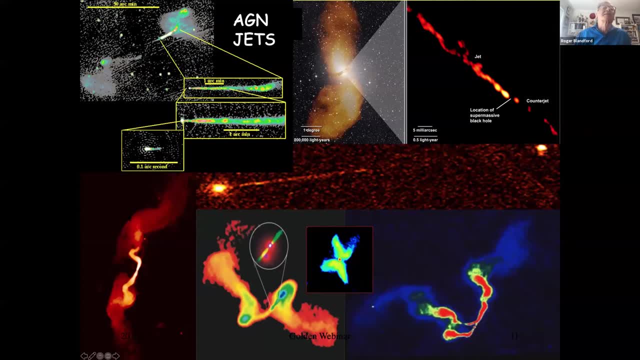 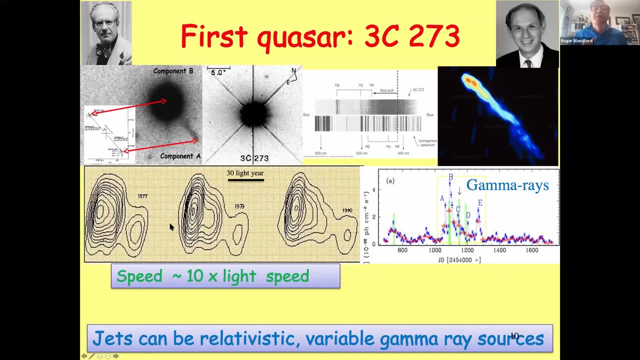 and it was actually made by my colleague, Tony Reedhead, who is no stranger to Chile, having worked with CBI-MAC with background telescope near San Pedro, And he was also responsible for this image here in his team, which showed this so-called superluminal expansion. 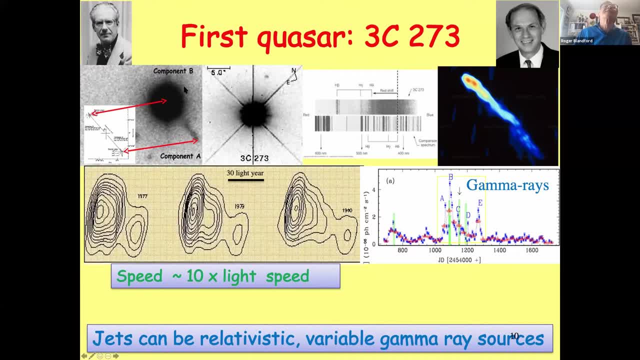 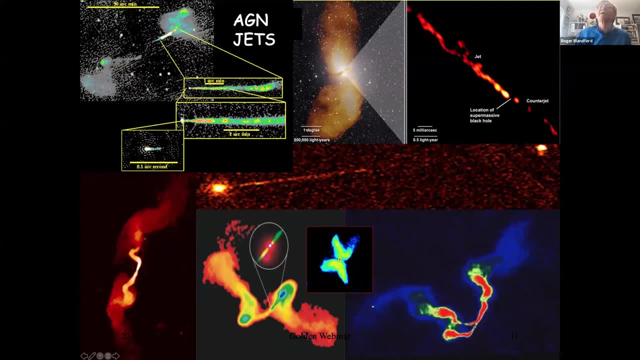 So this is a very nice one, And we can see again. these jets are remarkably straight. Here's another one of the X-ray wavelengths You can pick to array. See, You can see this dead straight structure and it's created by a black hole in there. 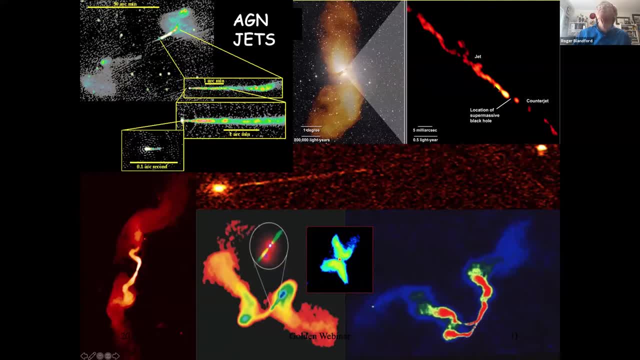 And then there's a sort of beam dump at the end. Here's a local galaxy that you know well in the southern hemisphere, Centaurus A. Here are other ones, And they aren't just the province of quasars or active galactic nuclei. 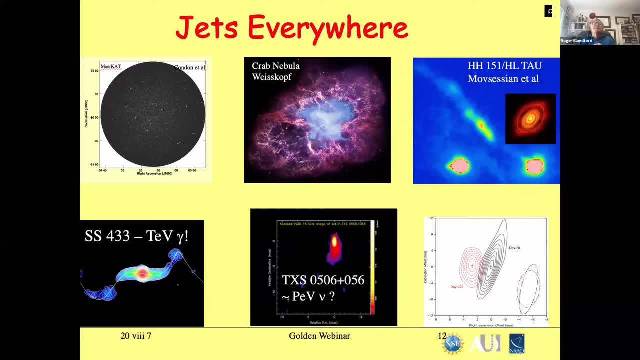 the nuclei of galaxies. We see jets all over the place. We see them in supernova remnants. Here we are. Here's the famous Crab Nebula And you can see two jets in there. Here's a protostellar, famous protostellar source. 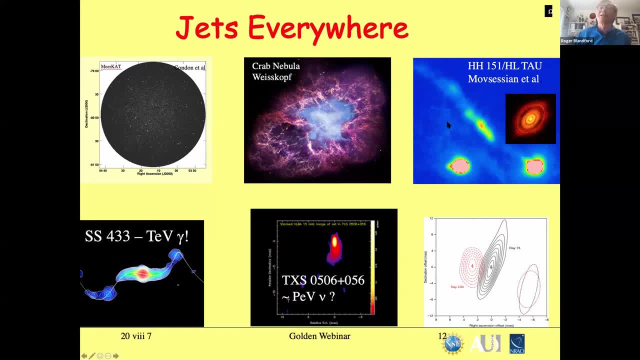 imaged by ALMA here, one of the most famous images from ALMA: HL Tau, That's got jets. Here's SS433, almost certainly a black hole binary. Here's a famous neutrino source that's been in the news a lot lately. 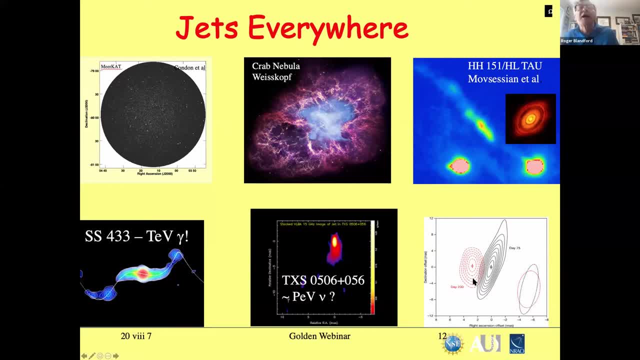 And here's the gravitational wave neutron star binary GW1708-17.. Again, that has a jet. And here's the South African telescope. Meerkat has done a very deep field And we can say that of the sort of AGN type of jets. 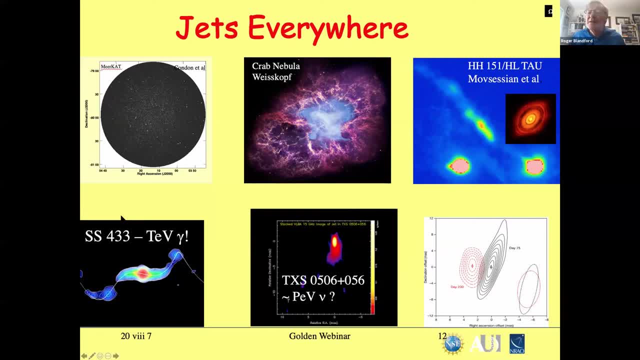 there's probably a billion of them on the sky that we can see already. I'm not going to name them all, but they're out there. They're extremely common. The jet business is very, very. it's a common cosmic process. 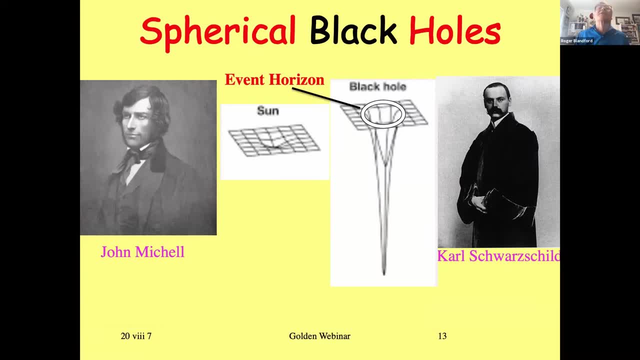 It's not just some idiosyncratic strange behavior. So let me segue out of the observational astronomy for a moment and go back to and go to physics now. And the idea of a black hole has many, many sort of precedents in some sense. 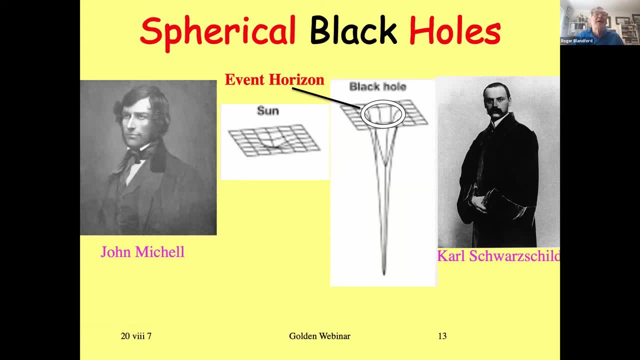 But one of the most famous was actually a professor of geology became eventually- was John Mitchell, who thought about many important impressions. He thought about many of the most recent ideas And he wondered about a star that was so concentrated that light could not escape from its surface. 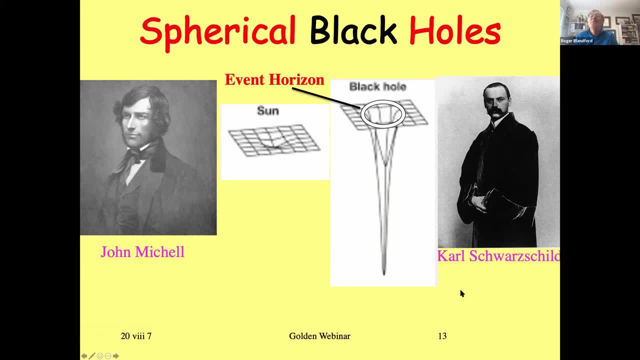 This was actually unknowingly put into a formal framework by Karl Schwarzschild, who at the time was a soldier in the First World War, And he took the newly minted Einstein field equation of relativity and was able to solve them and show that there was actually a spherically symmetric solution. 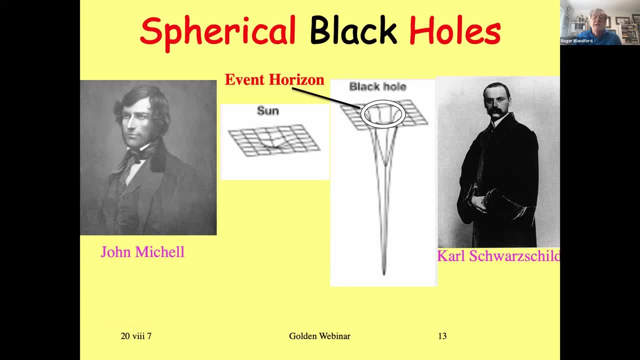 And if we do what he in practice did not do- and he passed away sadly soon after doing this- but if we take that argument a stage further, you can discover an event horizon that's described by this famous solution, And so, with a little bit of historical license, 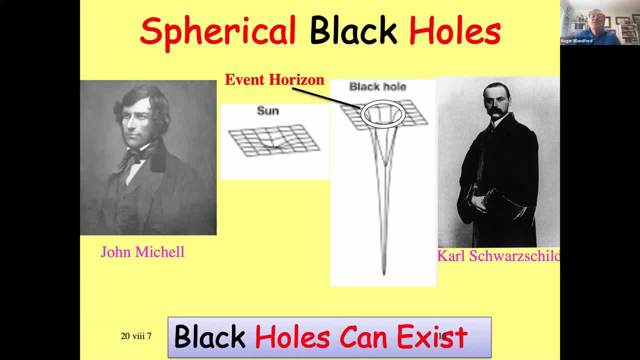 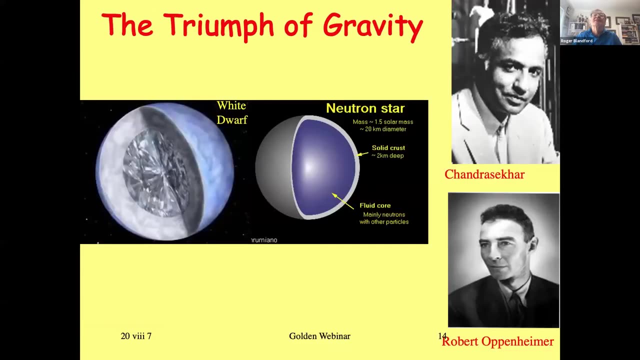 we can say that these gentlemen likely showed us the black holes in the ideas of a theoretical physicist. They can exist. If we go on a little bit more historically then several people, but notably Chandrasekhar and Robert Oppenheimer, thought about the properties of white dwarf stars and neutron stars. 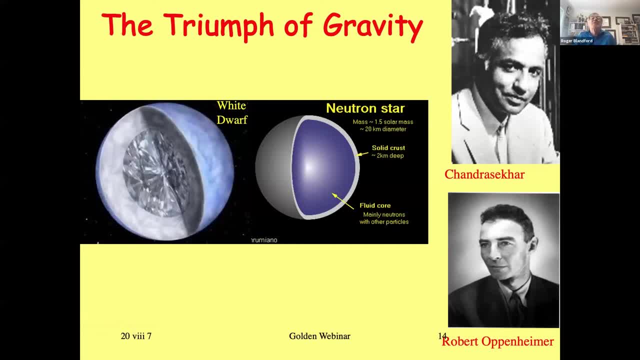 which are the other two types of compact object, And they showed something rather important, which was that there was a maximum mass to these objects And, as astronomical stars were going to leave behind remnants that were more massive than these maximum masses, there was really no alternative to them continuing to collapse. 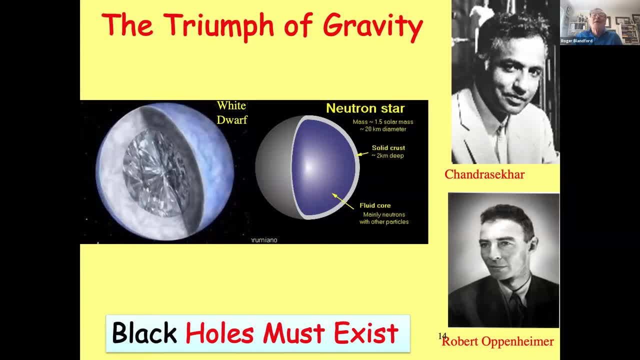 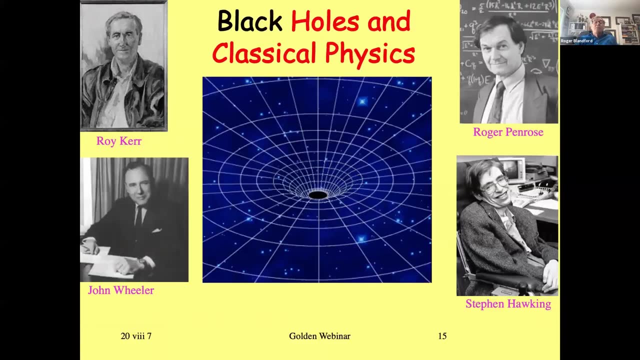 and form a black hole. And those black holes, therefore, not only can exist, they must exist according to what we see going around us in the universe and stars and so on. So that was again a great step forward. Now the mathematical and physical development of black holes. 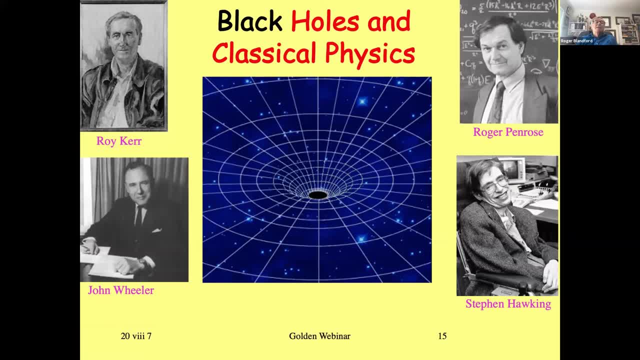 was prosecuted by many people in a rapid time of discovery in the 60s and early 70s. Here's Roy Kerr, a New Zealander, who discovered how to generalize the spatial black hole, And here's the so-called metric. 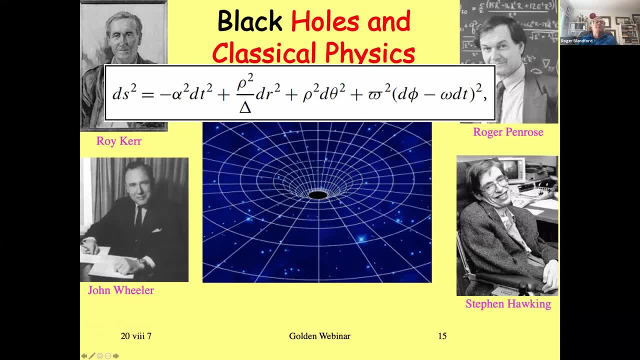 which describes the geometry of a black hole that is spinning. I'm not going to interpret this equation, just say that it's not that long And it was amazing. It was a great mathematics discovery to find this. Here's John Wheeler, who 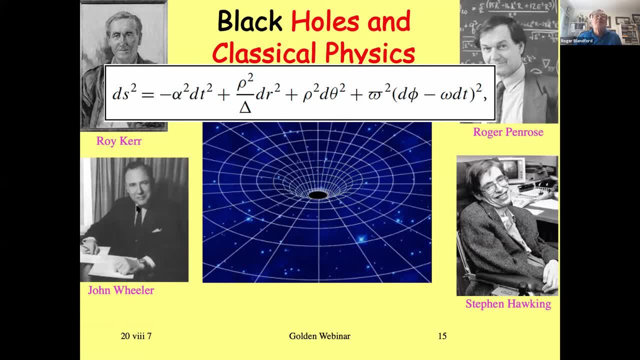 and with a team of people thought a lot about their physical properties and the challenges they presented. Here's Roger Penrose, And I'll give one of his many contributions in a short moment. And here's somebody else who needs no introduction: Stephen Hawking. 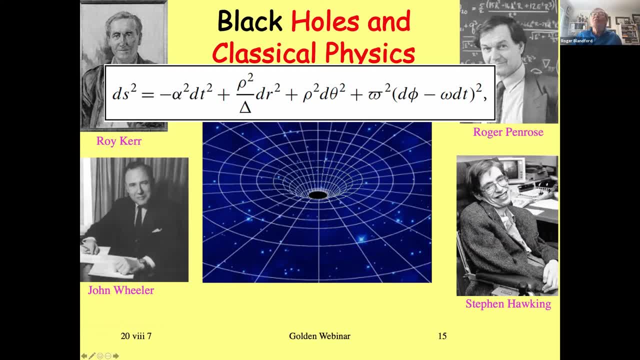 who again did research on the classical aspects of black holes as we see here, but also took this and put forward into a quantum regime, which will not be part of my story today. So associated with this black hole is an angular frequency, So there's a spinning black hole. 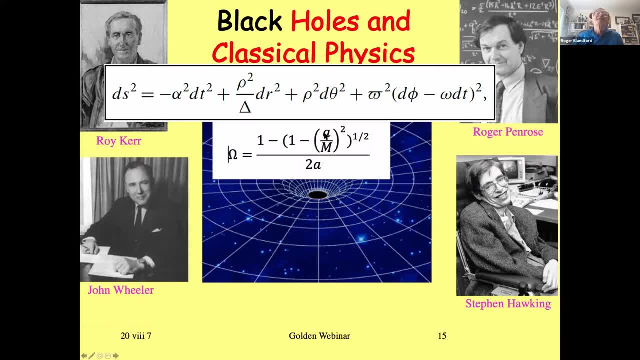 It's just not just fairly symmetric, it's actually spinning, And it has a parameter that describes it, called A. The only thing you need to know for this talk is that I can get an angular frequency, a rate of rotation, a rotation period with this black hole. 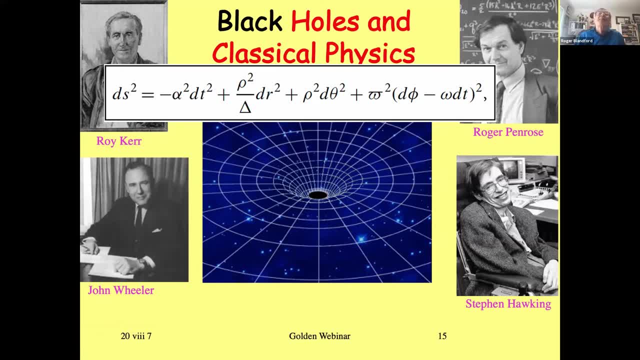 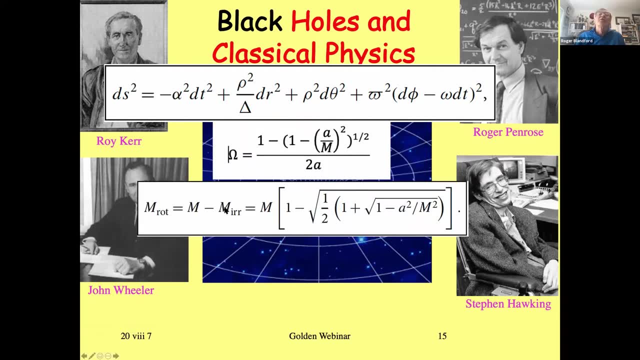 despite the fact that it has no fiducial mass, There's only a fraction of the mass of the black hole that's associated with it. And one other thing- and this is what Roger Penrose and the others understood- was that in the mass or the energy associated with the black hole, 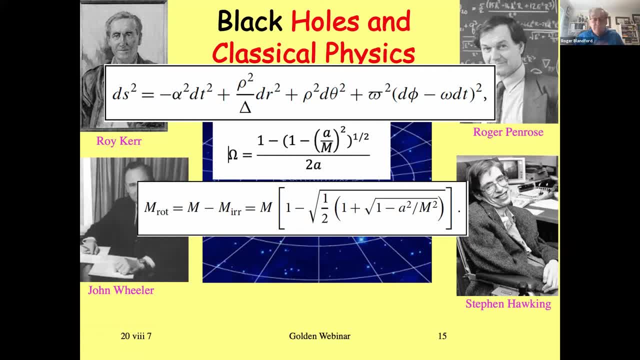 there's a part of it that's associated with rotation, And that part that's associated with rotation can be as much as 30% of the energy associated with the mass of the black hole, And it is, in principle, by thought experiments extractable. 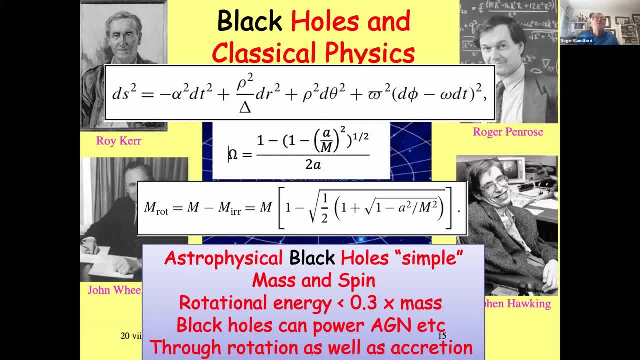 And what I mention here is that some fraction of it, perhaps a third or a half of it, is in practice extracted by a magnetic field in these sources. So just to summarize this, slide black holes. they're extraordinarily simple in the classical level. 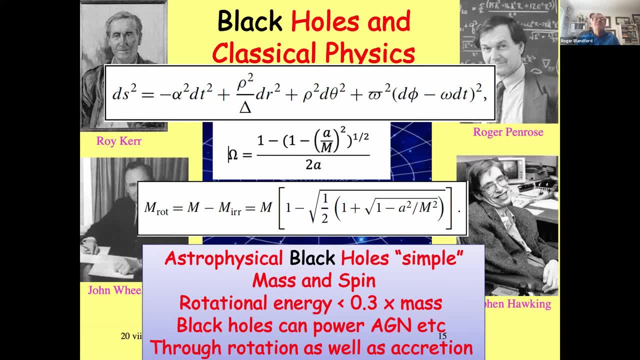 They have mass and spin, They have spin energy And there's enough energy there in one of these black holes in the galactic nucleus to power the activity in the galaxy and in the region around it as I described, And it can do this over the age of the universe. 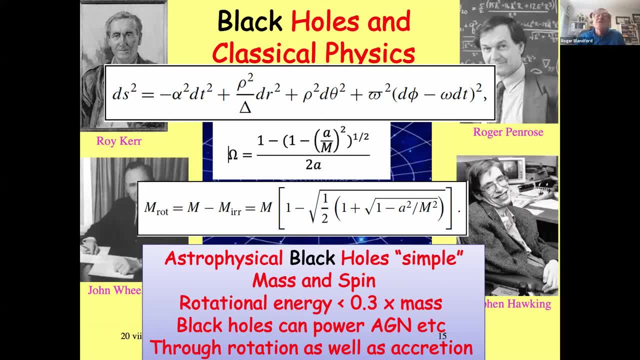 And it does it by two channels. basically, One of them is rotation, which is what I'm going to emphasize here, And the other is having gas that accretes, that falls onto it and liberates its binding energy, just like if you drop an apple on the floor. 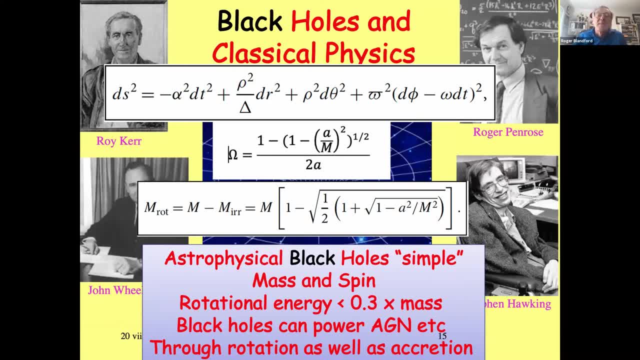 that apple will lose its kinetic energy and it'll be converted to get a little bit hotter and converted into heat and so on. So that is a very important part of black holes. Let me just introduce one other physical idea here. I think it's relatively well known. 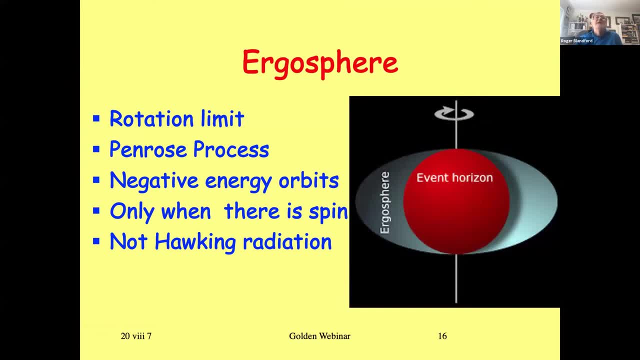 but I'll just repeat it here- is that there's a maximum rate at which black holes can spin. But if you try and perform some thought experiment, with one of your trusted colleagues being sent in a spaceship around the black hole and just hovering outside the event. 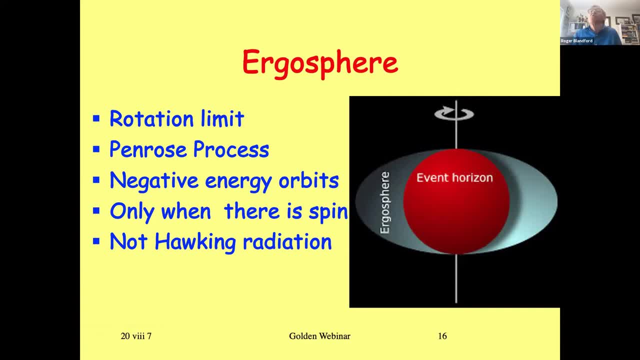 then that spaceship must orbit. it essentially is at the angular frequency of the black hole. It can't be at rest with respect to the distant stars, And the region within which it has to spin is called the ergosphere, And what Penrose showed 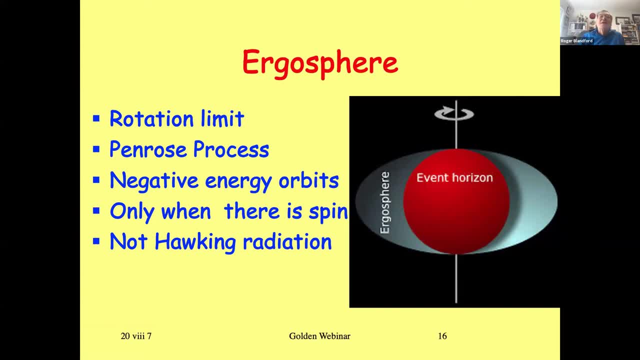 I'm going to go in a very clever idea- was inside this ergosphere, this region, here there exist orbits which have negative total energy. They don't exist outside the ergosphere, but within the ergosphere they do, And so what that meant is: 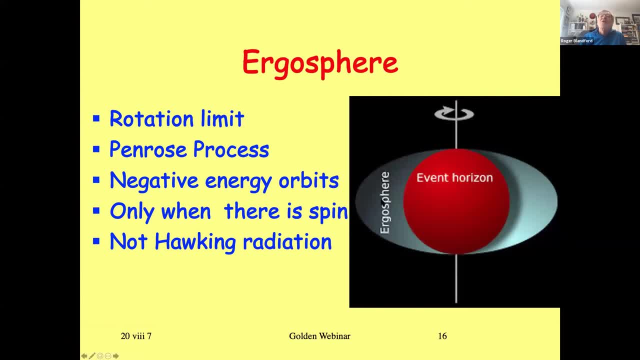 if you did a bit of engineering outside the event horizon and put a rock onto an orbit with negative total energy and let it go into the black hole, then it would actually remove some of this rotational energy. And that was as a thought experiment. 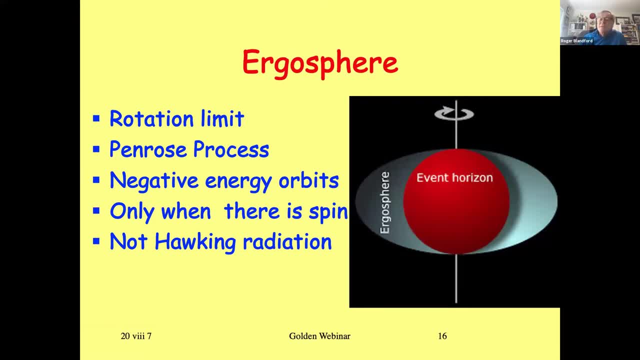 was a way of getting spin energy out of the black hole, And so that's the key point is that, in principle, it's possible to extract energy from a spinning black hole, And my contention is that's responsible for a lot of what we're looking at. 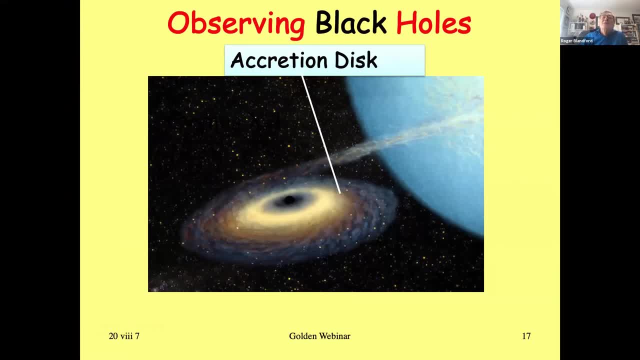 Going back to the observations, I'm not going to describe this in much detail, but in the early 1970s people started to find evidence for black holes that were more massive than the maximum masses allowed by Chandrasekhar and Oppenheimer. 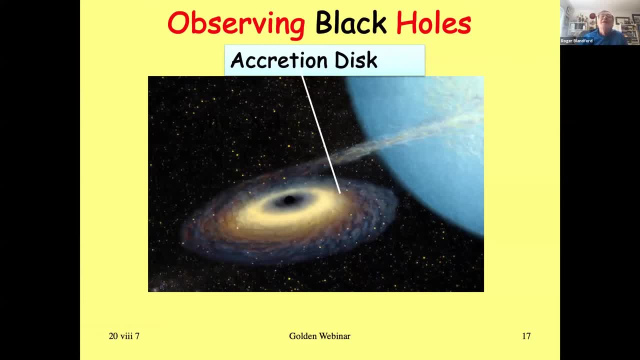 for white dwarfs and neutron stars respectively, And they had all the properties of black holes And, furthermore, it looked like they had disks around them, that disks of gas, like Saturn's rings that were able to glow, particularly at X-ray wavelengths. 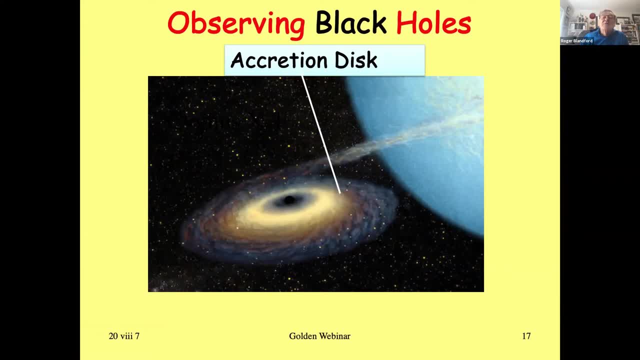 and then you were seeing the emission liberated by accretion rather than rotation, So you were seeing the accretion mode, if you like. And although people had thought about AGN as being black holes from the days of discovery, they didn't really know that black holes were actually quasars. 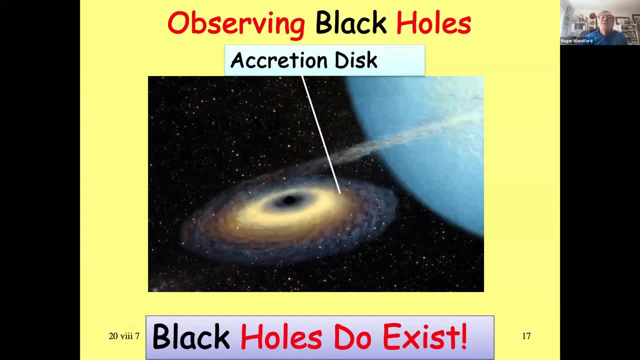 This was probably the time when almost everyone accepted that black holes really do exist, despite the disquietude that some physicists had with this proposition. Our galaxy itself. it doesn't have an active galactic nucleus, and we should be grateful for that. 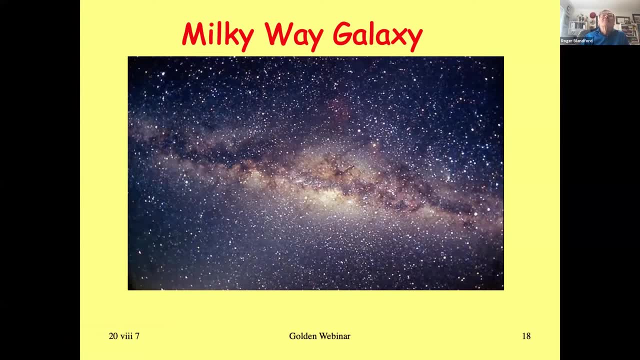 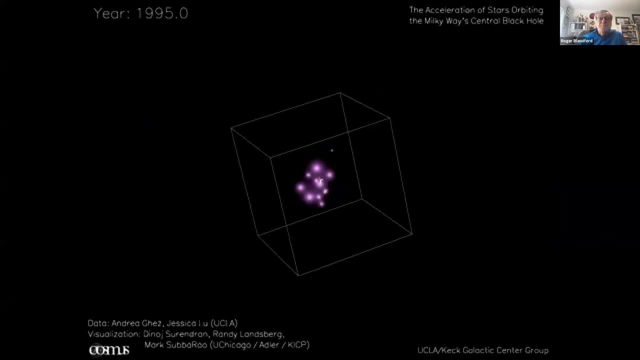 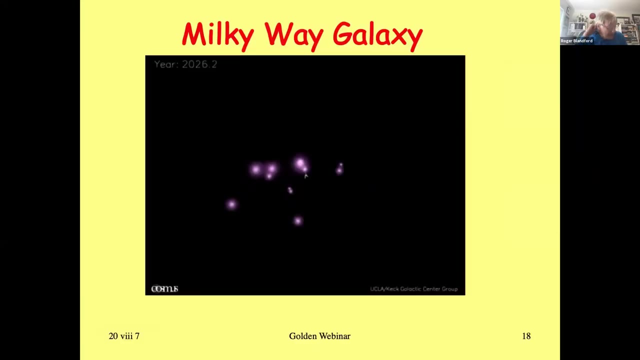 We wouldn't want to live next to a quasar, But here's the center of our galaxy. See in red here it's seen in X-rays. Here are stars observed at infrared wavelengths, shown in orbit around a central mass, And you can see just like the planets in our solar system. 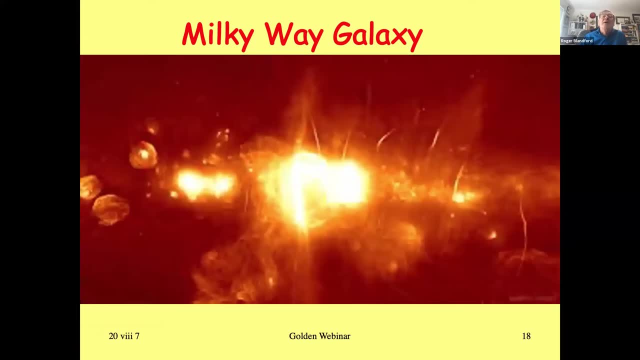 they orbit a central mass and that mass is four million solar masses. It's a relatively modest mass compared with the mass that's associated with M87, which is six solar masses, And this is a nice image shown by the South African telescope. 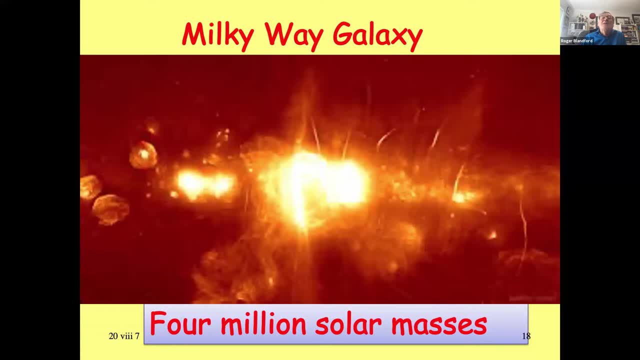 I just mentioned Meerkat and this shows on the large scale what's happening in the center of our galaxy at radio wavelengths And we see all these mysterious filaments and so on which are almost certainly magnetic structure and supernova remnants and so on. 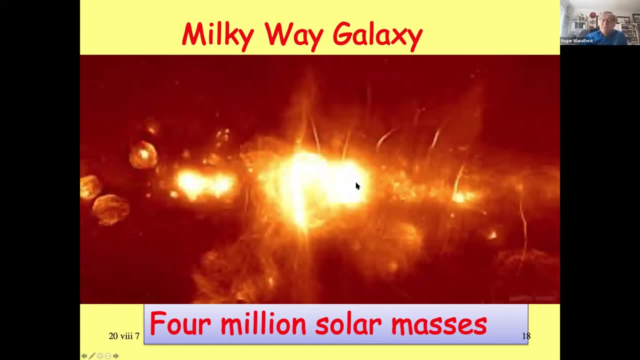 So we're learning a lot about the geography of our galactic nucleus using these new radio telescopes. So we have a black hole. we've measured its mass in our galaxy- a small one and a large one in M87.. And, of course, there are many more that we know about. 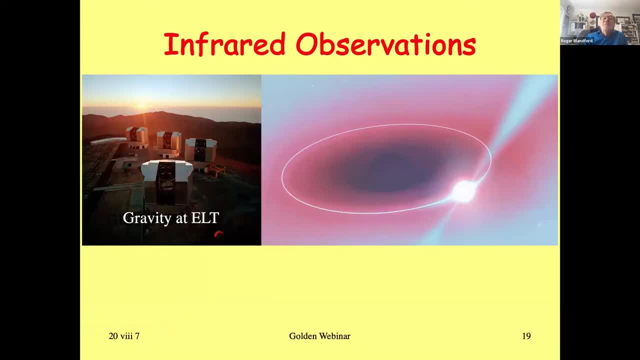 Here's another observation of the black hole and its environment in our galaxy, made with the gravity instrument at the ELT in Paranal, And this again has been a wonderfully successful program, And there you can see magnetized clouds that are in orbit. 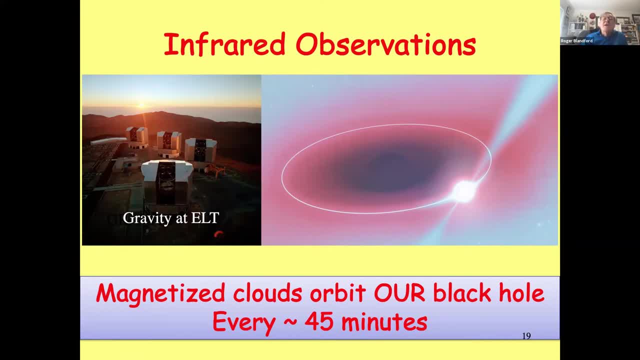 around this black hole at the center of our galaxy, And they're orbiting about every 45 minutes. We're learning a lot by these observations. These new infrared capabilities are extraordinary, And this is interferometry at infrared wavelengths rather than at radio wavelengths. 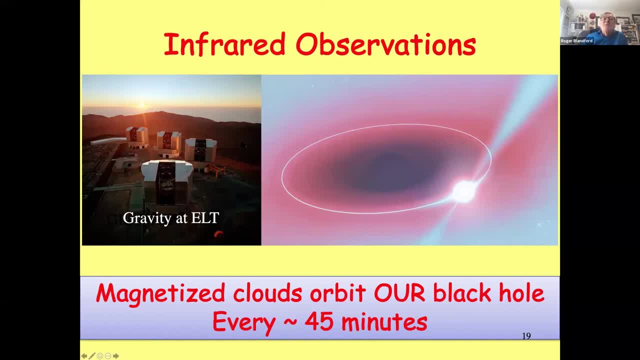 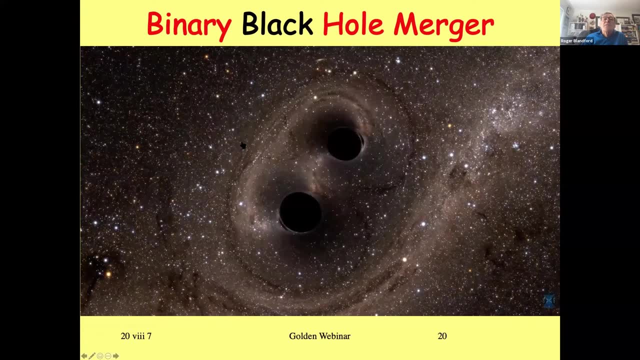 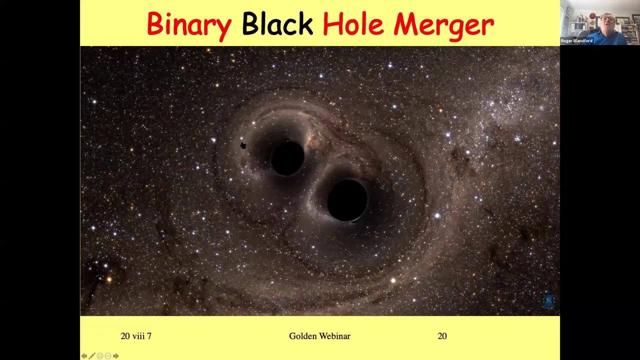 which is what we've just discussed. Black holes, of course, have been very famous recently because of the gravitational wave observations using LIGO, VIRGO and soon to be other telescopes as well, being part of the act. Here's a simulation. I emphasize: 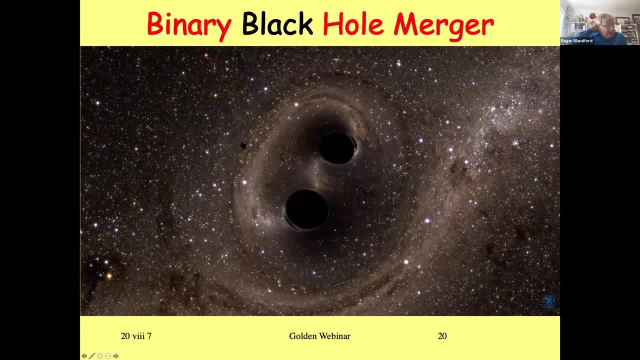 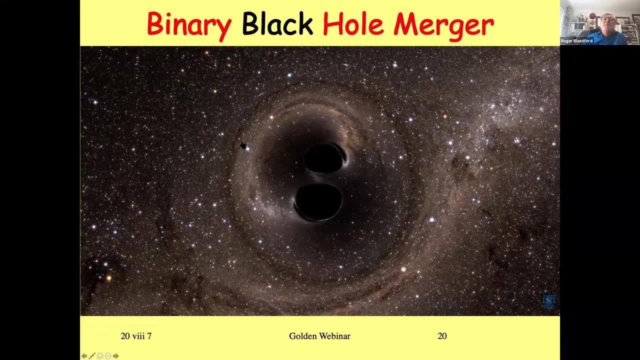 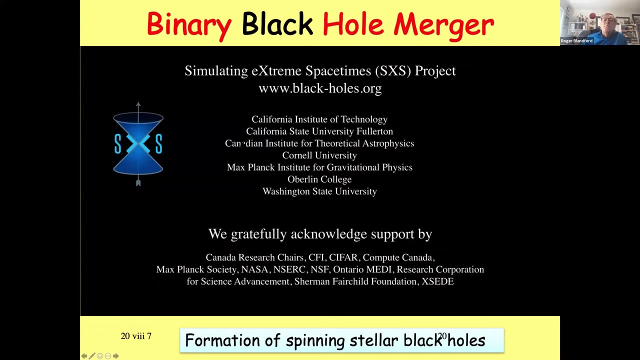 of the first merging black hole discovered in 2015.. And you can see the final merger happening there. And so there we have a process that was observed using gravitational waves that was able to form a spinning black hole, albeit on the stellar scale. 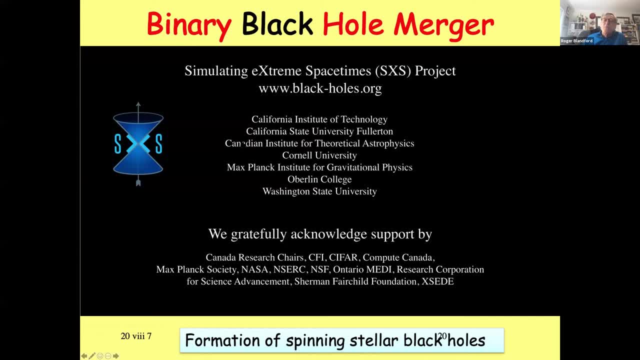 And although I won't discuss this anymore, corresponding processes are strongly believed to be happening on the scale of an active galactic nucleus And they're binary black holes with masses of millions to billions of solar masses, Occasionally merged by essentially similar processes, and are observable. 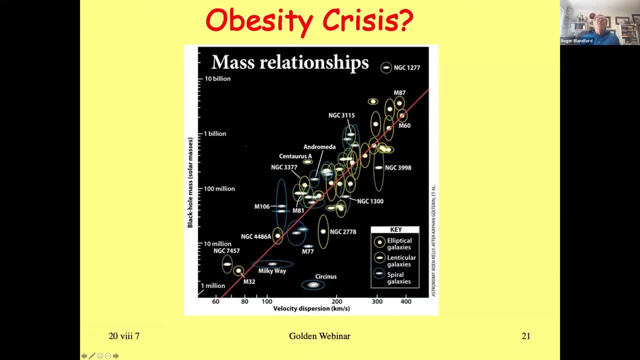 although that hasn't actually happened as yet. Moving on, as I emphasized, there's a range of masses involved. Here's a compilation of the measurements of the masses, And they range, as I said, from about a million or so solar masses. 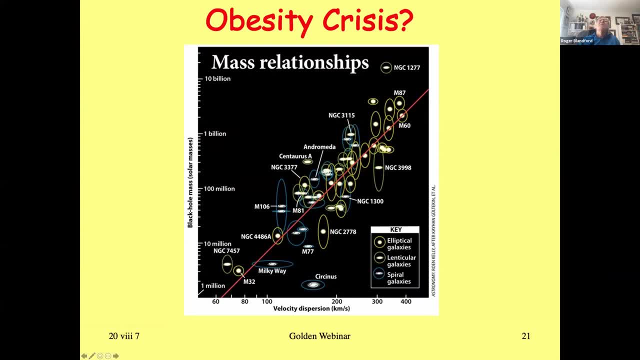 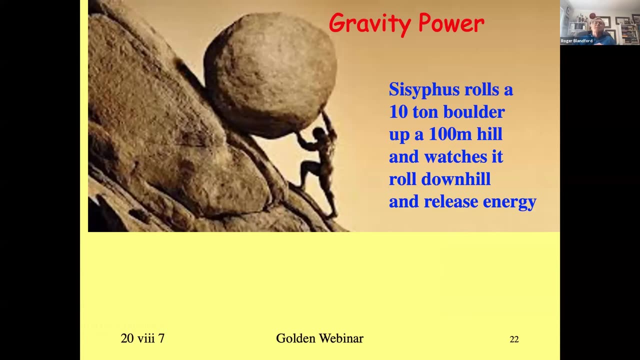 The Milky Way, our galaxy. there's 87. And the champion in the Guinness Book of World Records is up there at about 20 billion solar masses. Okay, so these are big beasts. now Let's talk a little bit about the physics now. 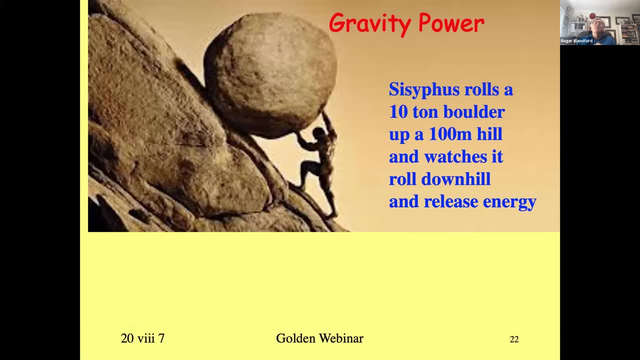 And I want to go back to this business about gravity power. So if we go back to the accretion mode and imagine a well-known character from Greek mythology, Sisyphus, rolling a 10-ton boulder up a 100-meter hill, 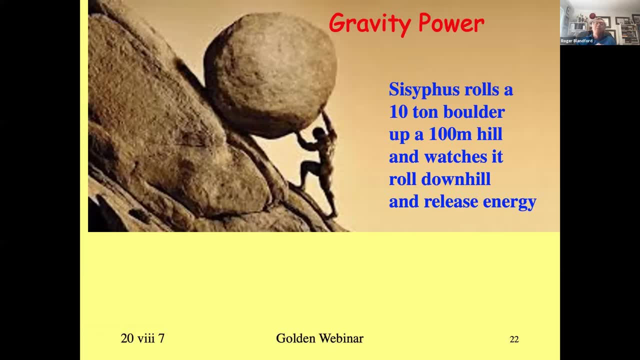 and then watching it roll down downhill. that was his lot in life. it would release energy, And the energy that it would release would be the same sort of energy you get from a much smaller amount of chemical energy with three kilograms of TNT or 300 grams of gasoline, alcohol or candy. 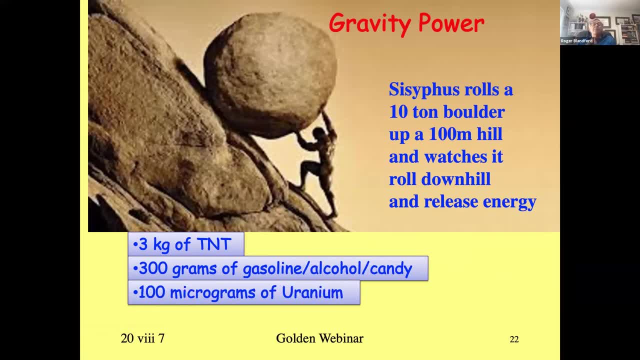 choose your poison: or 100 micrograms of uranium or 300 nanograms of gas accreting onto a black hole. So the point about this slide is that the accreting gas in these accretion disks orbiting the black hole. 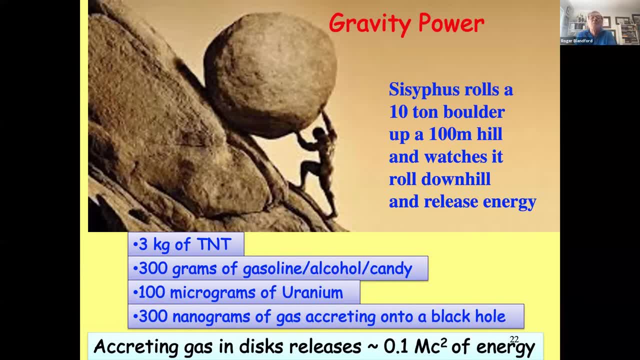 can release an enormous amount of energy for a small amount of gas. It's extraordinarily efficient, much more efficient than nuclear power. nor does the magnitude more efficient power or mechanical power as we see up here. So poor Sisyphus, So roughly, you can expect. 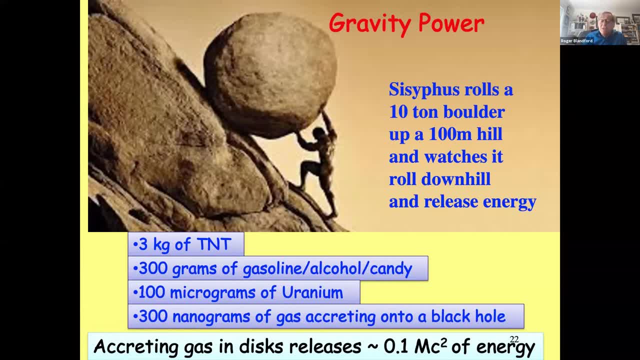 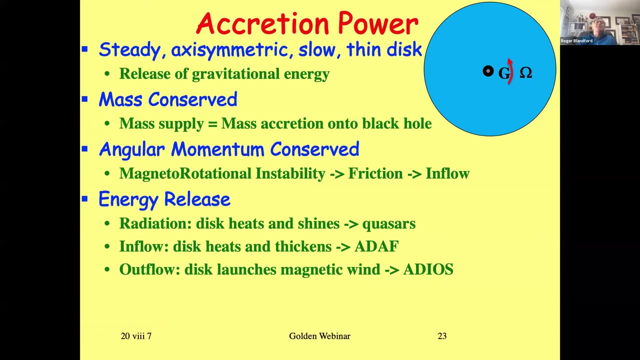 typically about 10% of the rest mass energy of the accreting gas being released in some radiant form, one form or another. And so let's talk a little bit more about this accretion pair And if we make the very simplest type of 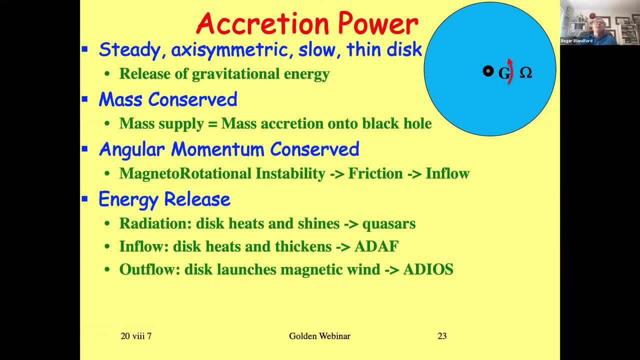 idealized description of this. we can imagine a disk of gas, make it flat and steady, have gas spiraling inwards under friction. it's a bit like Saturn's rings, if you like, but with friction between adjacent rings, and that friction is caused by a process. 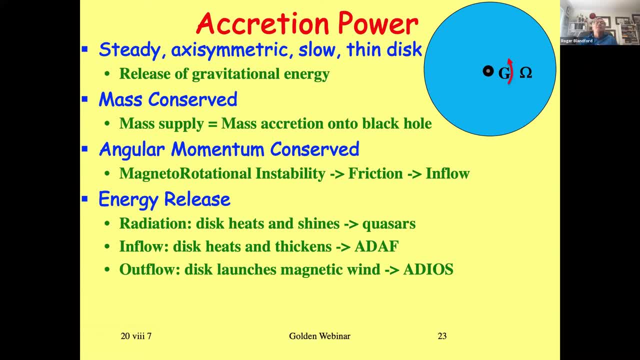 that we now think we understand It's magnetic fields that go unstable. they provide this friction and that friction causes the gas to move inwards And if we make the very simplest model, the mass will be conserved and what you supply up out here at large radius. 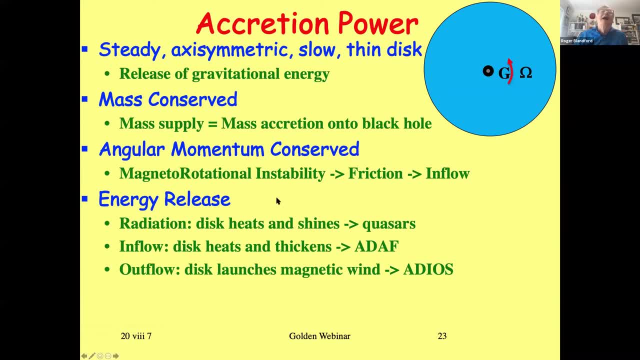 will go into the black hole at small radius, And not only will the mass be conserved, the angular momentum will be conserved. Angular momentum is a physical property, it's a sort of momentum of rotation, and that should be conserved. 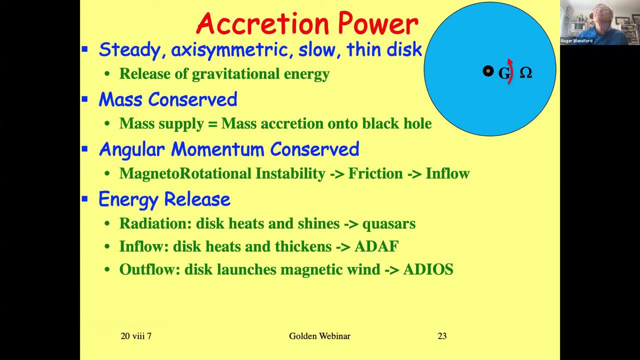 and indeed we think it is here- and the friction balances the inflow of the gas and you don't lose any angular momentum in this simple description And the consequence of this is that there's an energy release, there's a lot of energy released. 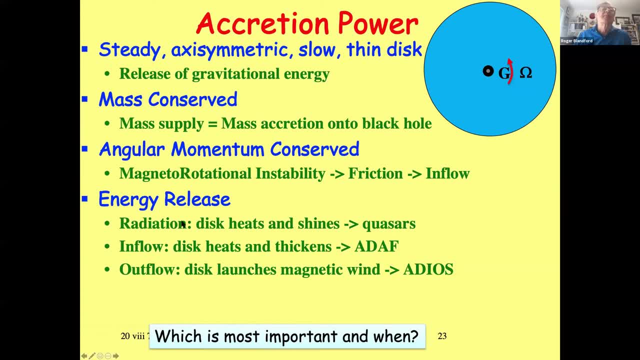 and there are three ways in which we think that energy might be released. The first is it will heat the gas in this disk and, because it's got hot, it will be able to radiate and shine, and that will be, for example, what goes on in quasars. 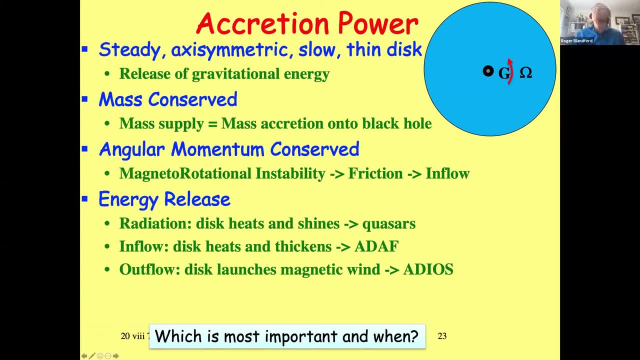 where we get lots of bright ultraviolet radiation, and we believe that comes from the frictional heating of the gas in the thin accretion disk like this. Another option that happens in different types of source is that the gas heats but it isn't able to radiate. 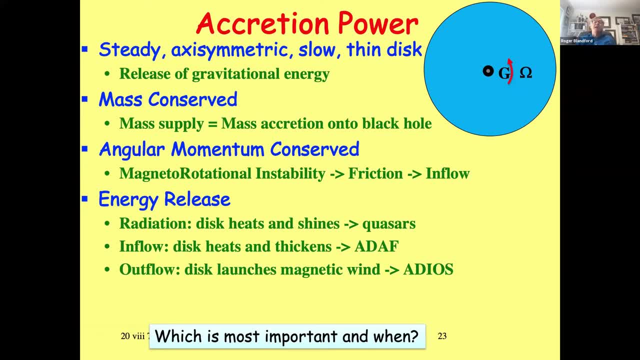 and that means that because there's a lot of pressure there now, the disk will thicken, and this is sometimes called an advection-dominated accretion flow, and so we'll see an example of this in a moment. but there needs to be a very thick accretion disk there. 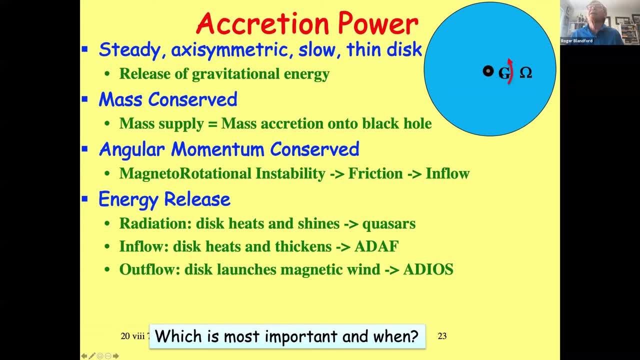 and basically, the gas is still more or less conservative, but it isn't able to radiate. but what is supplied goes eventually down the black hole, crossing the event horizon. And then the third possibility, which is the one I shall advertise more here. 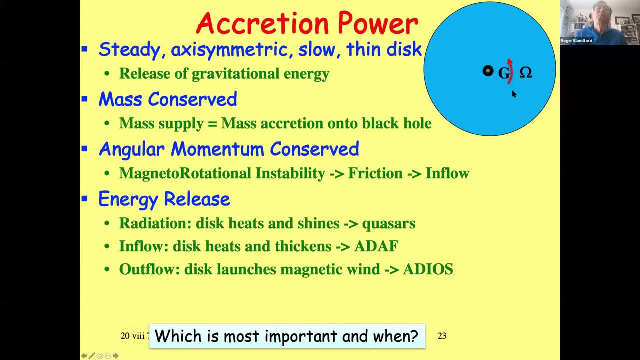 is the possibility that the energy is released, essentially all in the form of an outflow, and this disk launches a wind using magnetic field, and that is what my colleague Mitch Beigelman and I once called an advection-dominated inflow-outflow solution. 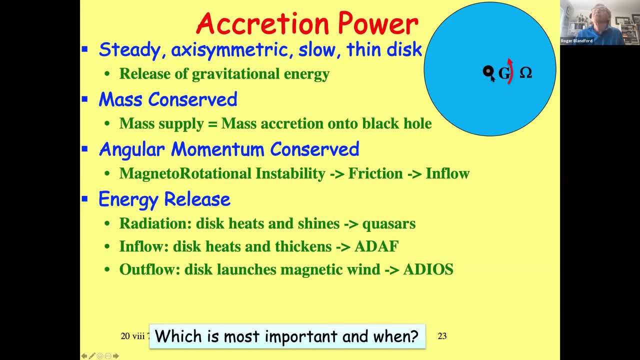 and this is an outflow that's driven by the energy that ultimately comes from the inner parts of the accretion disk, And so the question is trying to understand which of these modes of energy release is important and where they are Moving onwards. 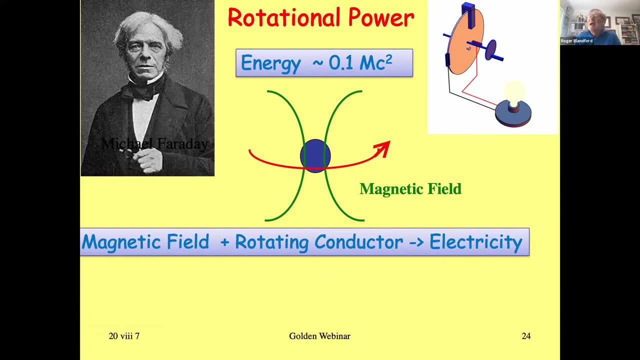 we can go from the accretion power to the rotational power, and here in the rotational power, this is Michael Faraday, and one of many, many things he discovered is that if you had a conductor spinning in a magnetic field- and that's what you have here- 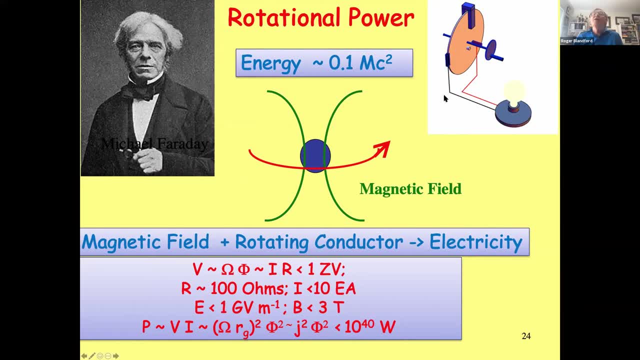 then you can drive an electrical current around the circuit and light a light bulb. And you can do the same sort of thing with a black hole. You can regard it as a sort of conductor with a resistance of about 100 ohms, and if you stick it in a magnetic field, 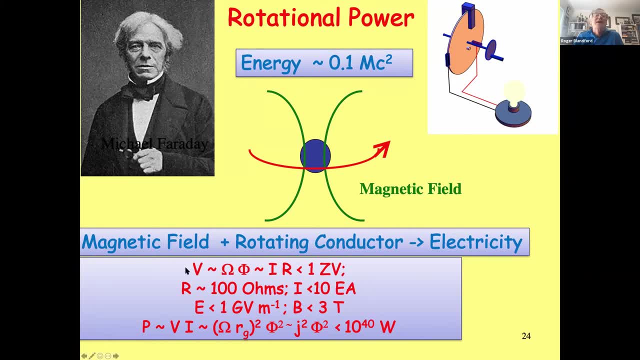 and allow it to spin, you'll get electricity out, you'll get a voltage. Those who have done basic undergraduate physics will be able to at least relate to this, this formula here that says the voltage is one zettavolt. and for those who aren't familiar with what zetta means, 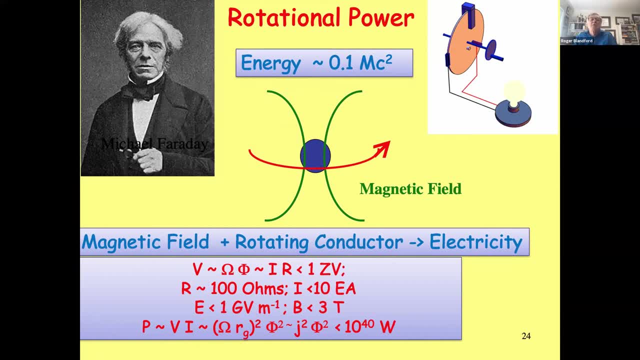 that means 10 to the power 21,, or a billion trillion volts. That's an awful lot of batteries, and the current is again equally enormous, and the magnetic field strengths are 10,000 times, say, or more. 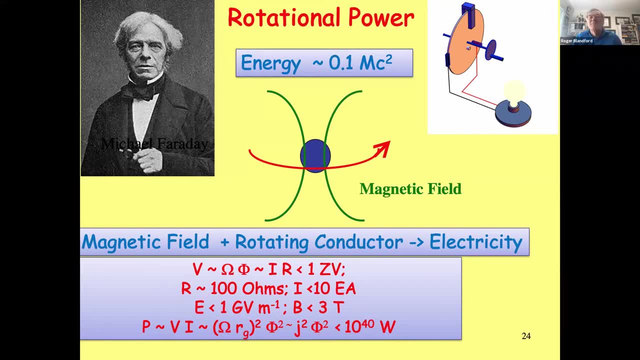 times the sort of magnetic field that you're associating with the earth. that's 100 times the magnetic field of a fridge magnet and this whole process drives an electrical circuit and that electrical circuit carries power. and that power can power compare the most powerful active galactic nuclei? 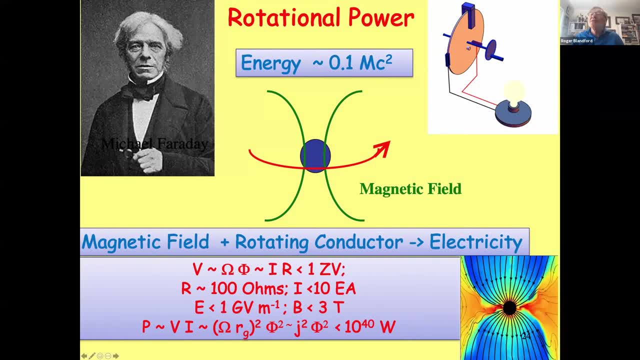 and other objects beside. So here's a simulation of this. We've got magnetic field lines shown by these lines here. Here's a spinning black hole, Here's a thick accretion disk that surrounds it, and electromagnetic energy is extracted through a process that was mentioned. 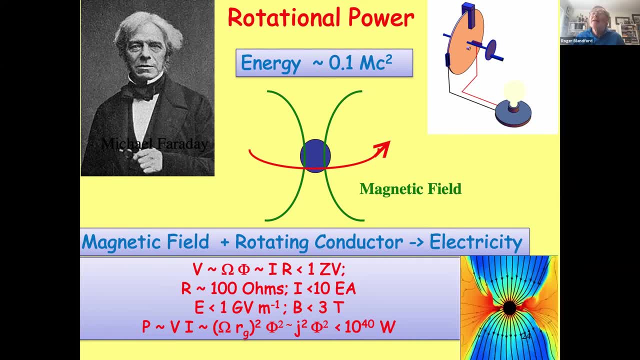 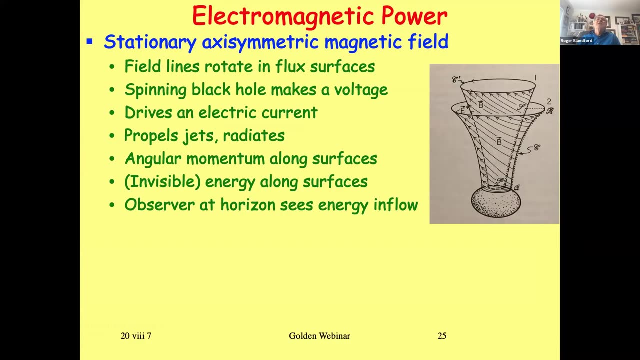 and I thought about in the 1970s and is collimated and confined by the surrounding gas in this region here. So, if we go on here, So let me talk a little bit more about the details of this means of extracting electromagnetic power. 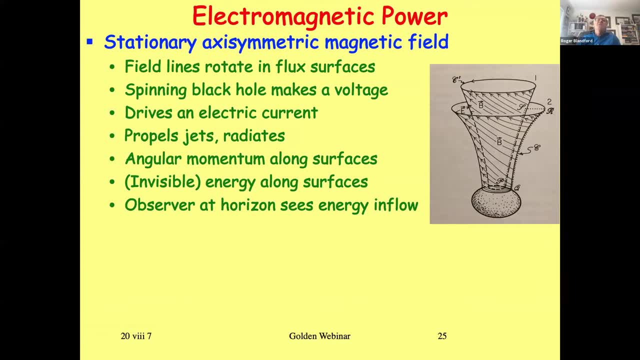 and this is a little bit of sort of physics here. but I've tried to remove all the equations and just explain qualitatively what the main points are. If one just like in the spirit of that very simple model of the accretion disk, that doesn't do full justice. 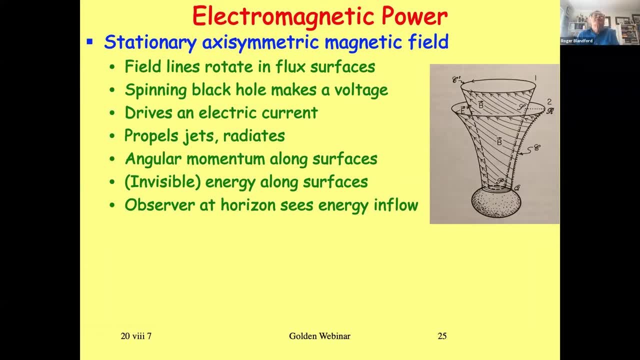 to the observations. for sure, one tries to make again a simple, steady, axisymmetric model of magnetic field, shown here threading a spinning black hole. So imagine this simple thing: here is a spinning black hole, We've got magnetic field lines, that's these lines here, like that. 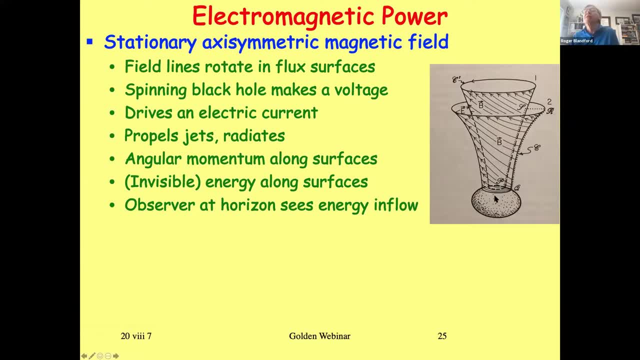 and they are going to thread the horizon of the spinning black hole. And these field lines that are wrapped around the axis of rotation are going to lie in surfaces. We call these magnetic surfaces, So they lie in magnetic surfaces. Here's one surface. 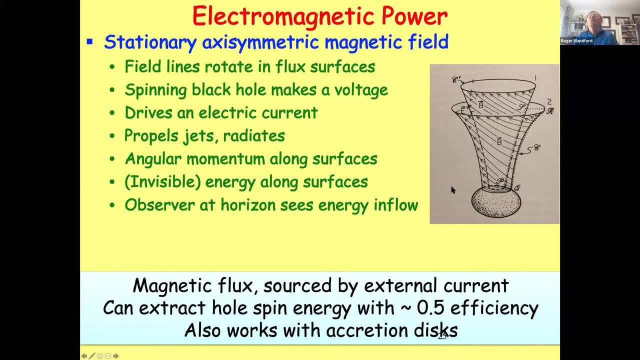 There's another surface, And so the claim is that, by this sort of Faraday effect, you're going to drive electrical current along these surfaces. There's a voltage associated with these surfaces, and we can think of these magnetic field lines as rotating. 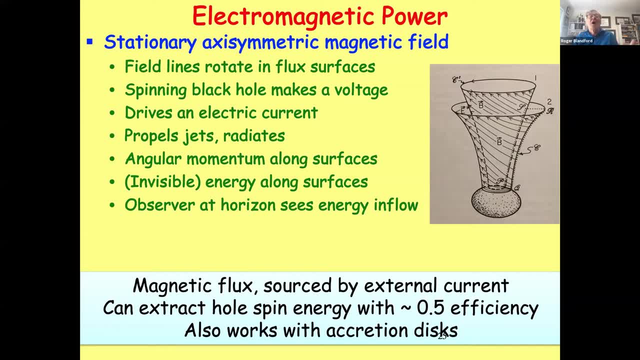 So we're going to rotate with an angular frequency that's about half the angular frequency of the spinning black hole. So we've got a black hole with an identified spin, as I mentioned before, And then these field lines are going to rotate with about half that angular frequency. 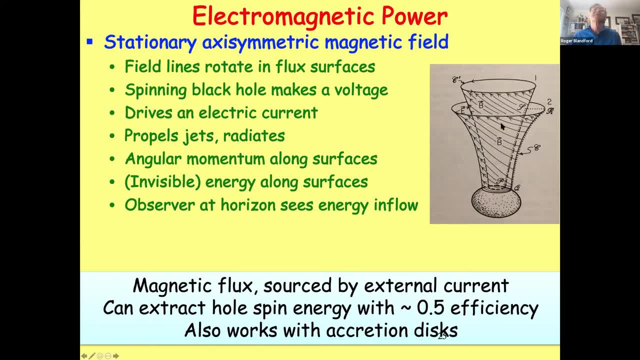 And that's going to send currents along these magnetic surfaces, take energy and angular momentum outwards from the black hole along these magnetic surfaces. It's going to extract it from the black hole along these surfaces And it's going to be essentially initially pretty much invisible. 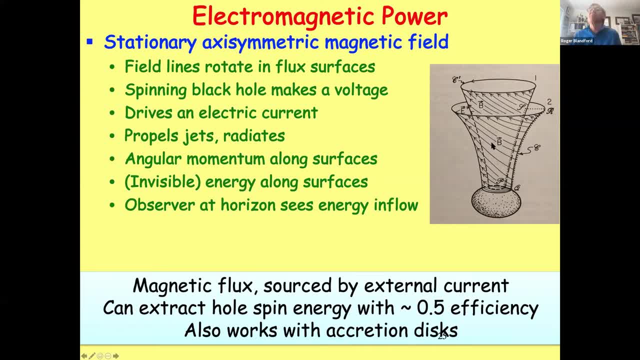 because it's just electromagnetic energy and there's no way you'll observe that directly until it starts dissipating. Now you might be worried at this point and say: but I thought energy was supposed to go into a black hole. And yes, it is. 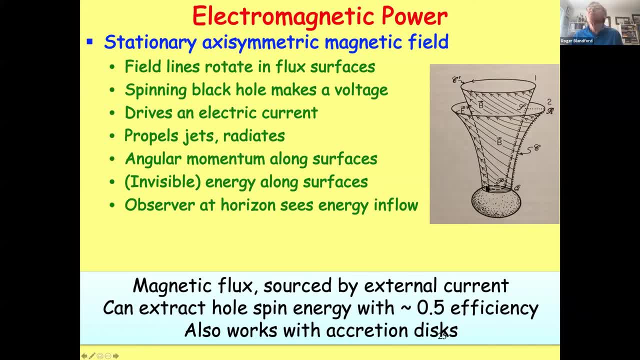 If you were an observer, as I mentioned before, in this thought experiment, hovering just above the horizon with the angular frequency of the black hole, then what you would actually see is energy going into the black hole, but in this frame that's not rotating from the outside. 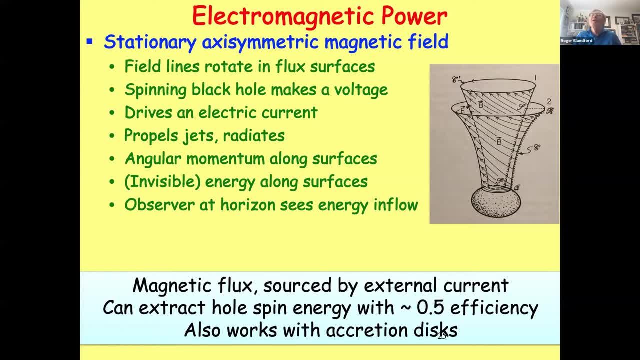 you get energy coming out. That's the sort of magic of relativity, if you like- And so you can get electromagnetic energy in this way from the black hole, And this sort of process also, I should say, works with accretion disks. 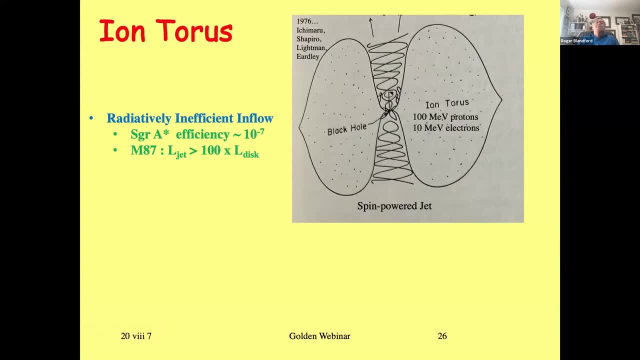 So the standard way of thinking about this- and it's an old idea going back to the 70s, and my colleagues Martin Rees and and Mitch Beigelman and I, we sort of thought about this too in the early 1980s. 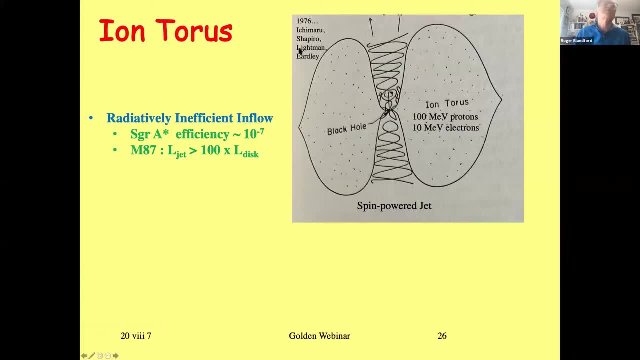 and I think this is one of our cartoons- to imagine some very thick accretion disk here with a black hole in the middle and then defining by its rotation a pair of funnels with magnetic field in the middle of it. And this thick disk here 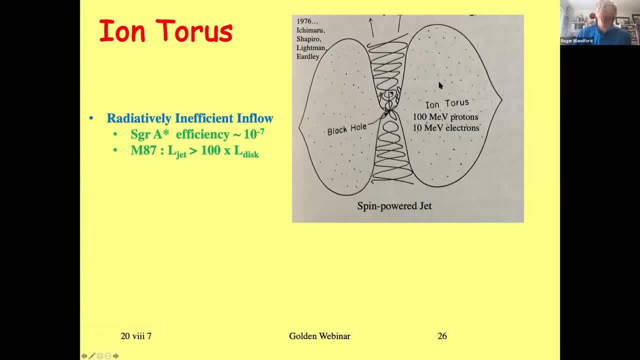 is supported by the pressure of ions, protons, of protons that are mildly relativistic with cooler electrons, And so what we have then is defining region here, this giant donut, if you like, defining a pair of funnels. 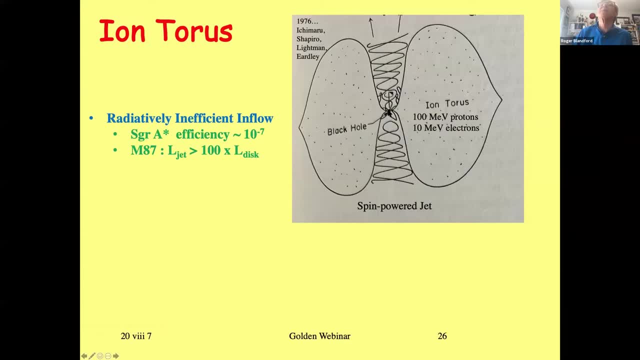 and inside these funnels outflows the jet which is powered by the spin of the black hole. That was the conception, as I say, nearly 40 years ago, and it is the basis of the sort of contemporary model and I'm going to sort of segue into it. 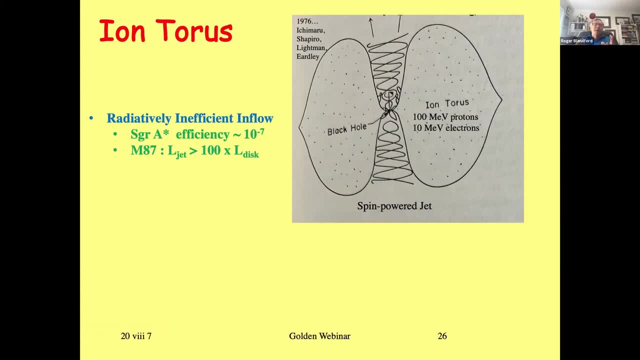 to give you a sort of almost heretical view of what's actually going on in these sources. but let me put up the standard view first of all, and why. I'm not so sure that this is what these marvelous observations made by the Event Horizon Telescope team. 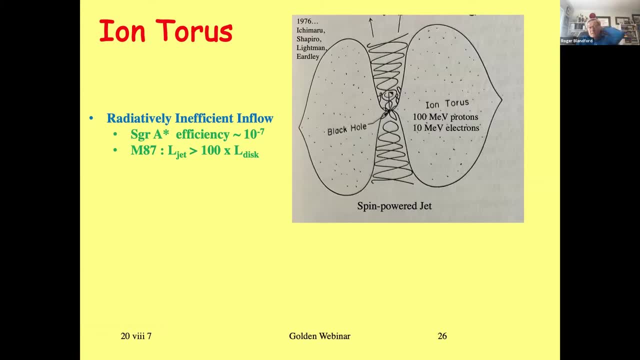 are actually demonstrating. So the problem really is that in saying the Sag A star is the black hole at the center of our galaxy, the efficiency is something like about 10 to the minus 7, so it looks like we're getting a very poor return. 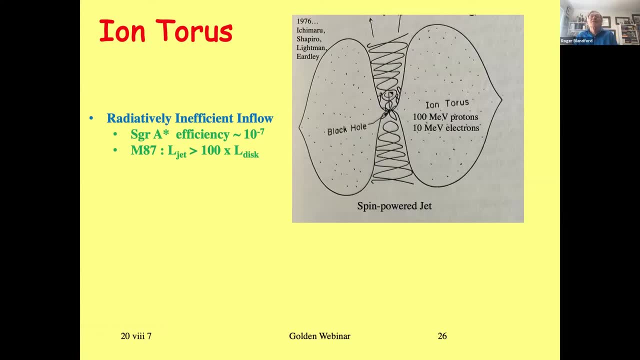 on the gas that's being supplied at large distance, And so it's very, very surprising if any of that gas is getting into the center, because it ought to be dissipating. Accretion disks are naturally extremely dissipative objects, and they ought to be very much brighter. 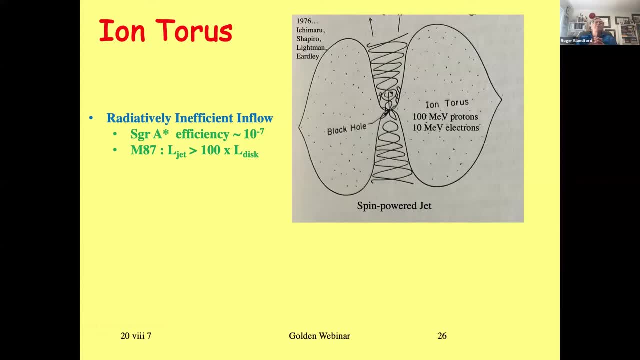 In M87, we know that the jet that's observed is 100 times or more bright, 100 times or more luminous than any power we see coming from the disk. So it looks like we've got something- the jet- when we eventually see it. 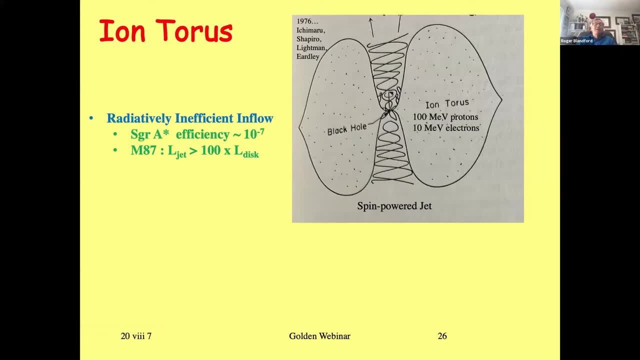 is extremely powerful. the disk is extremely faint And that's very surprising, because the problem is: can we have enough pressure here to confine these jets? These magnetic fields have to be confined and collimated by this thick accretion disk here. 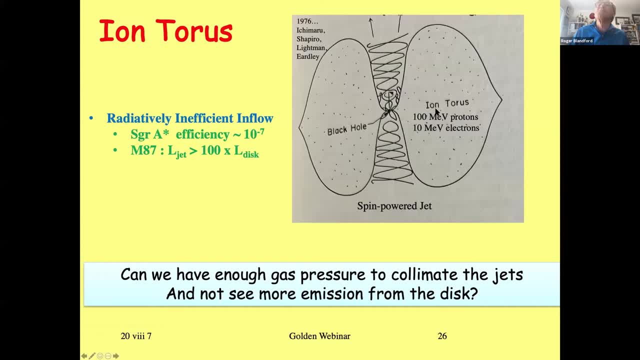 this giant doughnut without actually seeing it. This is a big, big puzzle. Let's continue. Let's give the standard view- and this may well turn out to be right, and a lot of thinking is going into this. This is made by the Event Horizon Telescope team themselves. 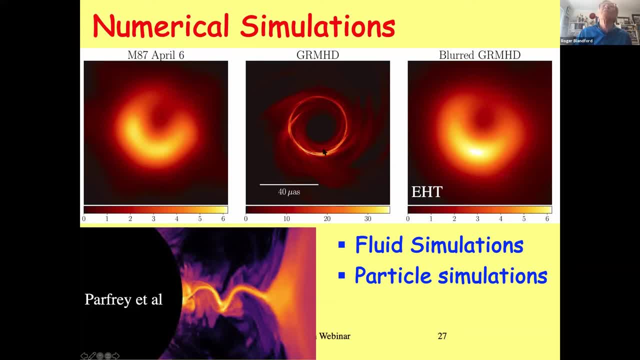 using numerical simulation. They made a model of emission with a certain set of properties from this giant doughnut and they said: this is what it would look like if you had perfect resolution and if you then blur it with the actual resolution of the Event Horizon Telescope. 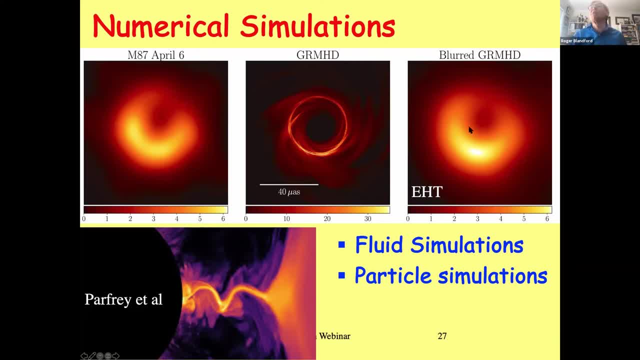 which is truly impressive. you'll get something here that looks really rather like what was actually observed, and so that's good, If we look at it not from the point of view of fluid mechanics, which these simulations were, but from the point of view of the individual particles. 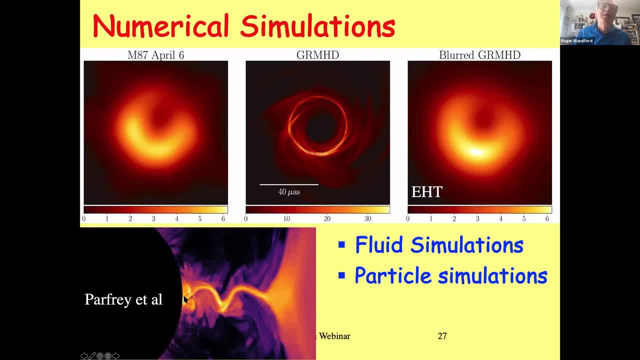 it's a rather nice piece of work that's done by Parfrey and others. They made a model and they show a current sheet here. but again it's the same story and you have gas. that's confining it, that's confining the jet. 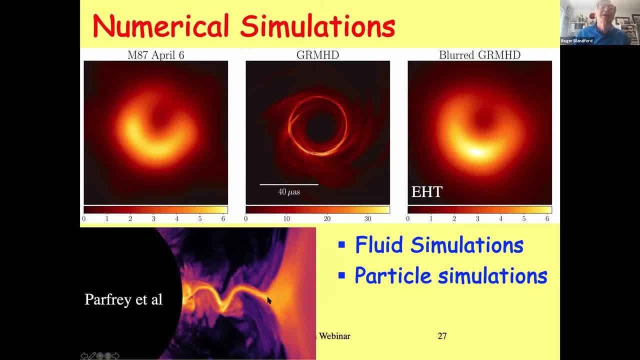 and there's the outflow and here's the black hole here, and this is a current that's flowing into the black hole in this particular model, making its assumptions, And so my question is: is this really the right model going forward? 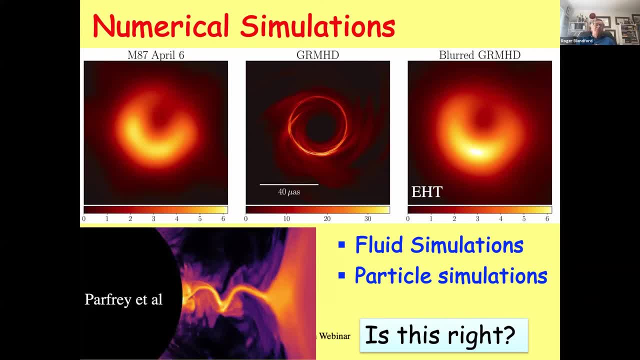 And what I'd like to share with you is an alternative conception of what is actually happening in these sources, and so let's just go on to here- And I've got here a cartoon, if you like- that contains an alternative viewpoint. I'm going to show this. 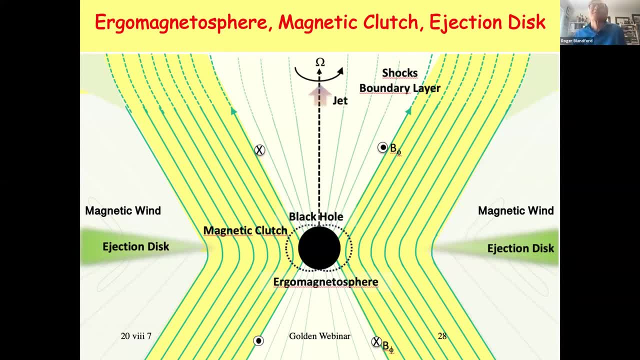 in three different ways going forward, but this is the sort of big picture, if you like. Firstly, the ingredients are. there is a spinning black hole here. It's rapidly spinning and imagine this is true in M87, but lots of other sources as well. 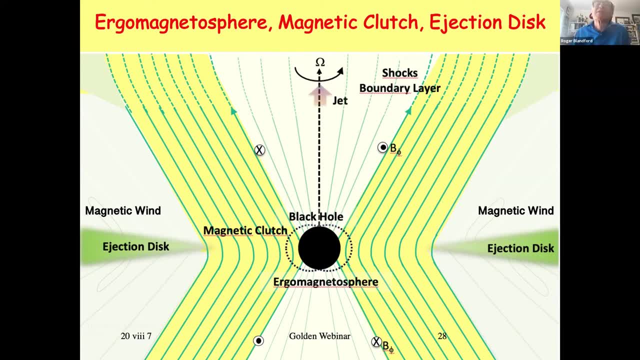 It's a source where the supply of gases is very low, unlike in a quasar, where the supply of gas must be very high. This spinning black hole has an ergosphere, which we introduced before. This is the region where an observer must rotate. 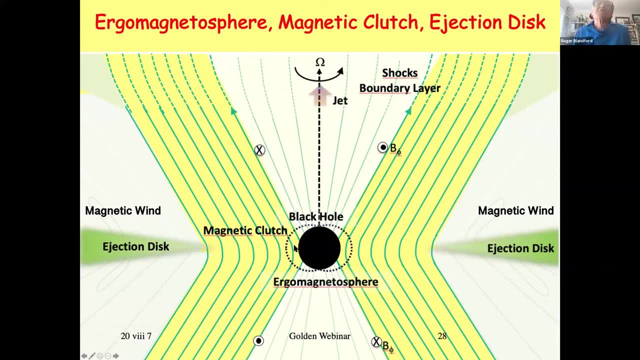 in the sense of the hole and from which you can, in principle, extract the spin energy of the hole, which is the black hole, And in this case, because it's believed to be magnetized, these are magnetic field lines that, in cartoon form, 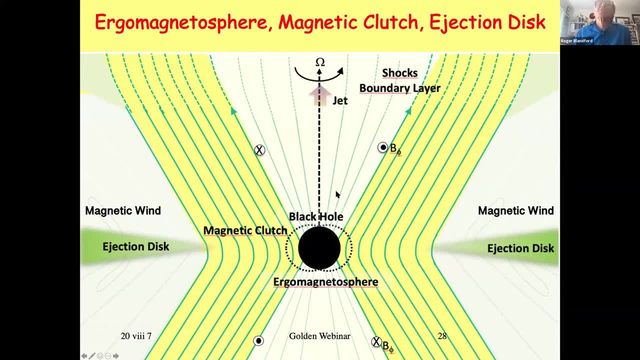 thread the horizon of this black hole and they are spun around and make a toroidal magnetic field and they send off an electromagnetic jet in this direction. The jet itself must be confined. This magnetic field must be held in place and the jet itself must be confined. 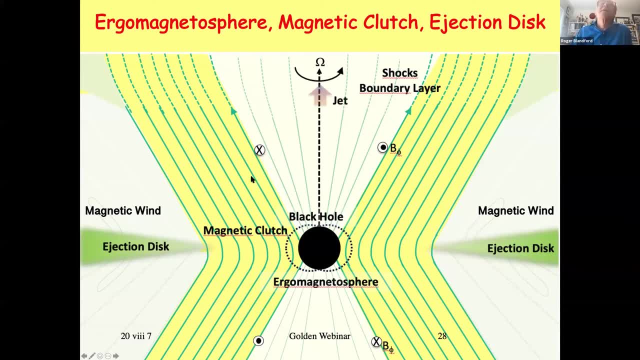 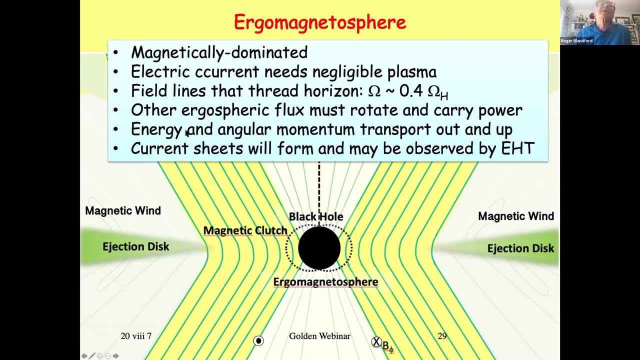 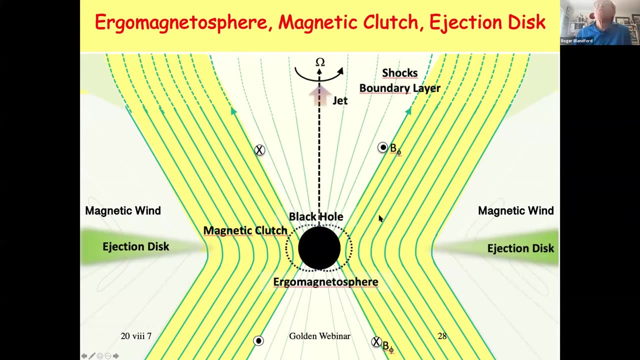 by something outside, And the conjecture here is that what is actually providing the collimation is a magnetic region. here It's magnetic field, and you get magnetic field that extends way outside the black hole that provides the collimation of this jet. Ultimately, it has to be held in place by gas. 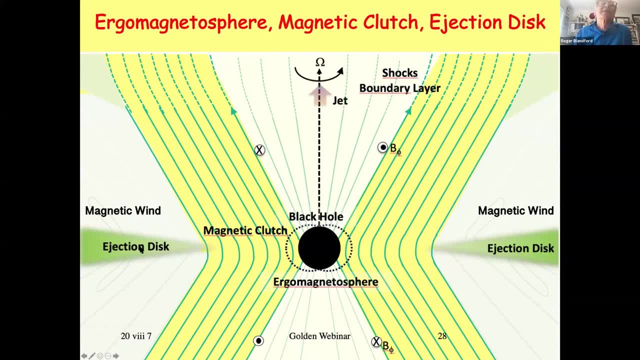 And here the story is that there is gas, there is an accretion disk. it's a much larger radius and it's being observed in that event horizon telescope image And in practice, the gas that is supplied at large radius is all ejected from this disk. 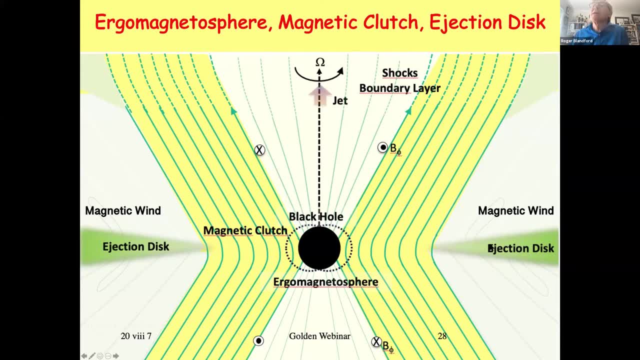 and that disk and the path of that ejection. the gas is carried off in a magnetic wind and that is energized by the spin of the black hole. So energy comes from the spinning black hole all the way through this magnetic clutch. it engages the ejection disk. 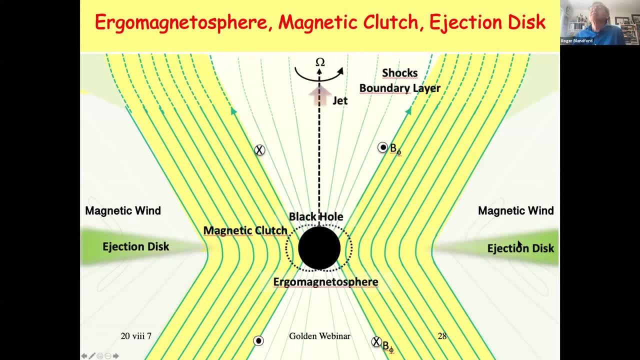 and all the gas that is supplied is given enormous speed and driven out from this so-called ejection disk. So it's an ejection disk, not an accretion disk, And there's an interaction layer that will start to develop up here. 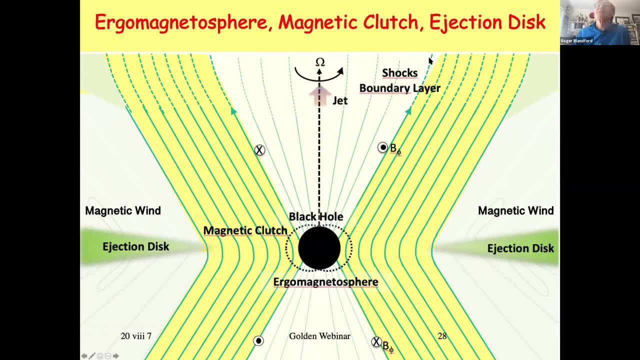 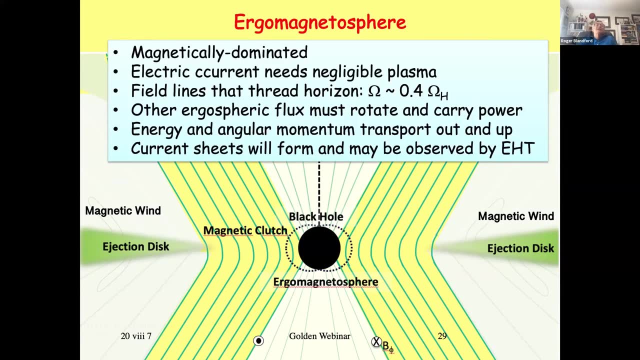 and this is what you start to observe schematically in those observations of the boundary layers of the jets. So just to summarize the basic point here: the idea is that what is observed with the event horizon telescope is magnetically dominated. there are electrical currents. 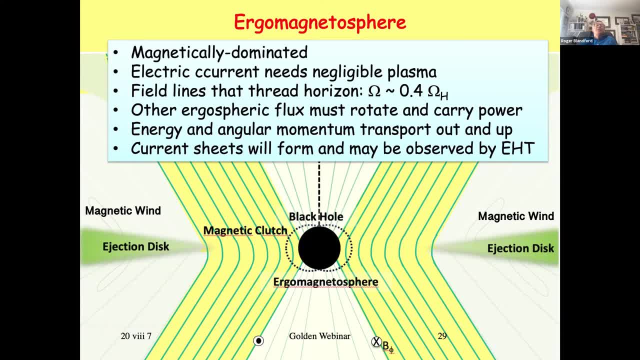 for which you need negligible amounts of gas, and the field lines thread the horizon and are rotated at about roughly half the angular frequency of the hole, and energy and angular momentum are transported not just outwards along these field lines into the jet, but are transported outwards. 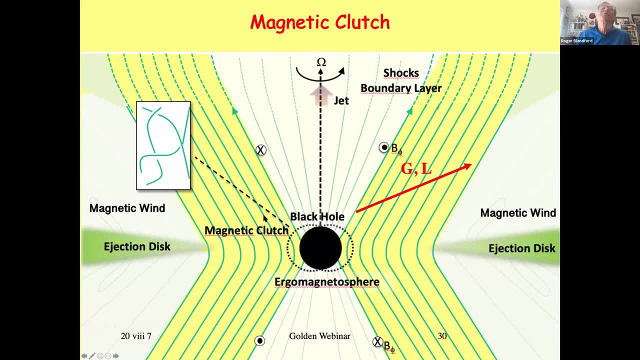 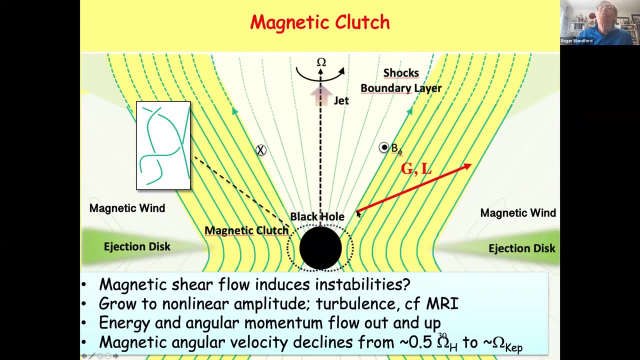 as shown in this cartoon here. This is the same cartoon, if you like, and the point is that the energy and the angular momentum that are liberated by the black hole are transported outwards as well as out along the jet. like this, they also go outwards. 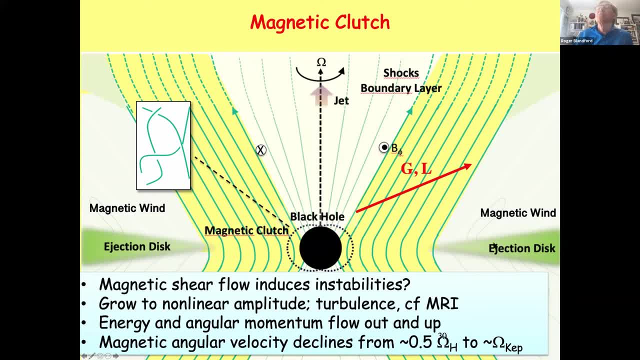 and so they can power the outflow from this magnetic wind, from the ejection disk. So this spinning black hole powers the out ejection disk that carries away all the energy, and the means of doing this is relying on magnetic instabilities that operate in this region. 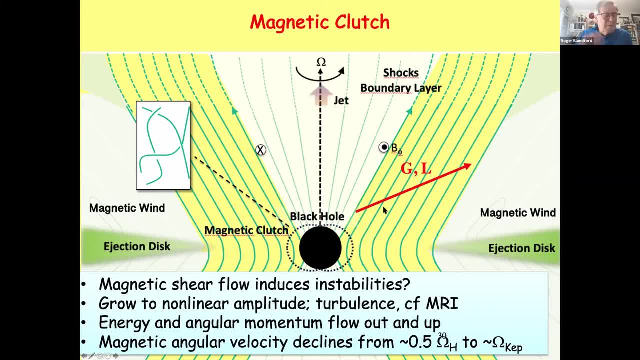 very similar in spurious to those that are believed to take place in regular, proper accretion disks, regular accretion disks where there are magnetic instabilities and that is responsible for the friction of the accretion disks. The claim is that there is the same sort of friction. 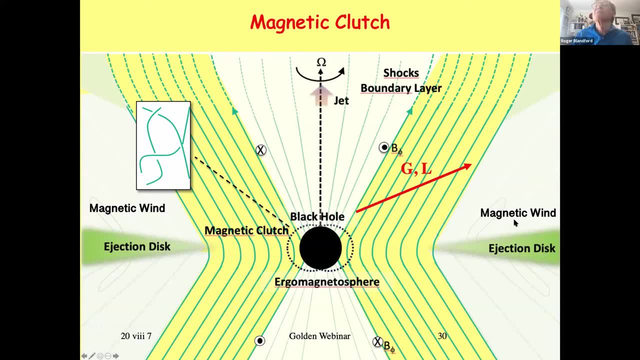 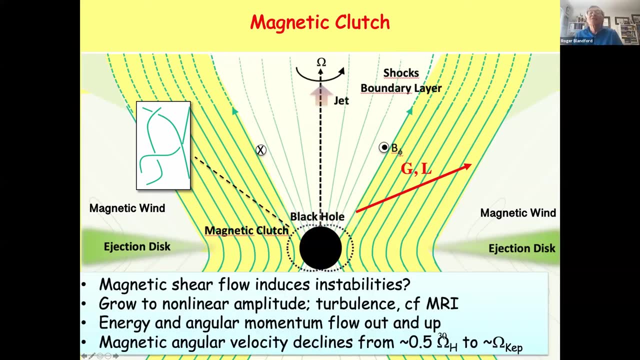 that happens in this region here, which allows energy and angular momentum to be transported outwards and to power this ejection disk. So the idea is that there is instability here and these field lines here make this clutch and what you're actually looking at. 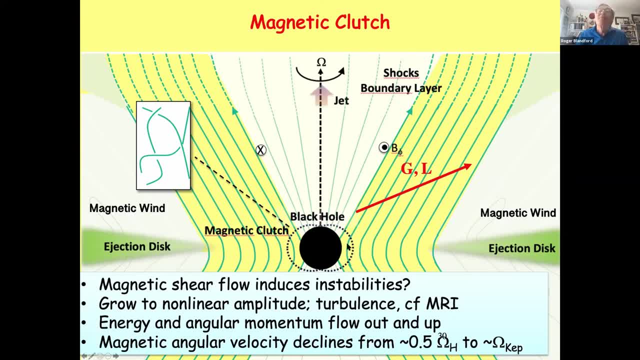 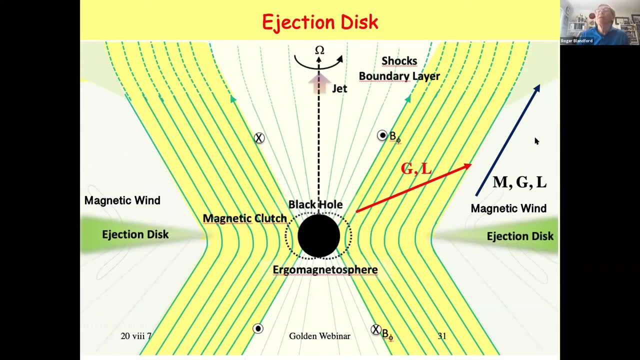 with the Event Horizon Telescope is a magnetosphere rather like in a pulsar, not a thick ring of orbiting gas as in the standard model. So here's the ejection disk, here's a magnetic wind here that's invading the energy outwards. 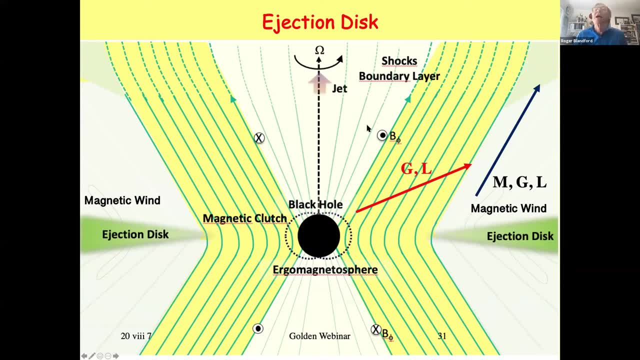 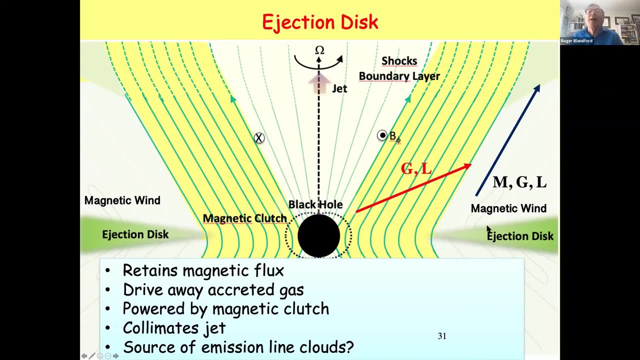 and this wind is responsible for shaping the jet, as observed by the radio astronomers, and it also could be the source of emission line clouds. The ideas that I'm sort of sketching here. they have some basis, but they're still somewhat conjectural. 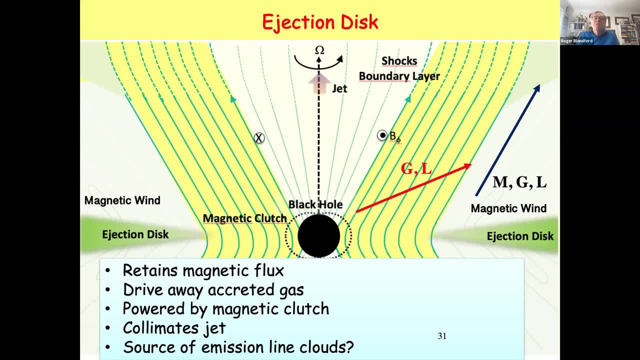 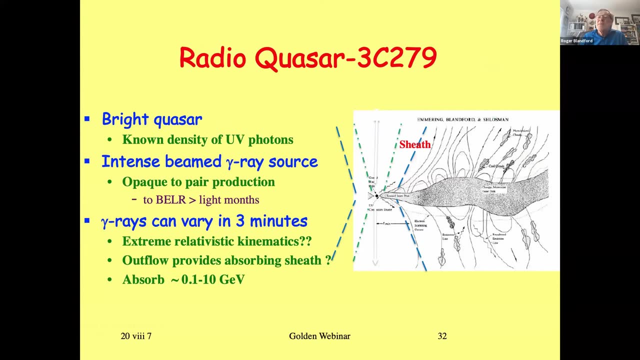 but they do have implications for many more types of source than those epitomized by M87.. If I just take another radio quasar 3C279, it is an amazing source, not the least for its gamma-ray properties, and it is able to vary on timescales of three minutes. 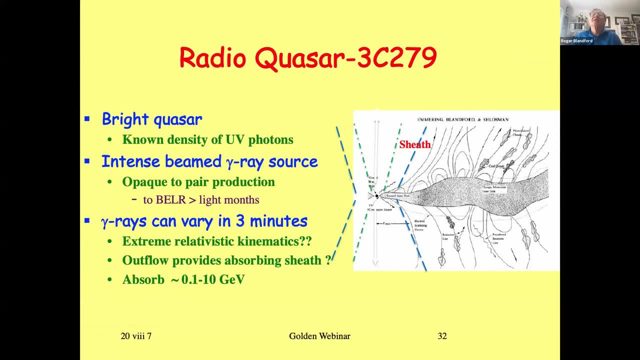 and this is a great puzzle, because the gamma rays that are seen can't- you'd have thought can't- come from very close to the black hole, because there's a lot of ultraviolet radiation there and those gamma rays react with ultraviolet photons. 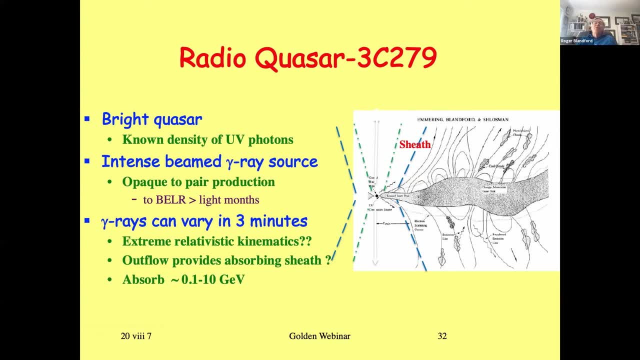 which will prevent their escape. So somehow or other you have to shield those gamma rays made close to the black hole by gas on the outside. and the application, the ideas I've just sketched to this source, are that you have a sort of a sheath of gas. 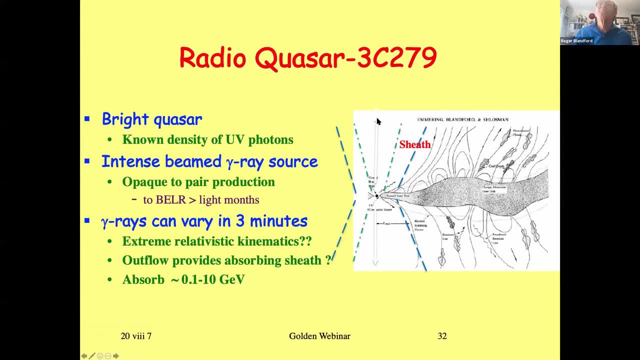 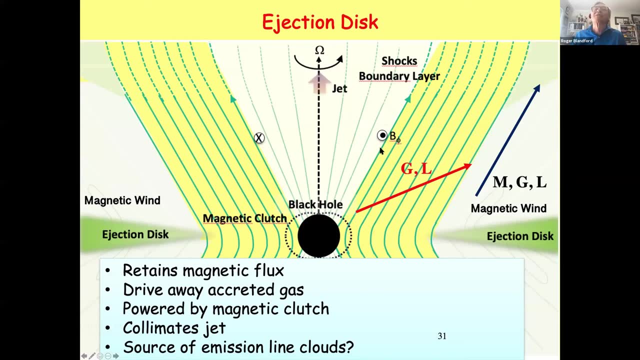 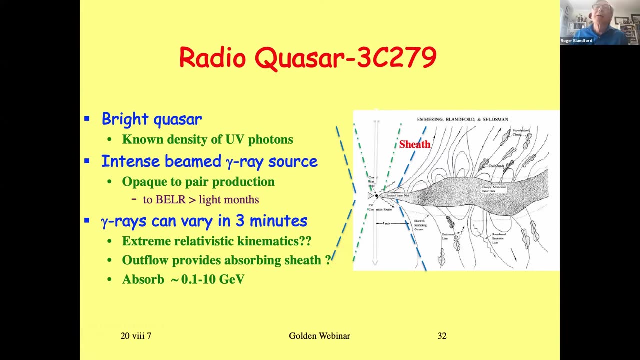 that absorbs the ultraviolet photons and when an astronomer looks right down the jet from this direction here, looks right down the jet, then it's able to see right down to a region where there aren't these reacting ultraviolet photons and the gamma rays can escape. 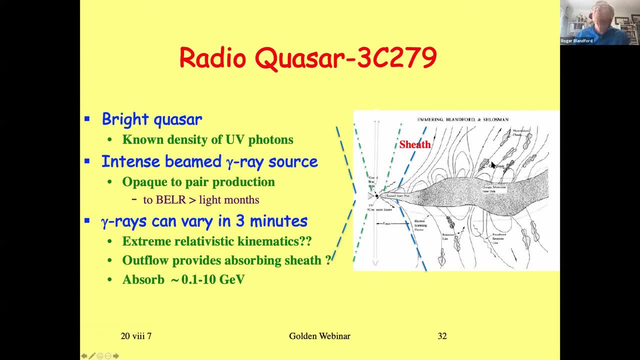 So that's one of the story, one part of the story. Another part is that the so-called emission line gas- for the astronomers who know all about this business- that's actually derived, that's the outflow from this accretion disk. 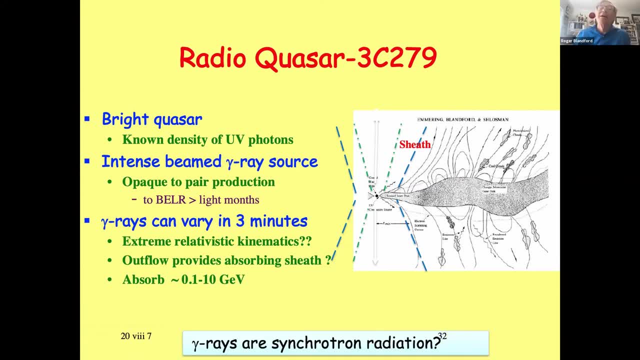 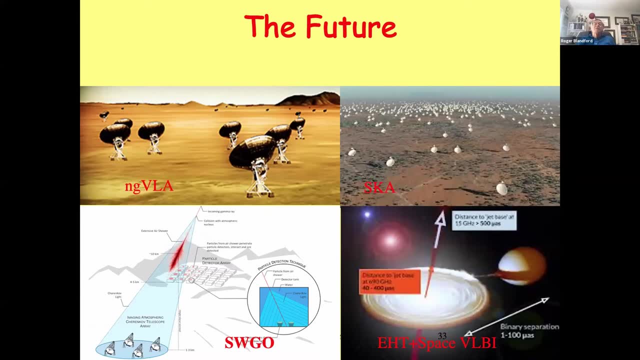 So I'm not going to take this any further here. Let me just say: finish with the concluding slide is that the future is very bright in this business. There are two major radioastronomers that are going to be involved in this project. 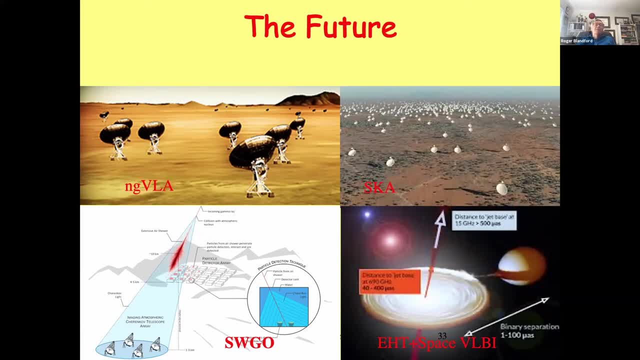 One is gamma ray astronomy projects which will complement ALMA at lower frequencies. One is next generation VLA, which is a US version, and there's a more international version, the square kilometer array. I hope that sometime in the future. 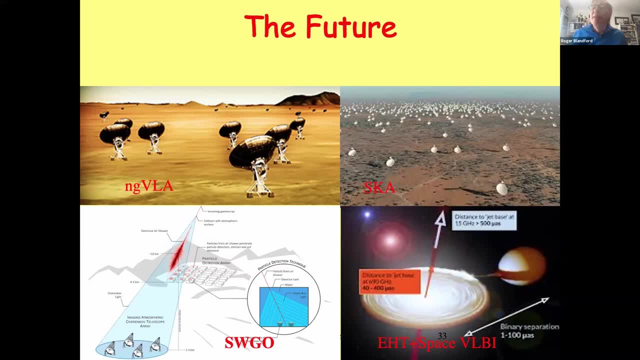 that these will essentially merge into one effort as they are somewhat complimentary as currently conceived. In addition, gamma ray astronomy, which I have not done justice to in this talk, one of the exciting things happening is the South American Wide Field Gamma Ray Observatory. 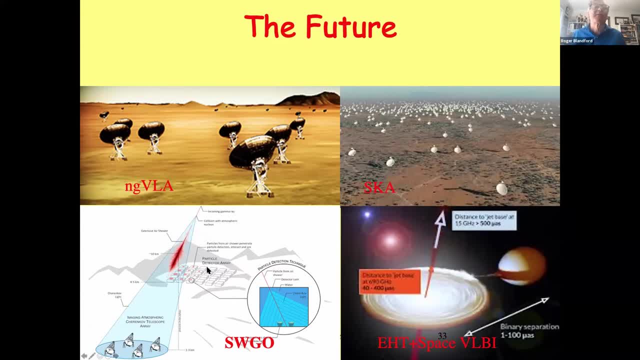 which is under intense discussion. I can't tell you which South American country it will be in, but I can tell you its altitude, which is very important. but it's a very exciting possibility because a lot of science is already being seen at these very high energy gamma rays. 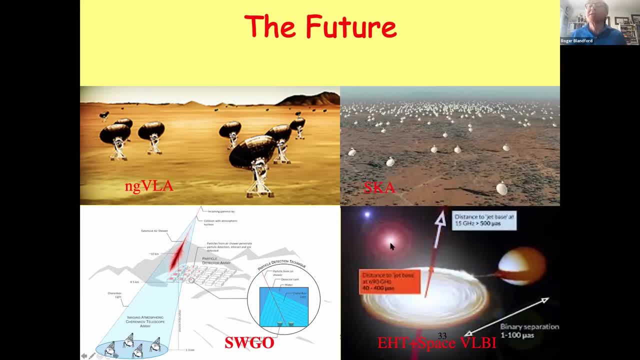 And then if we consider the Event Horizon Telescope, in which ALMA is, as I say, the anchor- going out into space at millimeter wavelengths is a dream of many of us- And then we'll have even better observations of more and more sources. 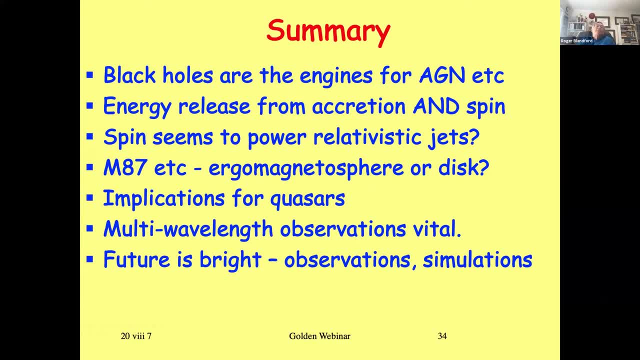 So my summary is basically- I hope I've been able to communicate- that the evidence for black holes being the engines for active black nuclear and much else besides- energy is released from accretion and rotation and the spin appears to power the relativistic jets. 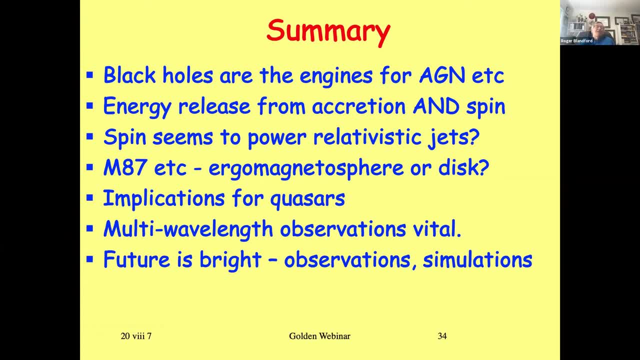 And I tried to sketch how that might happen. I've conjectured that in M87, it could be an ergo magnetosphere, a constructible magnetosphere, a portmanteau word, if you like- that the astronomers are looking at. 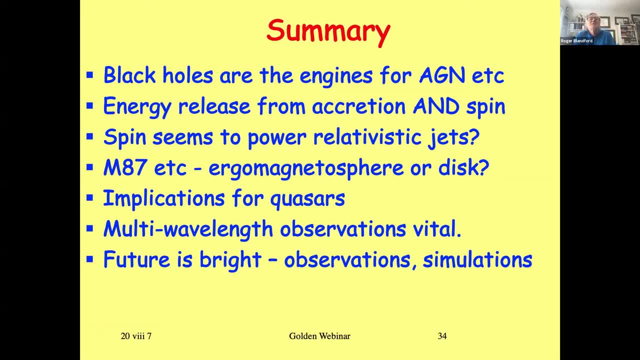 not a thick accretion disk, and this has implications for quasars. And I have two other things that have come out of this talk. The story is being told by astronomers working throughout the electromagnetic spectrum and beyond, and the future is bright. 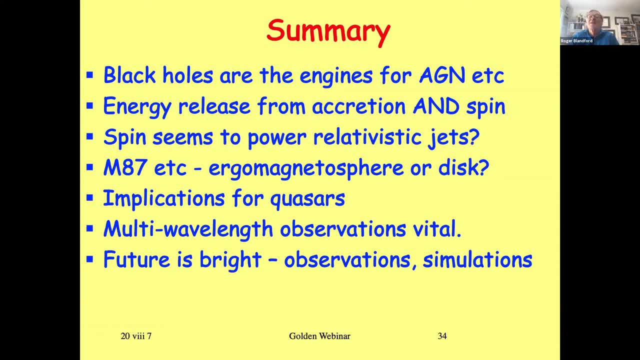 not just for the observations- which are very exciting- that are coming, but also for the ability to do simulations and so on And test some of these sketched ideas. I thank you very much and I have to say: do keep yourselves well. 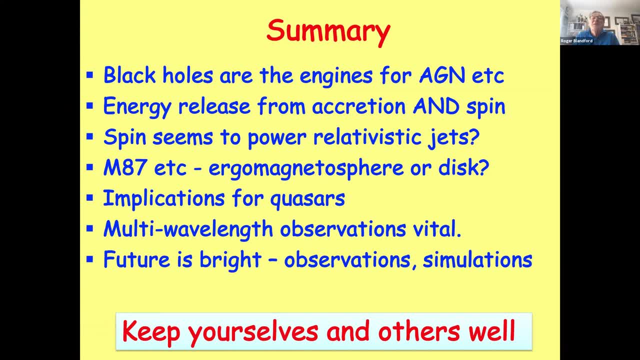 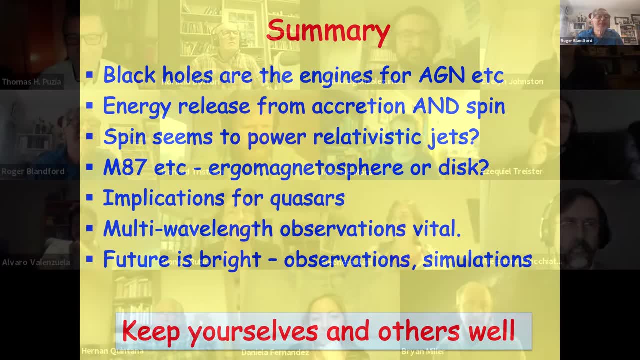 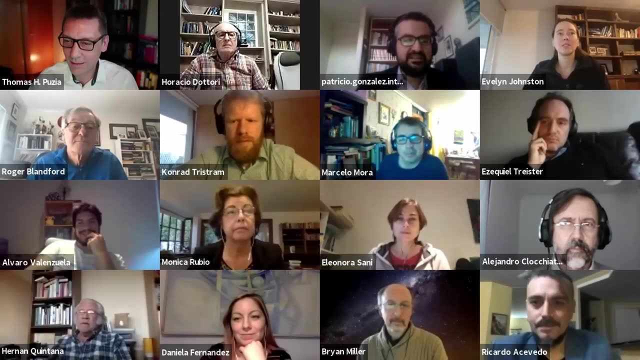 and pay attention to others at the same time. Thank you very much indeed for listening to me, and I'm very eager to take questions. Wonderful. Thank you very much, Roger, for this fascinating, beautiful overview. We have quite a few questions. 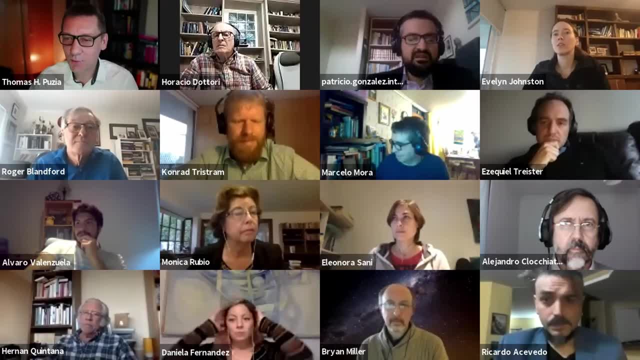 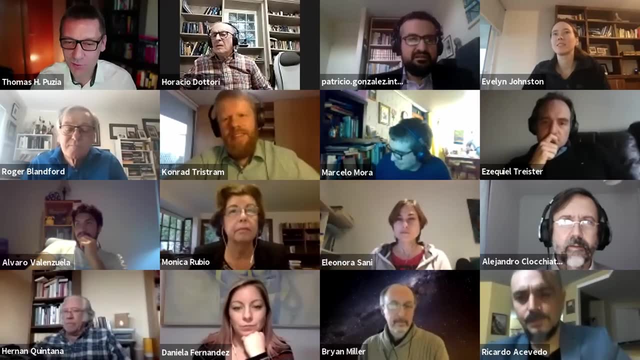 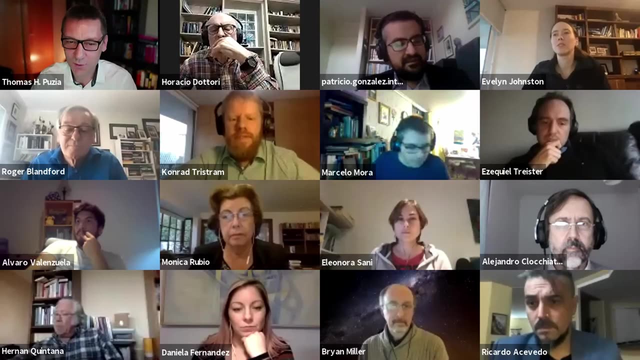 There are a few questions on the panel, But I'm going to take my privilege of asking the first question. There is something that is called the ISCO radius right, The innermost stable circular orbit that correlates in radius with the angular momentum of the black hole. 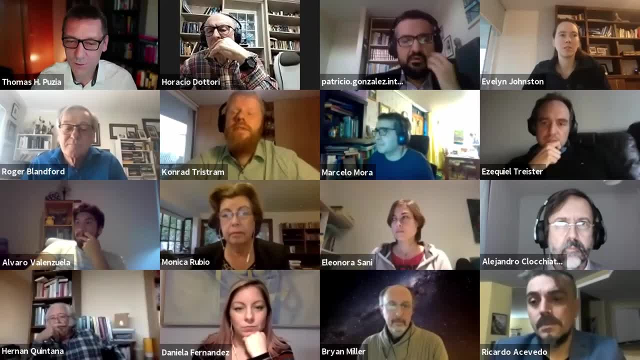 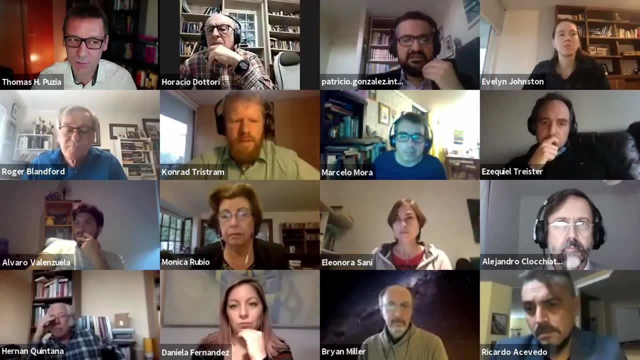 So in your picture would that mean that the faster that the black hole rotates, the more efficient the jet formation and the inflow of material actually would be of feeding the collimation? Would there be a correlation expected there? Thank you very much. 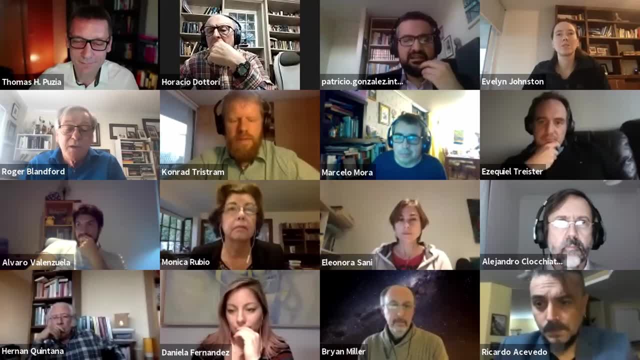 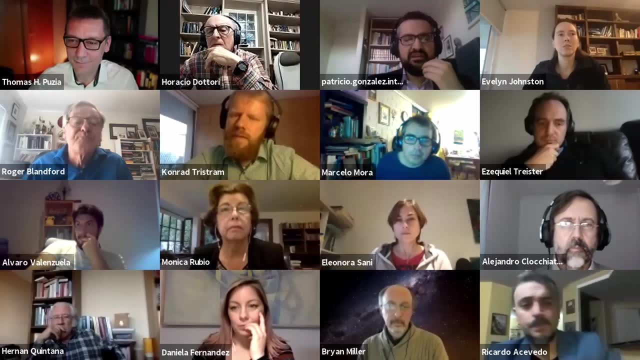 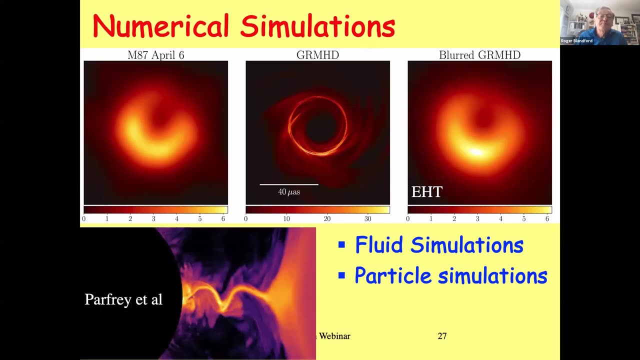 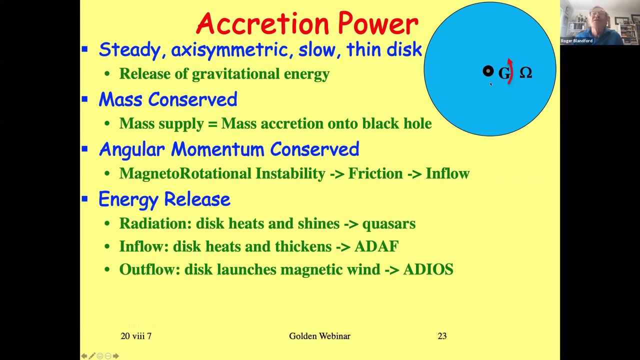 I'm really glad you asked that question because, as you appreciate it, it brought up one of the points I didn't have time to make. If we go back to Okay, this is the one: Take this thin accretion disk here. 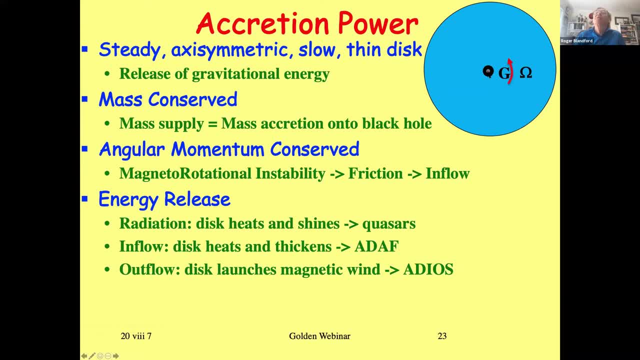 you'll see, I've actually got a gray hole in the middle for some reason, but it's a black hole, and then there's this region around it, And if you just imagine gas in orbit around this black hole, then it turns out that the circular orbits. 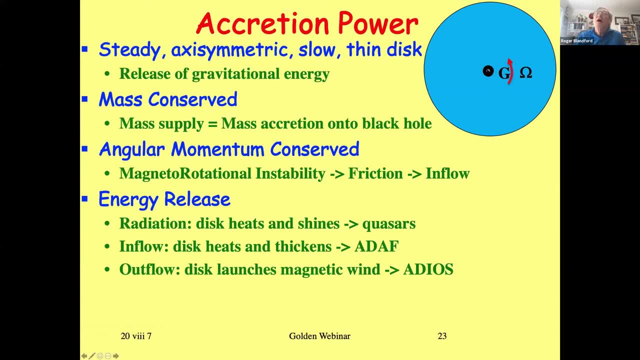 within this region here are unstable and the gas in this region must just spiral rapidly into the black hole. So, as Thomas said, there's an innermost stable circular orbit, or ISCO for short, and that in this particular cartoon would be at that radius there, like that. 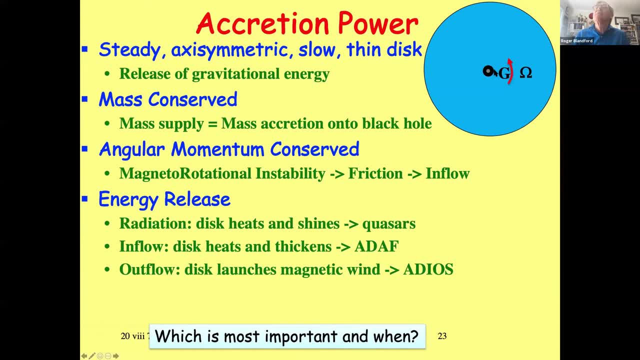 So that would be the innermost stable circular orbit. Now, if you like the oversimplified classical not matching up to the job theory of thin accretion disks, then what you would say is: the gas spirals inward, it liberates all its energy as radiation. 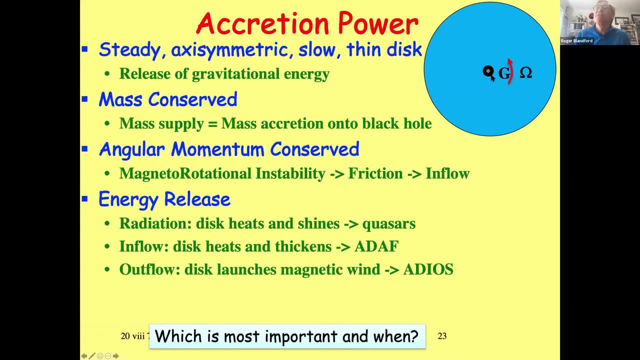 until it gets to that point, and then it just plunges into the hole and you don't get any more radiation out of it. Now the location of the ISCO, the innermost stable circular orbit, depends on the spin of the hole. 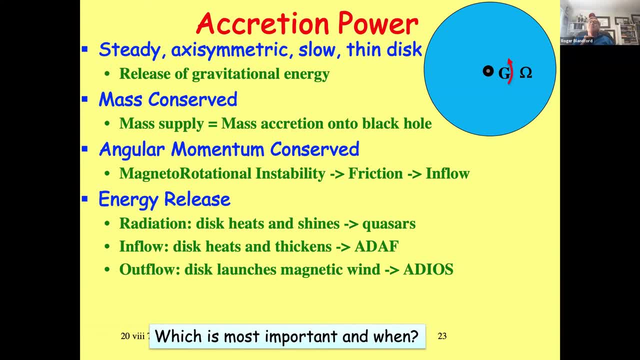 It is at six times. it's got certainly three times the radius in some coordinate system of the event horizon in a non-rotating hole, but in a prograde rotating hole going as fast as it can, it's essentially right on top of the horizon. 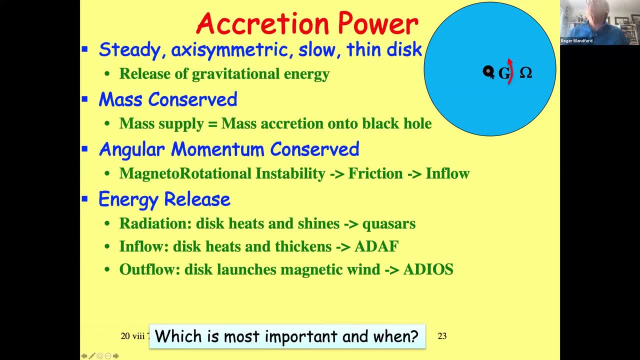 It's not quite on top of the horizon, but it's almost on top of the horizon. So there, and so you get a very efficient release of energy from that region. Now, what I actually think is going on is that in the story that I told, 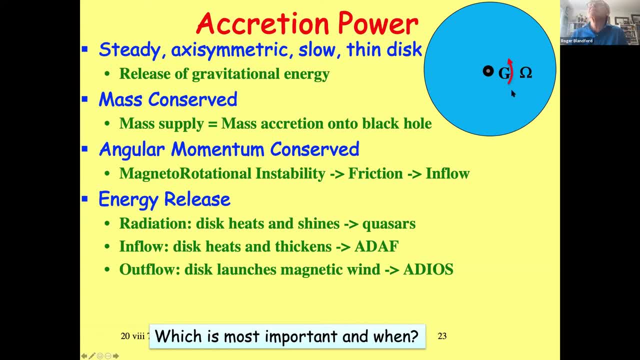 you don't have a thin accretion disk like this. You have enormous transport of energy and momentum outwards, rather than this passive accretion disk here. So and so the ISCO is essentially irrelevant to this story, And in the particular, 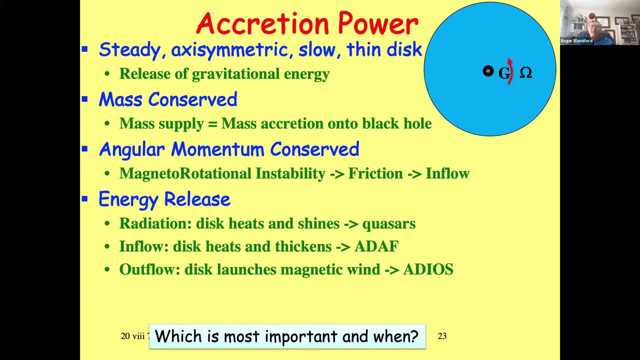 you know- cartoon that I showed, if you like, and there's a bit more to it than that- then any appreciable amount of gas is a very large radius compared with the size of the black hole And essentially everything that's supplied to the black hole. 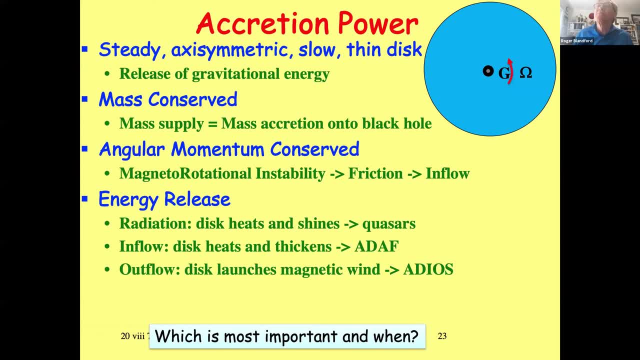 is more or less everything, not all of it, but most of it is going to be driven away in the magnetic wind. And so in this particular type of source, in this particular type of model, the ISCO is not important. What is important is the ability. 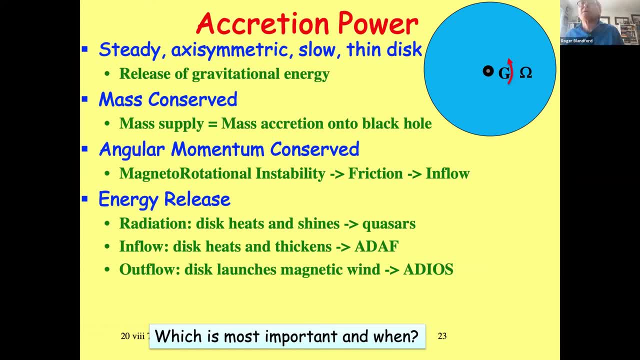 to trap magnetic flux within a much larger limiting radius and then have that efficiently extract energy from the black hole. However, other types of accretion disks, particularly those associated with stellar sources, may well operate in this way, And then the ISCO is a very important concept. 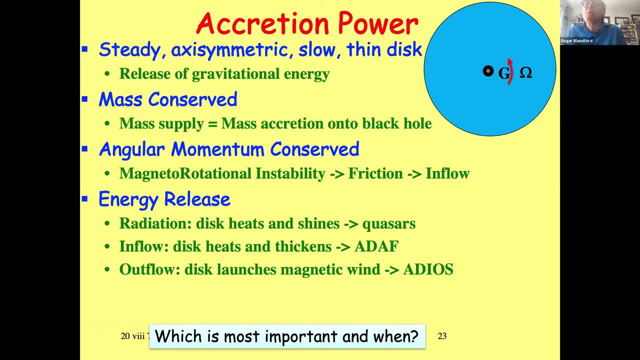 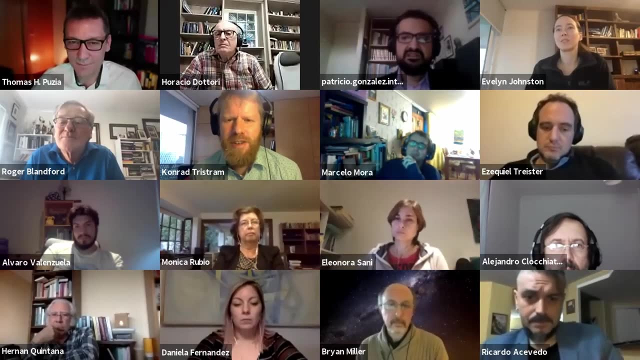 and you get more power out when you have a pro-grade spinning hole. So thanks for answering the question. I see that Konrad has a question. Konrad, would you like to go ahead? Yes, Actually, this question is almost related to where you were just finishing off now. 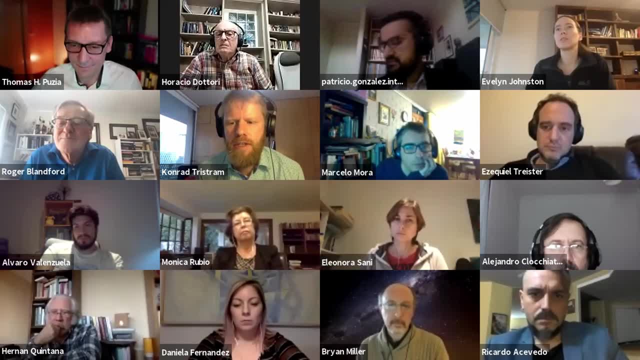 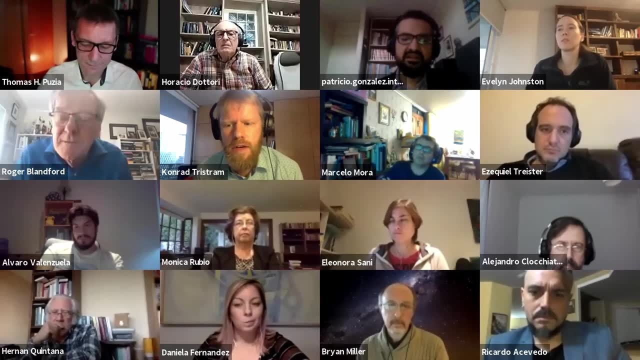 So, if I understood you correctly, you proposed that the formation of the jet, in AGN at least, is driven by the extraction of energy from the rotating black hole in the ergosphere. So, as you just mentioned, there's also other jets observed for non-relativistic objects. 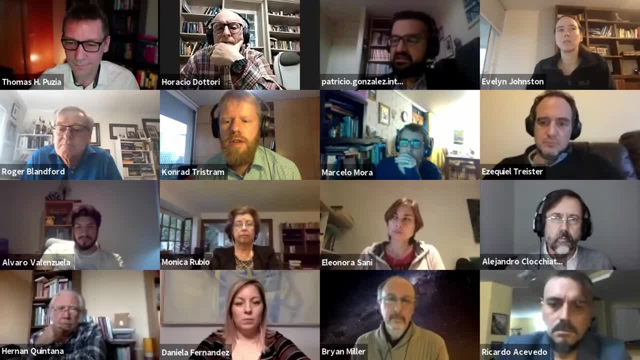 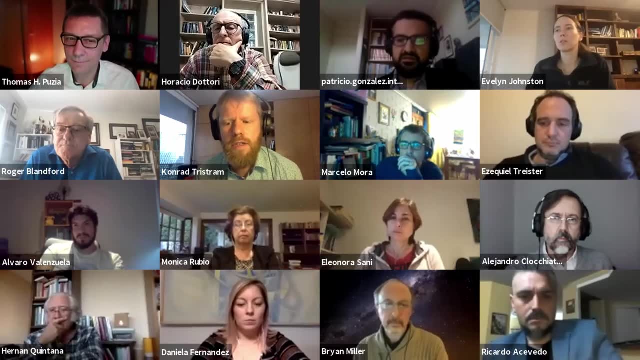 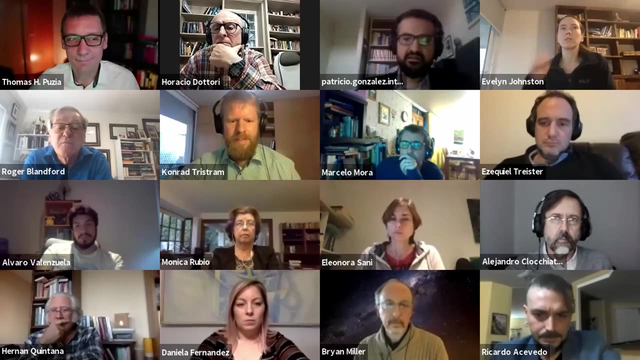 like young stellar objects and so on. So do you think there is a way for us, as an observer, to find the difference between the jets driven by accretion disks and by black hole spin-driven jets? Excellent question. Again, you've put your finger. 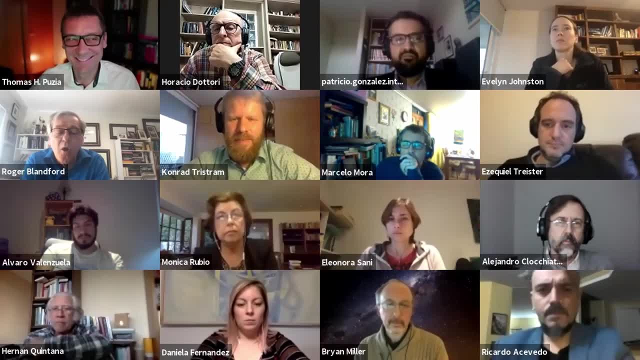 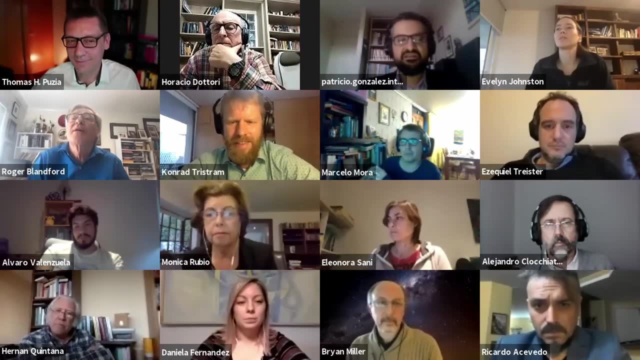 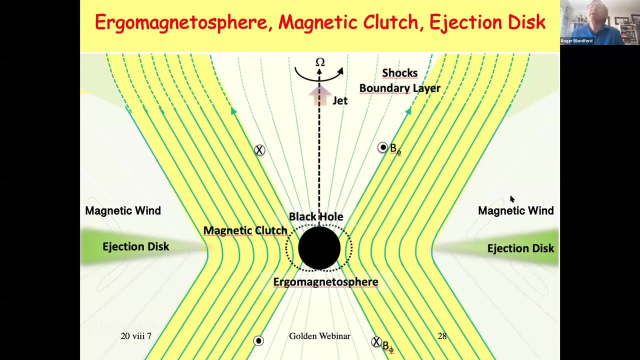 on one of these observational or phenomenological choices that have been there for a long time, And I'm going to go forward. I think Let's go to this one, That's right. So, basically, those of us who saw these jets as being essentially magnetic, 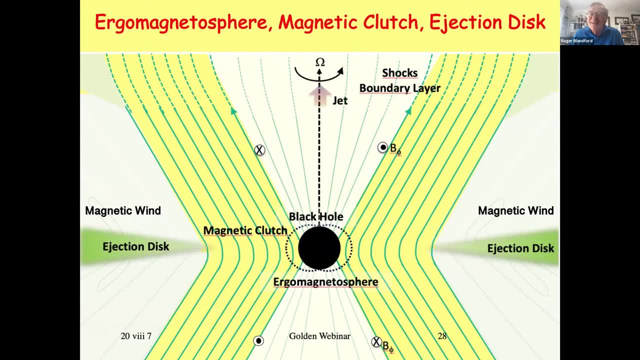 or hydromagnetic or electromagnetic, take your pick. structures were faced with two choices: Either they were powered mostly and again everything's present. but the question was: how did they dominate? Well, they were powered mostly by the spin of the hole. 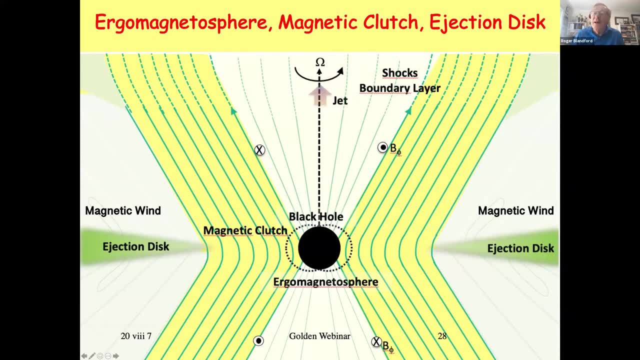 in which case it was the field lines that came to the horizon of the black hole, Or, alternatively, they were: forget the black hole, say it's just not important, it's not spinning, or something. They were powered by the magnetic field threading the accretion disk. 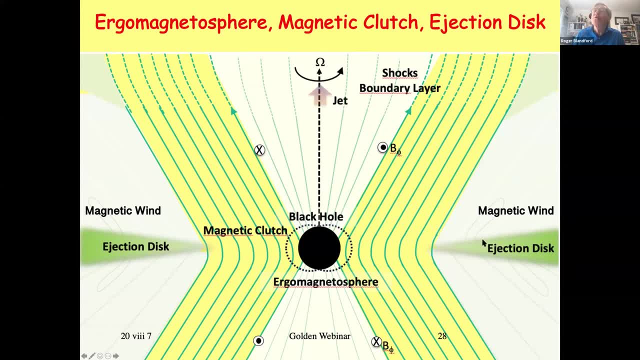 And David Payne and I and many others thought about ways of taking the energy out of the gas in the accretion disk, taking it off in a hydromagnetic wind, and that wind is able to take away all the energy and it could in practice be the jet itself. 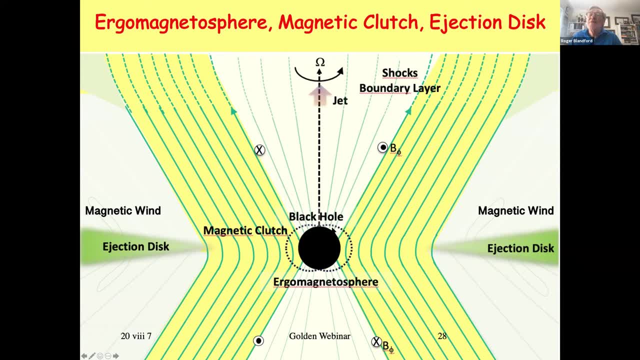 Now I think most of us believe, for two reasons, that in the quasars, with the relativistic outflows and so on, it comes from the black hole. Most of the power comes from the black hole And that's because you're seeing the rapid motions. 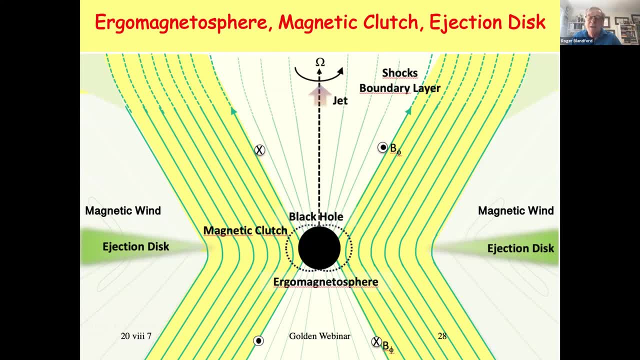 the ultra-relativistic motions, You're seeing a highly evacuated, invisible region which you can get from a black hole, whereas this is going to be much more luminous And observationally now one's tracing the jets down to very tiny radii. 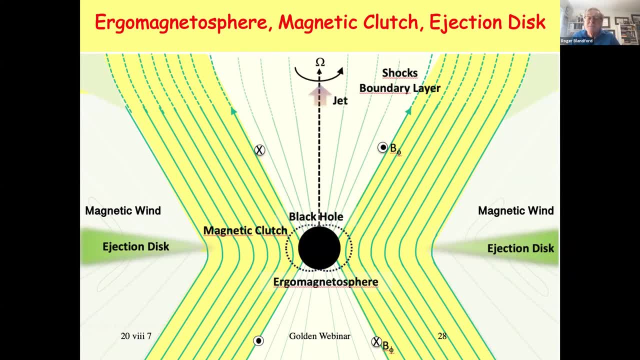 They're not coming from accretion disks. Now, that's the mechanism that's believed to happen in the AGN, but there are many sources- low-power AGN- and there are many other sources. So if you have a protostellar disk, 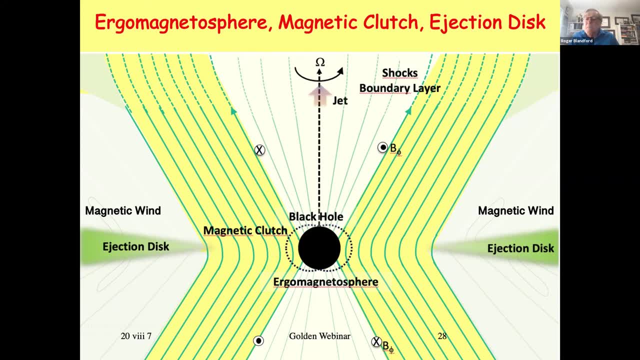 nobody says there's a black hole in HL tau and so that has to come from. probably mostly the path of that must come at much slower speeds from the accretion disk, But even then there is a possibility that you can have an analog of the black hole. 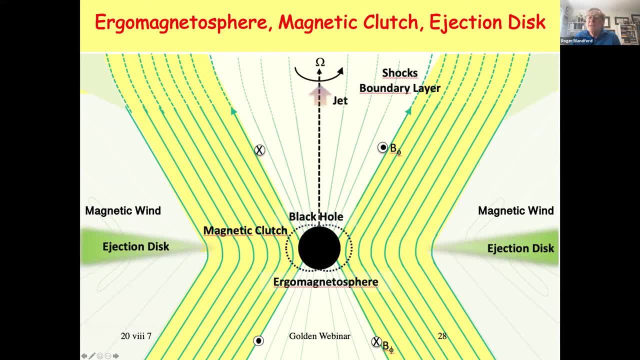 say in a protostellar disk like HL tau, because if you have a slowly rotating star, most of these protostars are believed to have a black hole in HL tau. So there'll be a boundary layer here between the inner edge of the accretion disk. 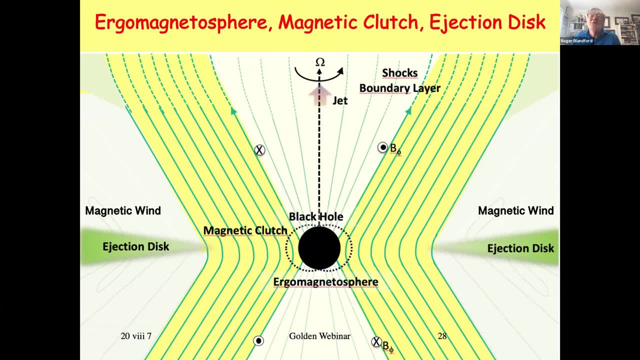 and the star itself, and you could get a lot of dissipation there. So you could have some crude analog of the operation of a black hole, but in a highly non-relativistic context in these other types of sources. George Novy can do the same sort of thing. 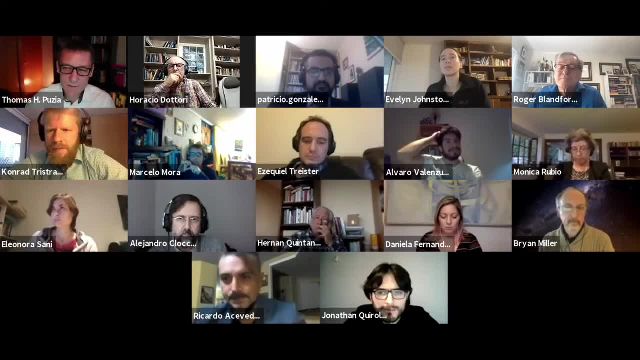 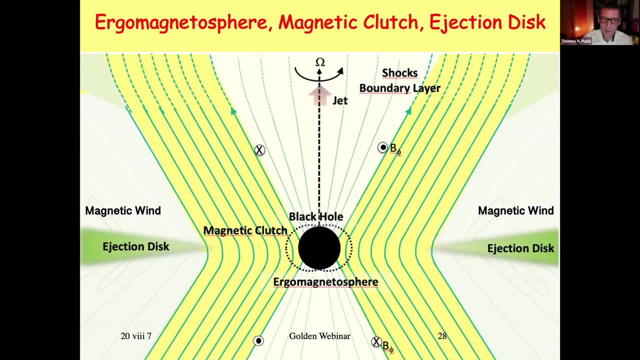 So thanks very much, Conrad, for questioning. I have just a slide up here, just a conceptual question: Does the handedness of the magnetic field actually flip at the top of the graph here and at the bottom of the graph? Oh, wait a minute. 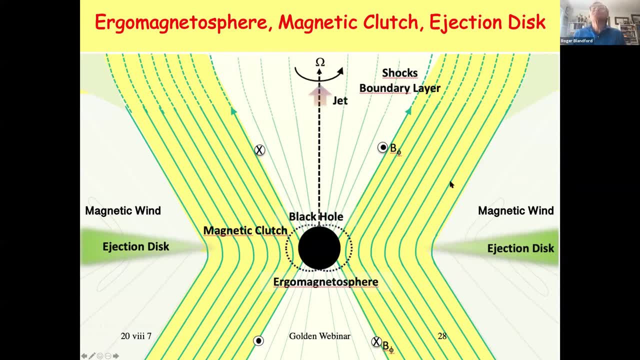 The magnetic field lines, as shown here, are what I call dipolar, and so they continue from the bottom going up to the top. in this representation, The toroidal field has this different pattern and the alert amongst you may have noticed in advertising for a German motor company. 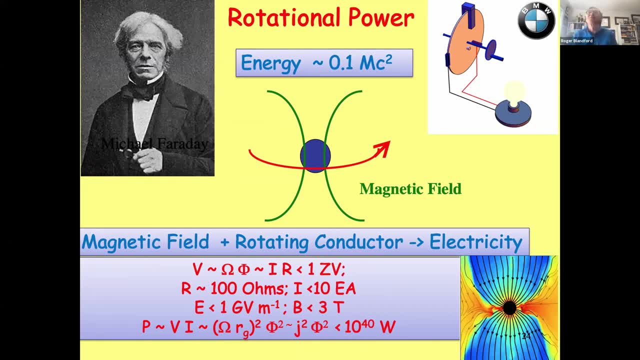 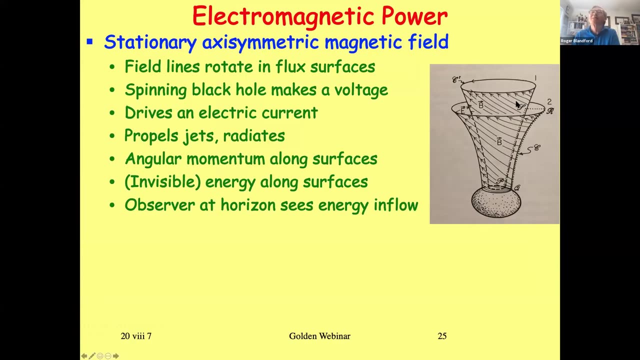 the three ingredients of magnetic field, mass and angular velocity, for those who know how to translate Greek into LaTeX. And then this pattern here, of course, is the pattern of the toroidal field. So if we go back to this one here, 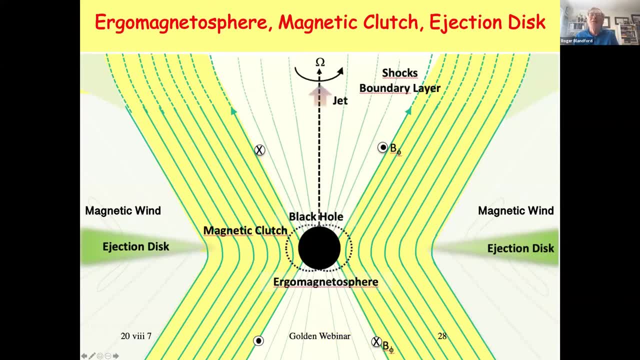 Now there are Nick Lovelace, and I and others have entertained the possibility that the magnetic field could have a quadrupolar geometry, but for reasons I don't really have time to go into here- both observational and theoretical- it looked like a good idea at the time. 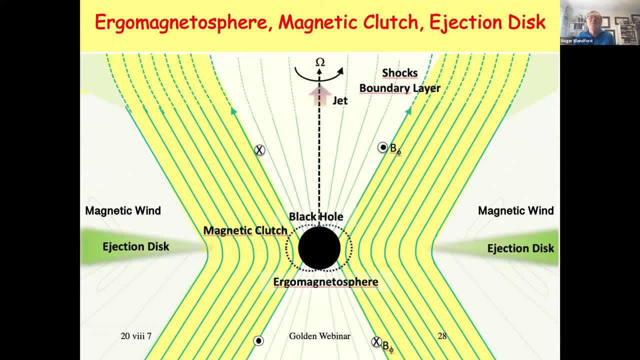 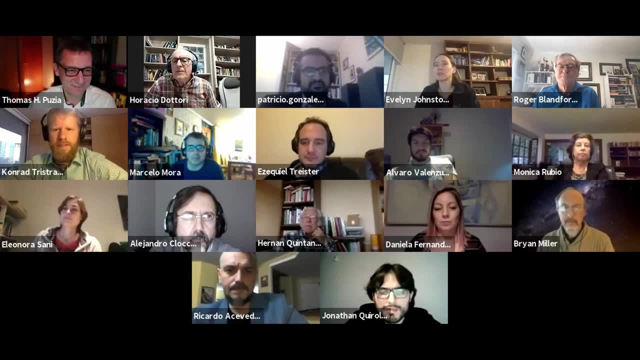 but I think it's not likely to be relevant now. All right, So we're going to continue with Eleonora. Yeah, thank you. So the question is still related to the mechanisms, but trigger a jet because anyhow we can observe relativistic jet. 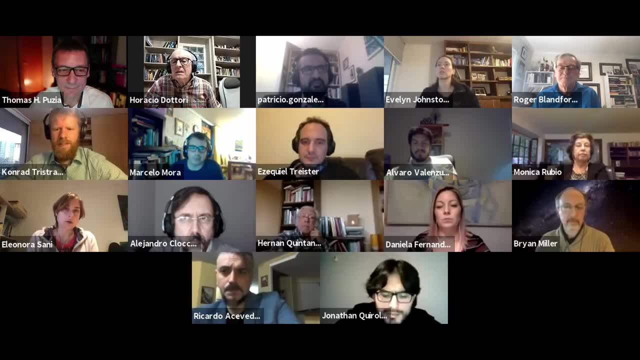 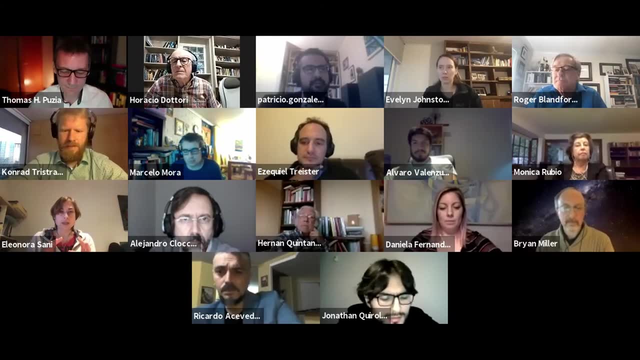 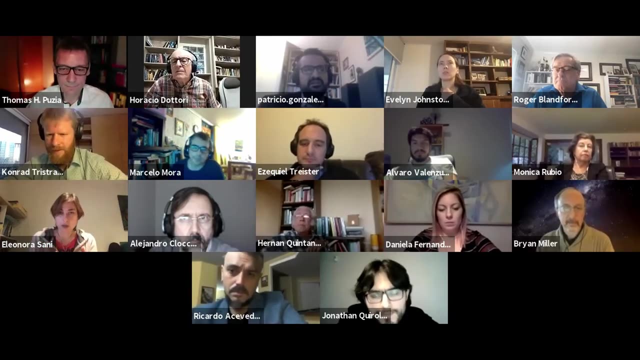 in a fraction of active galactic nuclei, a relatively small fraction. So why this? It depends, So it's a matter of just coincidence, because of the conditions, the inner conditions of the environment surrounding the black hole, the conditions of the magnetic fields. 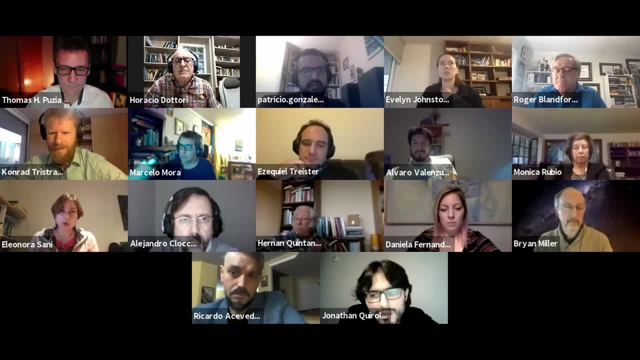 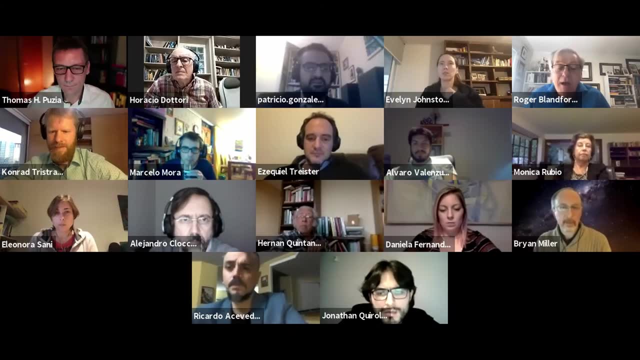 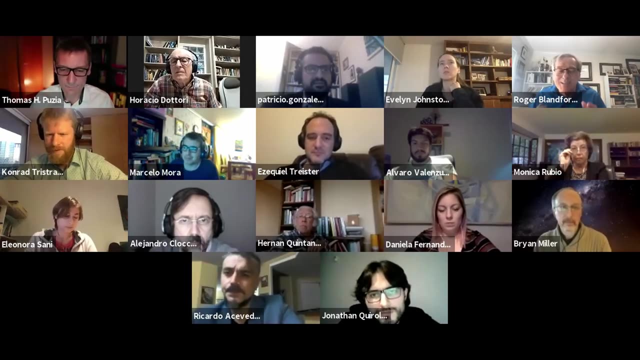 and so on and so forth, Or there is also an evolutionary component of these systems. Okay, thanks, Yeah again, I think that is a large part. The answer is, as they say nowadays, yes, in the sense that both of those are important. 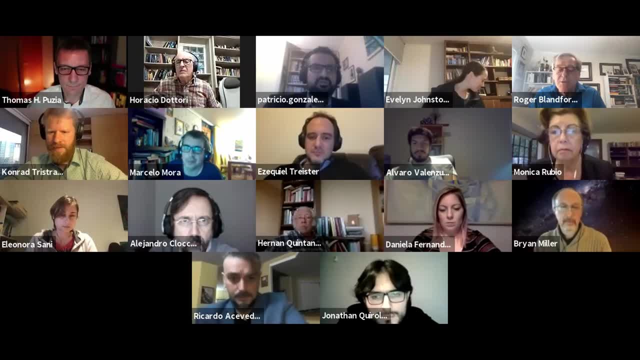 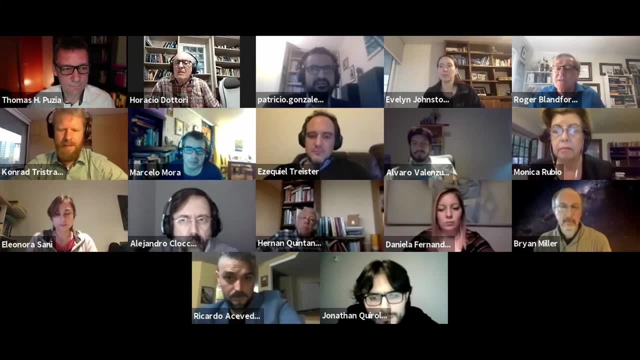 Not every black hole makes giant, powerful radio sources. That's pretty clear. This seems to be the province of the massive black hole and the centers of giant elliptical galaxies. Now, there are one or two exceptions to this, but that's almost all the really big, powerful ones. 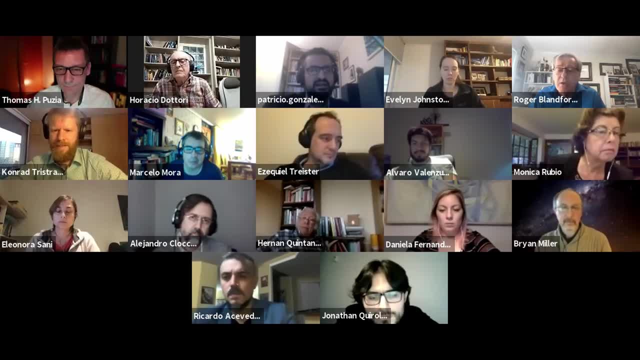 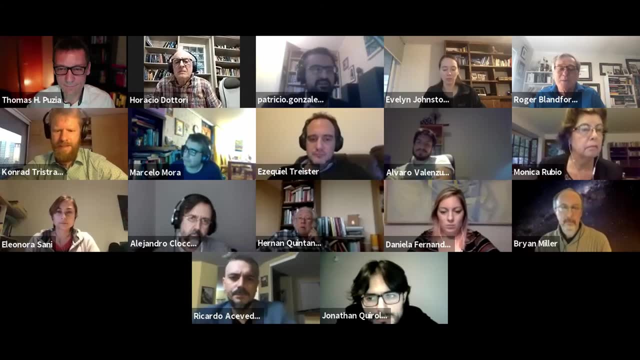 But low-power jets are quite common. I showed you the image from Meerkat with a billion of these things on the sky And you could say there's some. you know, there's the Fermi bubbles and other sort of evidence of bipolarity. 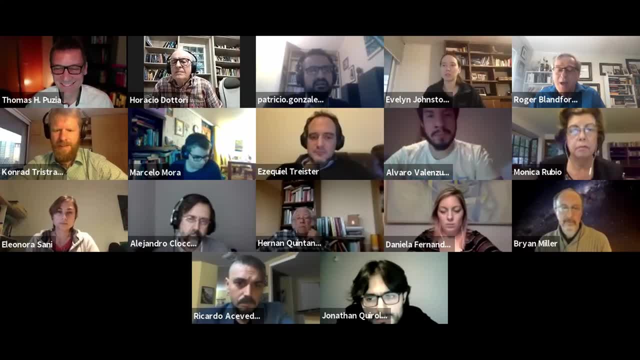 in our galaxy's black hole And that would not if that were at the Hubble distance. that would not make the cut for Meerkat by a factor of about a thousand. So it probably all AGS, all galaxies, at some level. 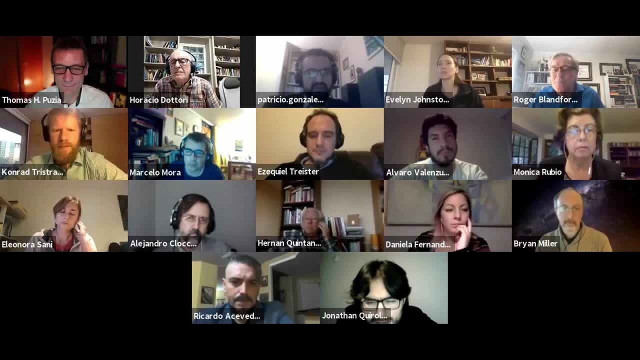 have some black hole near their center, and all of them probably make some bipolar activity, And so it's all a question of degree. Now what happens in a particular source? Let's take M87.. You may think it's a very you know. 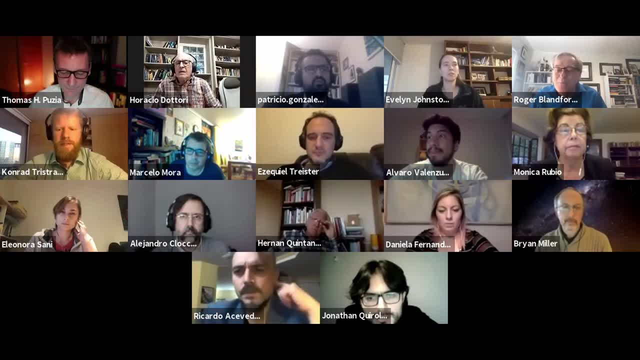 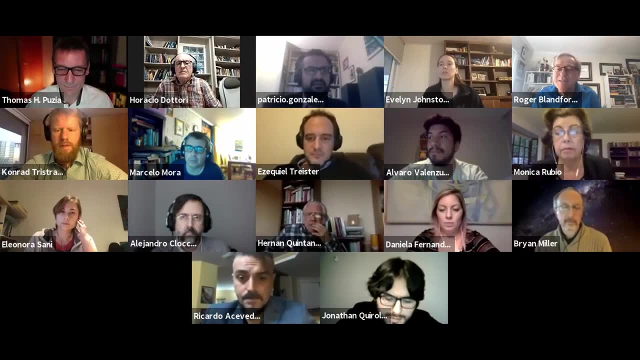 it was an early radio source. It was a great, powerful, wonderful discovery. From the- you know, the quasar perspective, it is truly pathetic. It is a very low-power source for a six billion solar mass black hole. There's almost, you know. 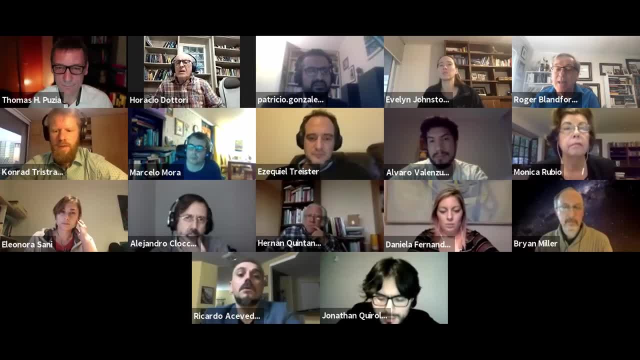 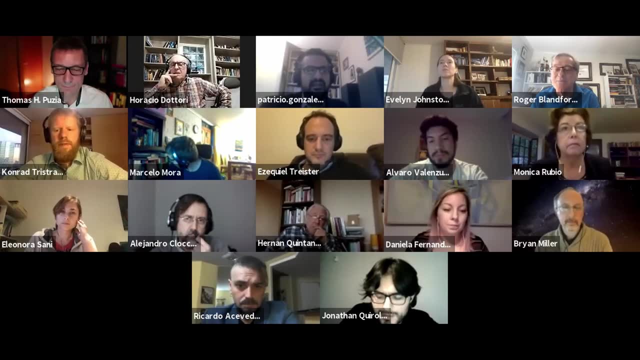 five orders of magnitude less than it could have been in its heyday. It would have been as bright as Vega in the sky. Our ancestors, if they were around at that time- and I doubt they were- would have been navigating by it. 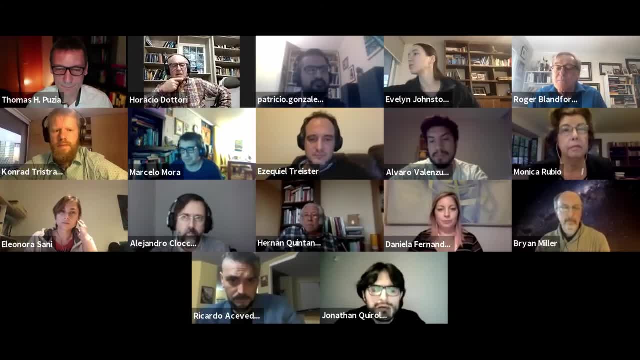 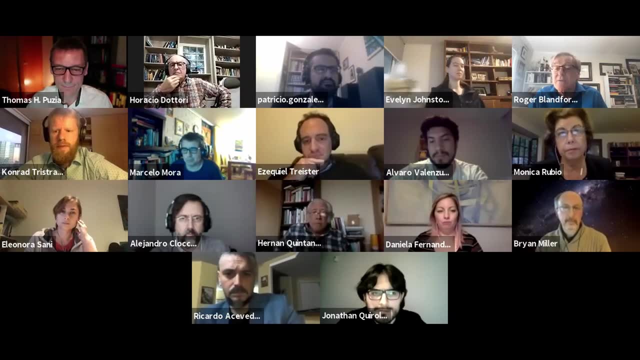 And it has enough, you know, and that's when it would have been providing essentially the heating for the major heating for the cluster gas and the Virgo cluster. So, and its behavior and how it operates and how it radiated and so on. 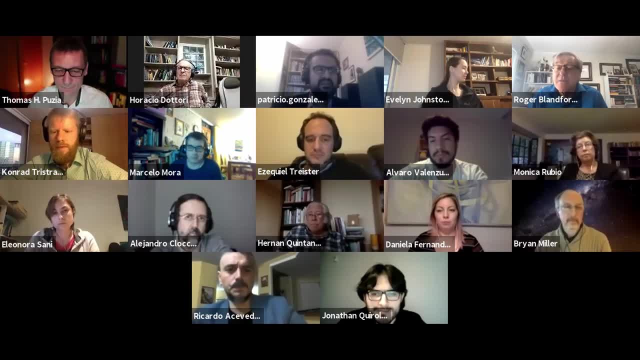 would be quite different in that mode and that phase than it is today, when it's a very has a very low rate of mass supply, And I would claim that the mass that's actually getting into the center is, you know, three, four, five, six. 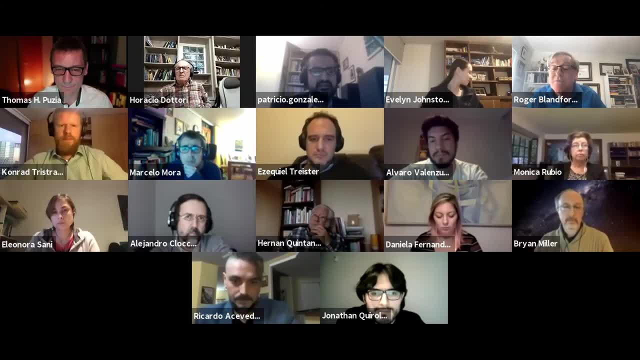 orders of magnitude smaller than that's what's actually supplied at larger radius. I mean, some gas is always going to get in. It's not a, it doesn't need excluding, and plasma is very slippery stuff, So it's always going to get in. 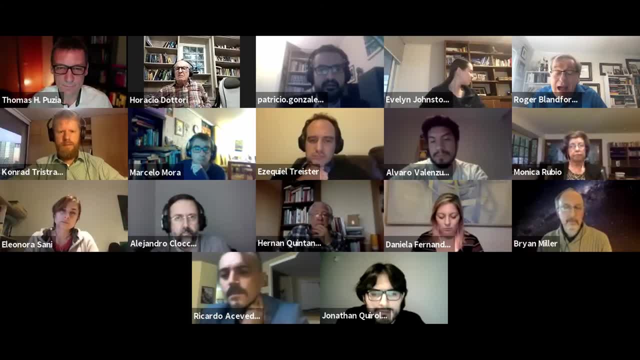 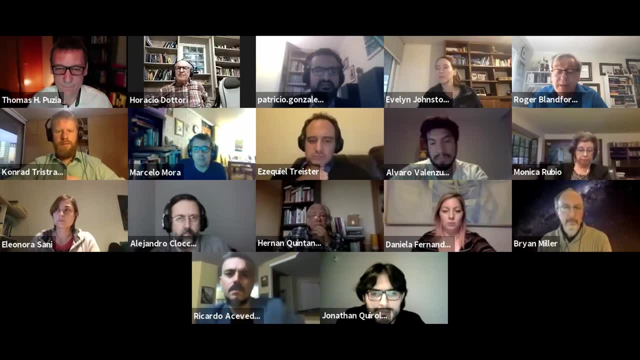 But the contention is that in the case of M87- now it was- it's expelling most of the gas that's being offered to it, Whereas in heyday, when it was accreting at the so-called Eddington rate, it was. 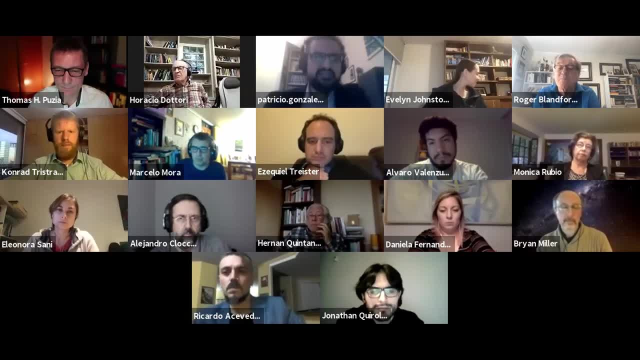 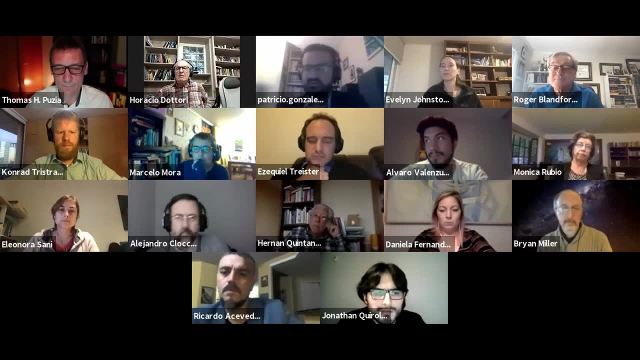 it was accepting most of that gas, taking its binding energy, making prodigiously powerful ultraviolet and optical source from the accretion disc and so on. And there's, you know, there's a, there's a life cycle Spinning up a black hole. happens relatively fast, compared with growing it, because you've got angular momentum from gas at large distances, So it can happen relatively fast. If I can continue, Imagine something like M87 having gone a hundred times through its cycle, Sure, Concerning the spin. 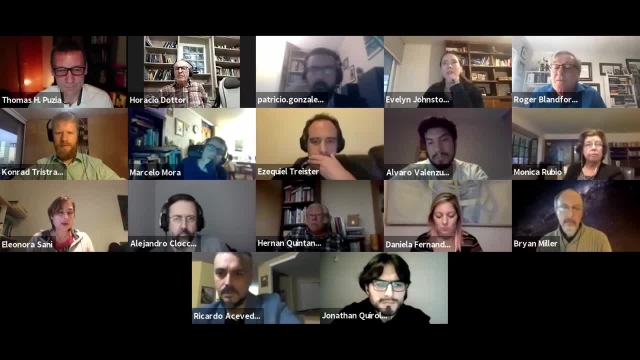 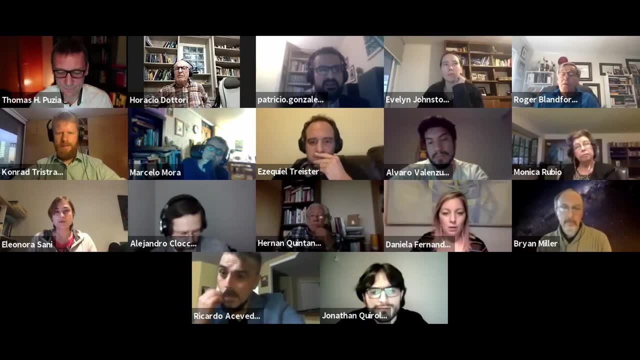 do you think we are close to being able to measure the spin of a black hole in a statistical, in statistical samples, And in case? with which kind of CET? Okay, Yeah, I, I didn't. I actually took these slides out. 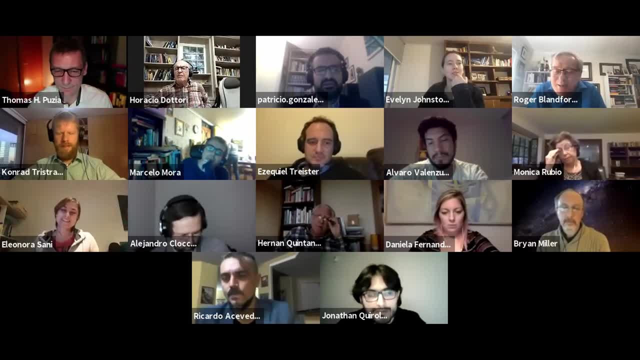 but I'm so, I'm so glad for asking this question. We do have measurements- not just of the mass- from using Kepler's. we do have measurements of the spin, And some of them are a little dodgy in my view. but 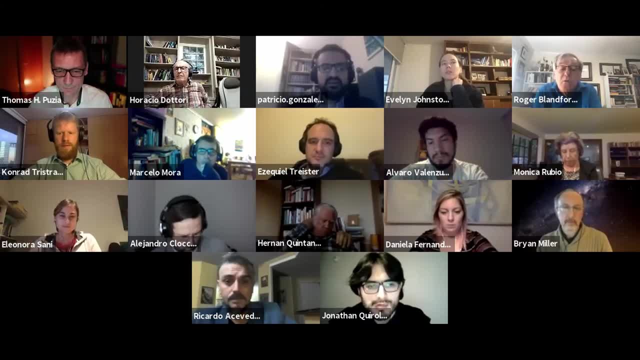 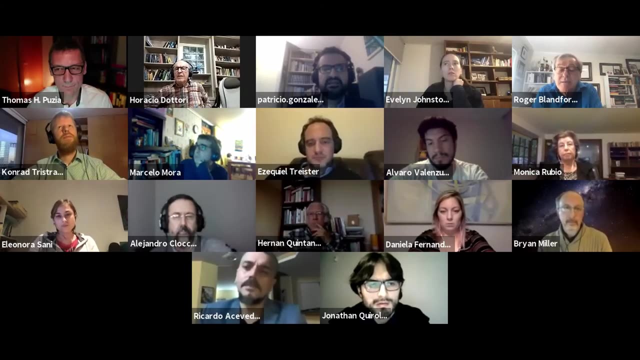 but there are some, but there are ones that are looking very good And one of them is to look at the accretion discs and look at the, particularly the ion line seen at x-ray wavelengths, And that has a thickness which is believed to be. 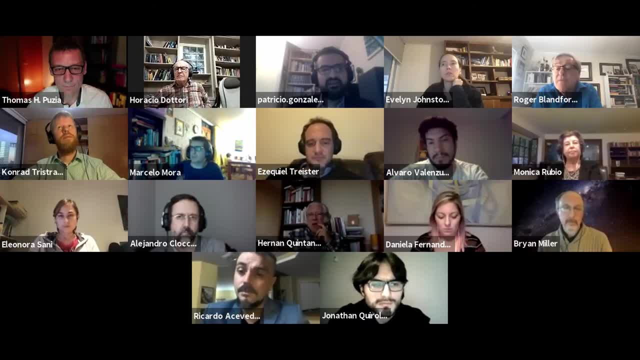 and modeled to be a measure of the spin of the black hole. And to cut this, this observational story short, what you have is evidence that many, not all, but many of these sources are spinning. not just spinning, but spinning almost as fast as they can. 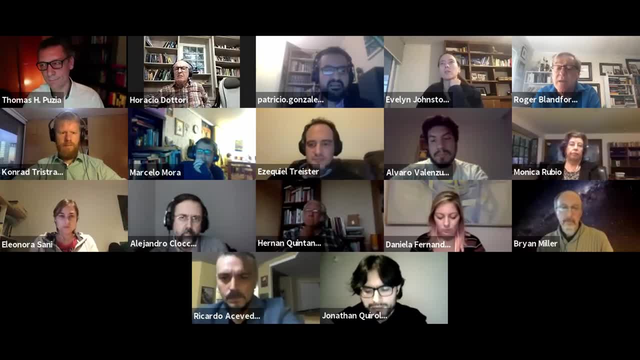 And that's the observational evidence. And you know it looked like a good story when it was first told from the x-ray observations. But as we've looked in more and more detail with x-ray telescopes you can see lots of features. 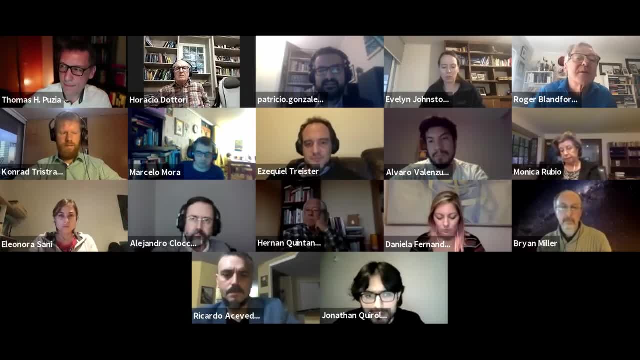 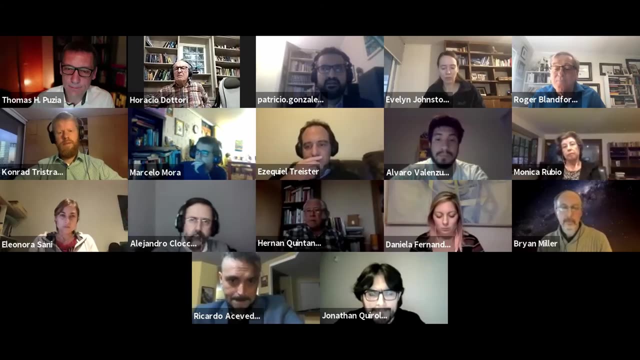 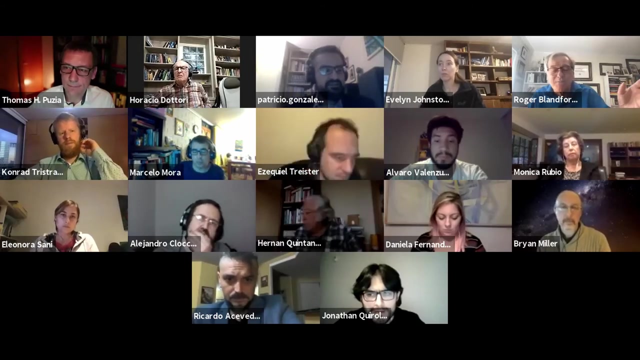 that are interpretable as lots of features that are interpretable in terms of the rays of light going close to the black hole, for example, time dependent behavior, so-called reverberation mapping, where you see a flash of x-ray radiation illuminating the accretion disk. 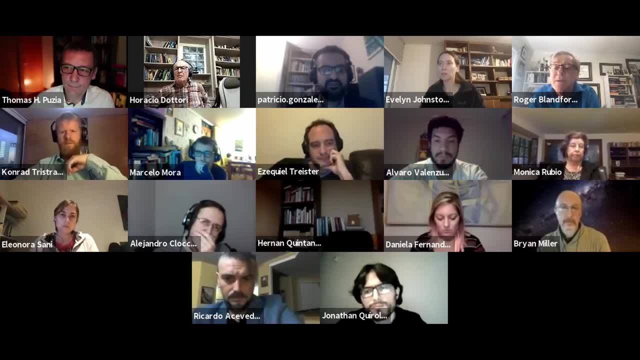 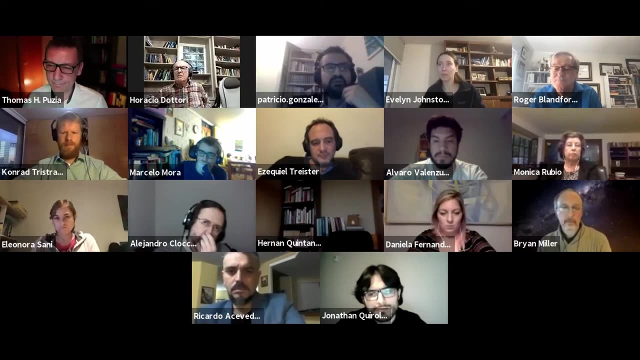 and then you see the response at a delayed time. This sort of sort of second order business seems to be fitting into the story, And so I trust. I was always quite trustful, but I'm even more trustful now that they're measuring very high spins. 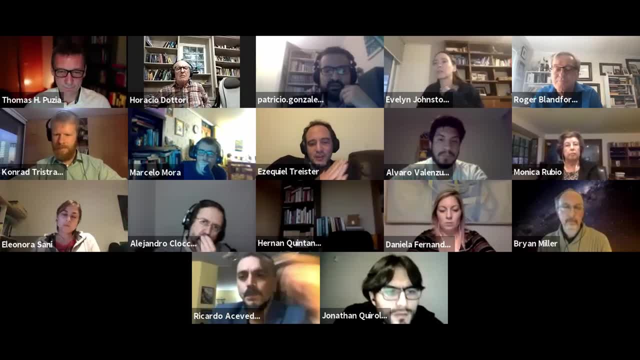 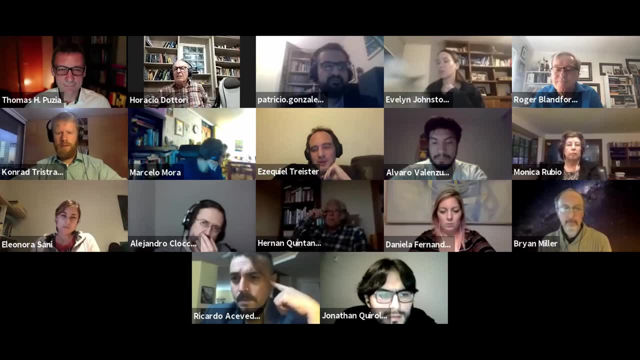 Ezequiel has a follow up question. Yes, Well, thank you very much. Well, thank you very much, Roger, for the magnificent talk And also, yes, what I want to ask is basically a follow up on this. 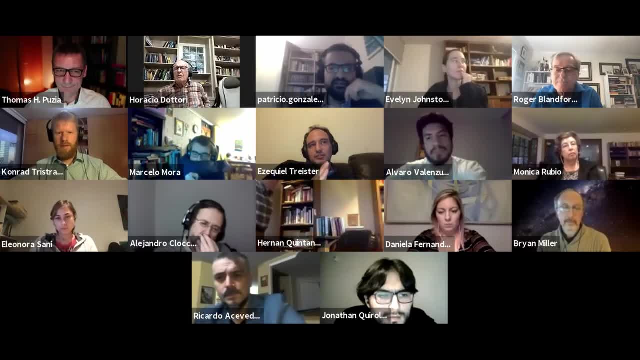 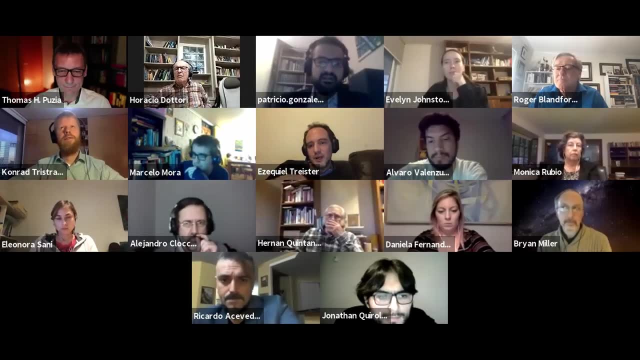 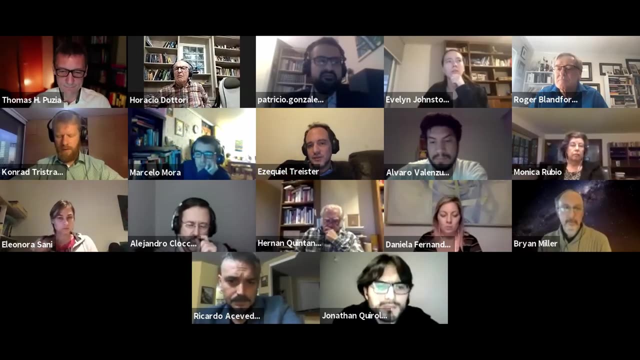 Also statistically. I think some sort of the sultan argument. basically, when you integrate the accretion on an AGN and turn it into a black hole mass, you require a fairly high efficiency. Typical value is about 10%, but more recent models. 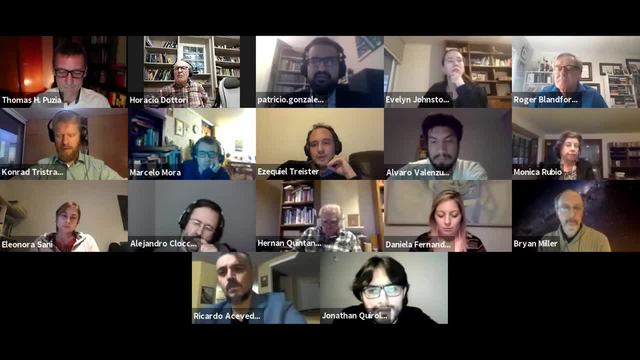 can take it up to about 30% or so, Which will require statistically, as you say, very high spins on average. So it means that if that's the case, then it seems like a spinning black hole is basically present in most AGNs. 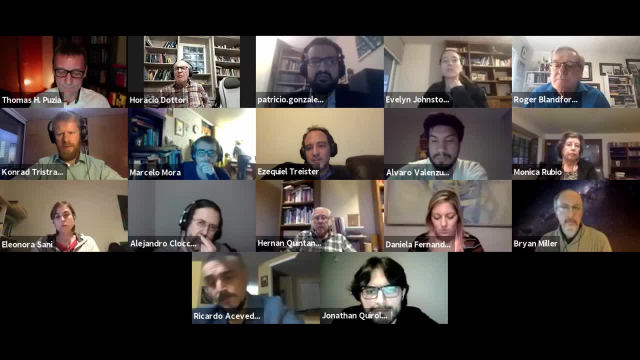 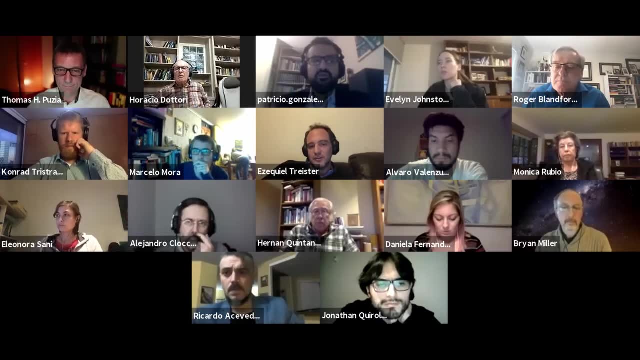 or more, or the most powerful AGNs, And yet only few of these sources have powerful jets, And so it seems like the key difference is the presence of magnetic fields, And in that case, my question is: what do you think will be the relevant? 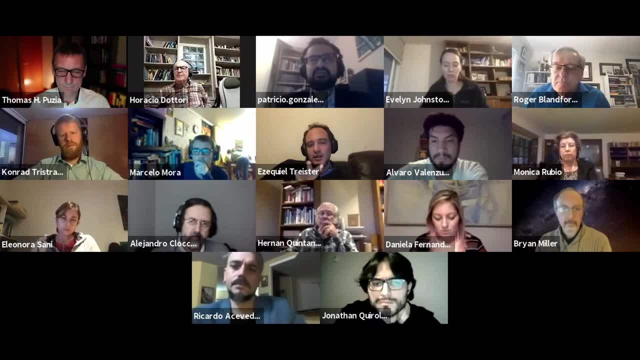 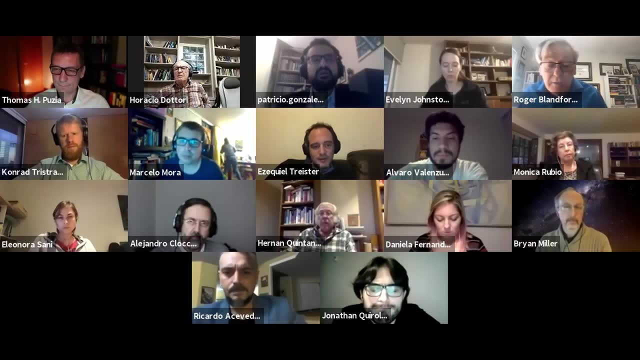 physical parameters in determining whether a magnetic field is present or not. What should we look for, Okay? Well, thank you very much, Ezequiel, And I think again, that's a very good point. Let me just back up a little bit. 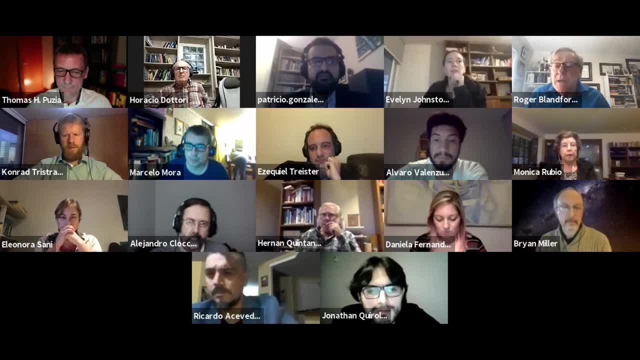 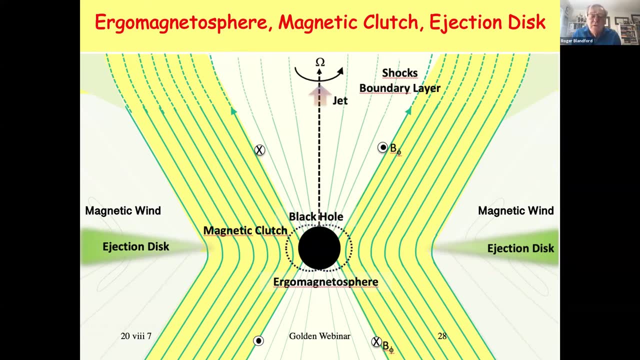 just to explain something because I think it's important. And you sort of alluded to the so-called sultan argument And this was an argument that was a very important argument that was given by Andreas Soltan 30 years ago And basically, 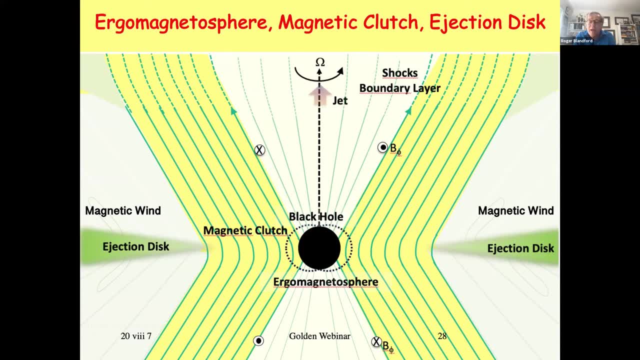 he did something very, very simple. He said: let's just look at the amount of radiant light- mostly ultraviolet- that quasars over the whole sky make and what's the energy density associated with it. Then let's take the equivalent energy density. 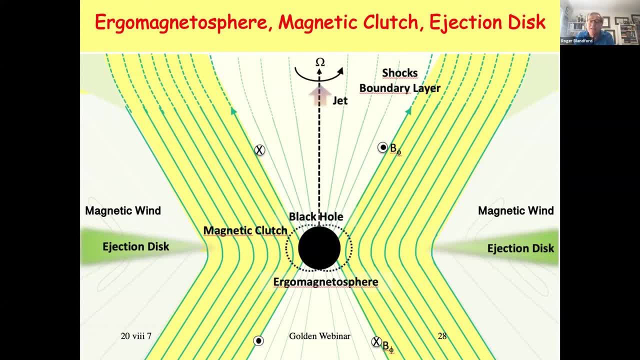 or mass density, but it was mc squared, so it's energy density of black holes. So let's compare those two. And he found that, independent of the tortured histories of these black holes. if you say that some fraction of the mass energy 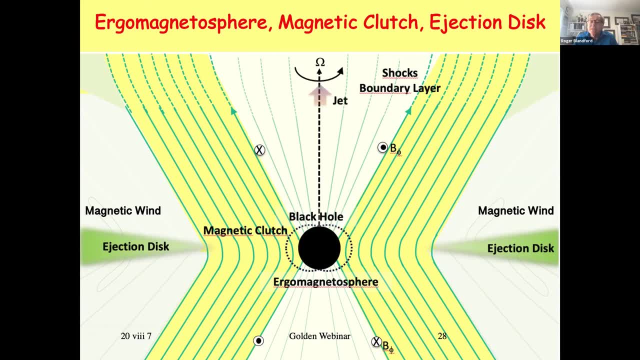 of a black hole, spinning or not, goes into radiant energy. the efficiency has to be pretty high. Now you can. it becomes a sort of messy observational astronomy business doing the details here and volumetric corrections and all of that stuff. But some people say 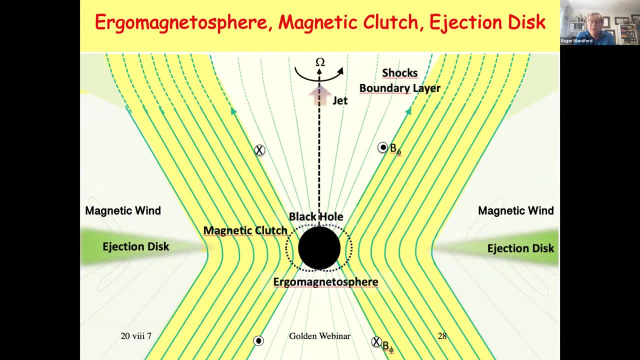 it's got to be 30% efficient. Some people say you can make do with 5% efficient, but it's still pretty high. So you're not allowed the luxury of growing black holes invisibly. You want those photons out, just to account. 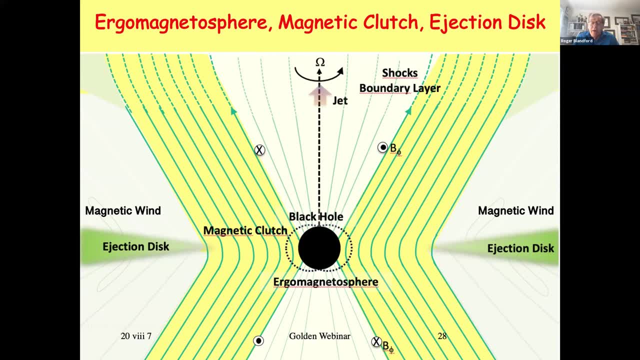 for what you observe as an astronomer. Now some people have gone on to say: well, let's take the ISCO arguments and take the spin energy of modestly rotating, rotating black hole and you're going to get 10% out. 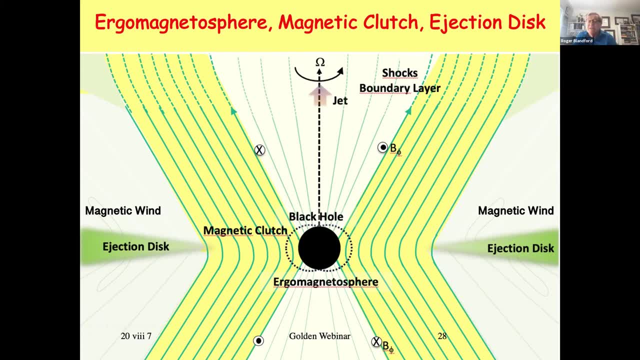 I need more energy than that. Therefore, I have to tap the spin energy. Some people have actually said that I'm not sure that's. I believe that's going on, but I'm not sure that's necessary. quantitatively, You might say well. 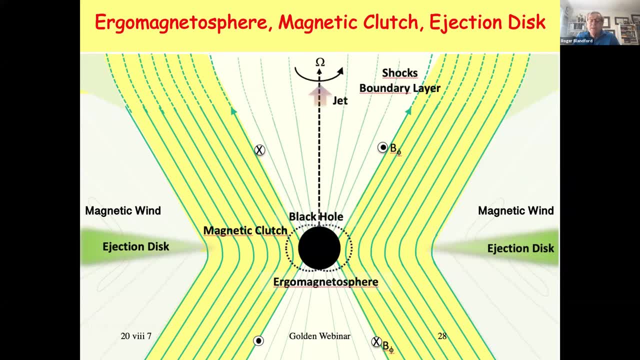 does every spinning black hole automatically radiate by this mode? And the answer is, observationally no. There are radio-quiet quasars and some of them, and the reciever galaxies and so on, are spinning rapidly and not making jets. 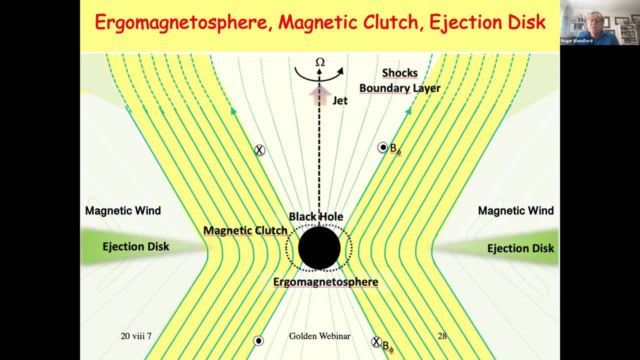 So there's some other factors in there that are telling an accreting spinning black hole whether or not to make a jet. It may have something to do with history. My guess it has to do probably with cycling of gas in the 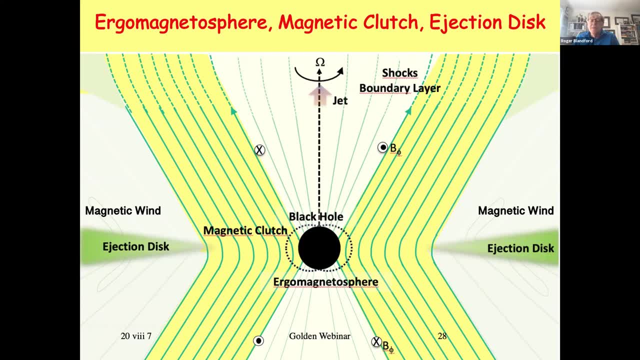 in the accretion disk. I think one of the things that I'm very impressed by is the association of jet, of the powerful radio source, with elliptical galaxies, And for me, I might you know, I actually wrote about about this in an annual article. 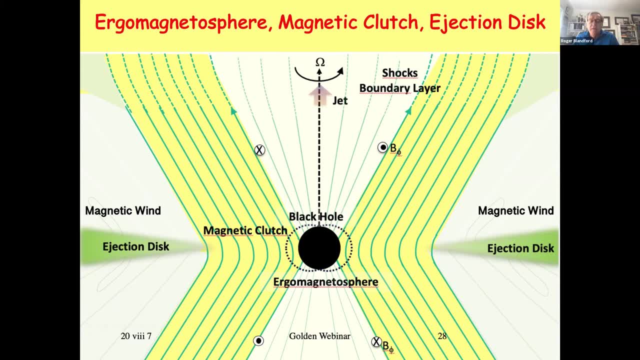 with Tony Redhead and Dave Meyer, And there the thought is that in the in the elliptical light galaxies the gas is being supplied at all latitudes. It's falling in essentially from some circumgalactic flow And that provides a much better. 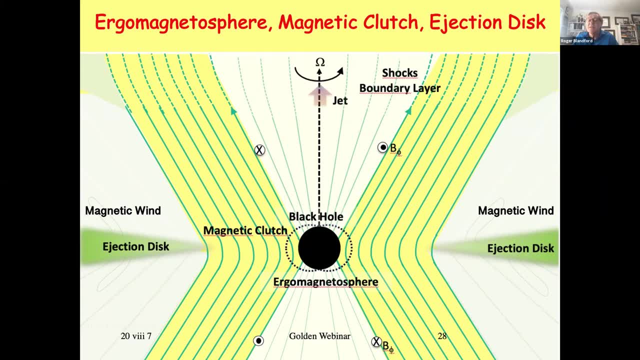 confinement of the magnetic field than what happens in a disk galaxy. And in a disk galaxy the gas only comes in in the equatorial plane, And I think it's easier for the magnetic flux to escape that hole in the middle, as it were. 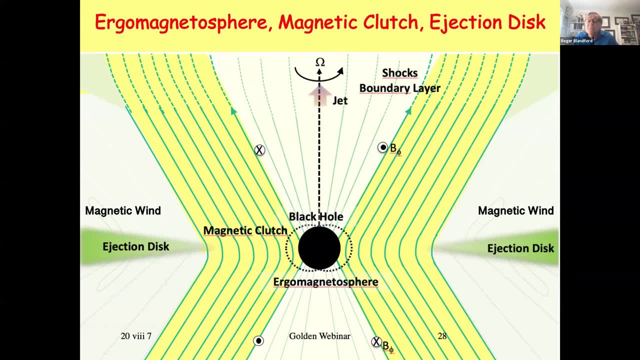 when, when, when there's a disk inflow associated with the spiral galaxy, say, than there is in accretion at all latitudes in an elliptical galaxy. So that's my current favorite additional factor, or switch or whatever, for answering that. 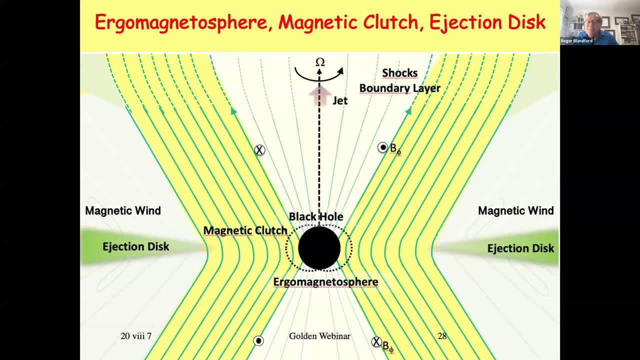 But but it you know, this is a time of rapid discovery and Webb is going to tell us stuff. I mean, Webb, James Webb Telescope is going to tell us things And we'll have a very interesting conversation again and I hope, in a few years' time. 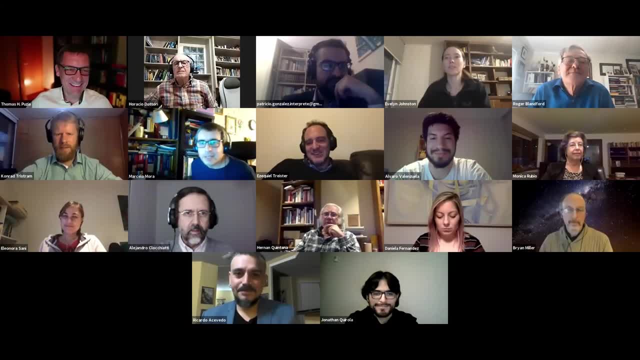 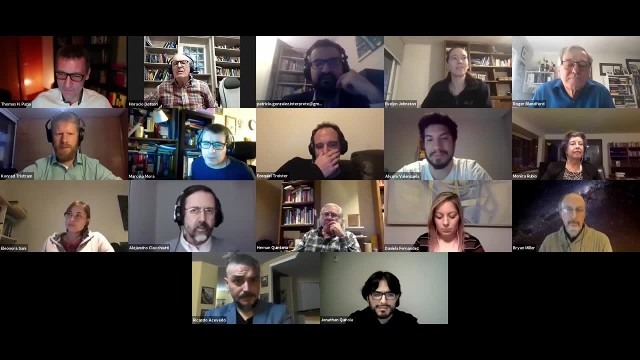 about this topic. So it's me. I have two questions, one from the audience, Natalia Moreira. So she's asking: how do I discover the black hole? has an electric charge? And, following that question, what happened with the magnetic field? 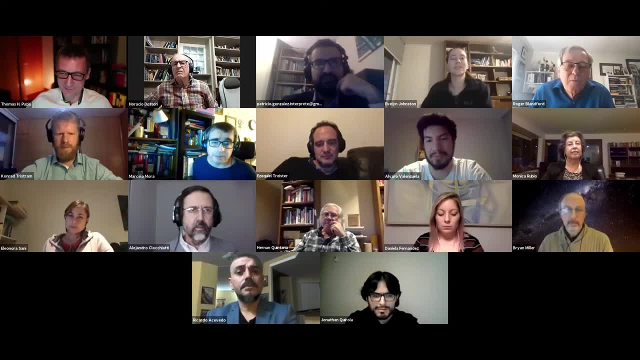 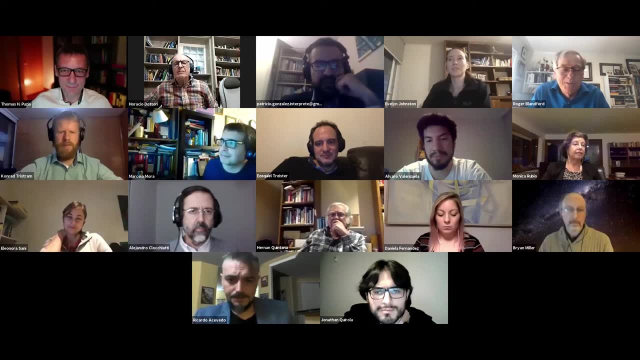 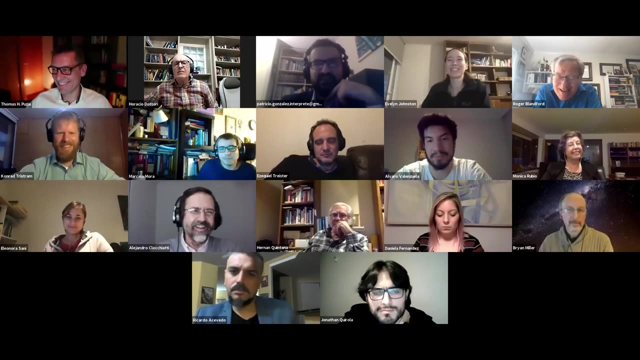 once it's inside the black hole or once it's across the event horizon. Okay, Lovely questions. Okay, Let me again. these questions are artfully addressing slides that I took out of out of the presentation, So thank you very much. There. Roy Kerr and others actually discovered in the 1960s an additional generalization of the Kerr solution for a spinning black hole, And it's one that had charge associated with it and its own magnetic field associated with charge inside the black hole. 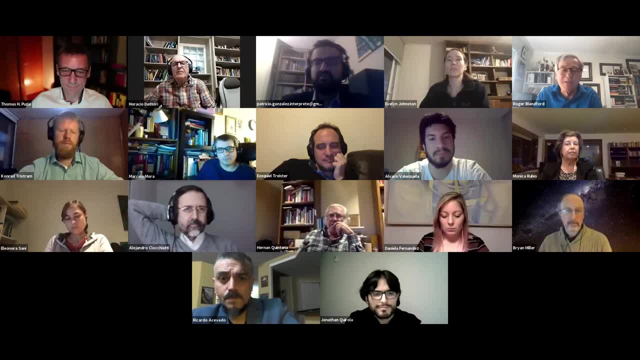 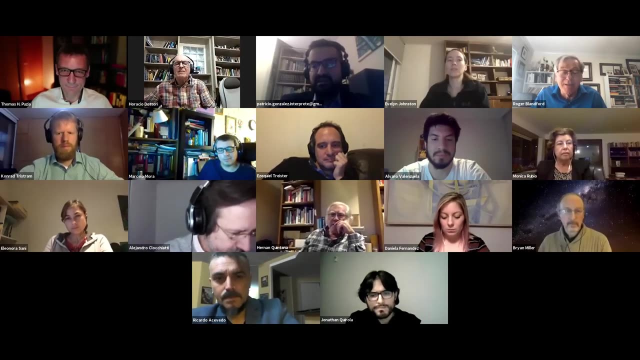 This is a wonderful solution. Like many of these constructs, it is a playground for the febrile imaginations of theoretical physicists And they have gone off to you know, perform wonderful, get wonderful understanding of the interior geometry of these black holes. 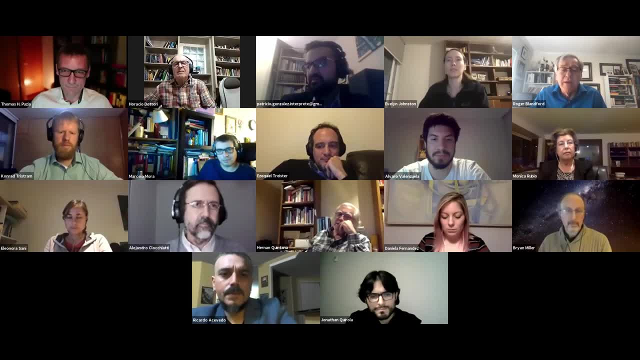 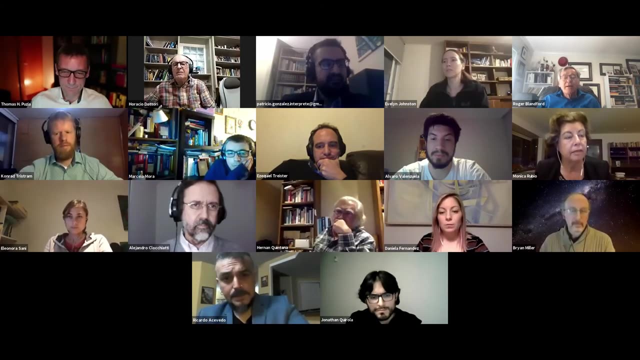 However, I believe quite firmly that they're a bust in astronomy, Because what happens is, if you have a gravitationally significant charge- not just a tiny one, but a gravitationally significant charge- in a stellar mass or larger black hole, then it will immediately. 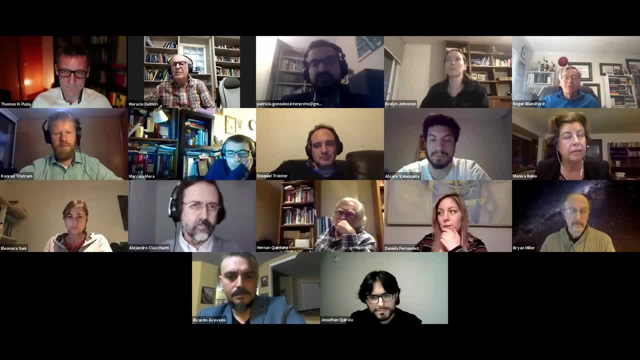 discharge. It can make electrons and positron pairs, just like lightning on the Earth, if you like, And that will immediately discharge itself. You can't build up that amount of charge anymore. You can do that on the surface of the Earth underneath a cumulus cloud. 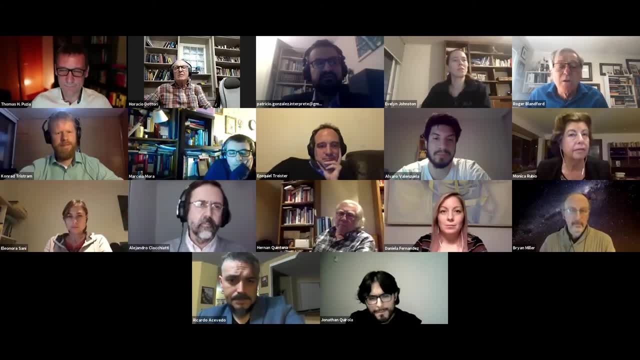 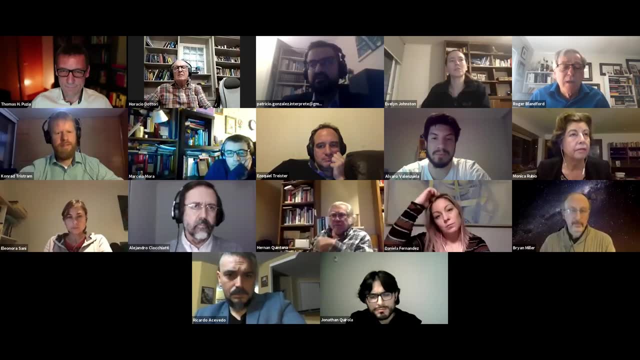 And so I think that they're not of great interest for practical astronomical observation, but they are terribly important. Now, the corollary of that is that when we talk about magnetic field lines threading the horizon of the black hole- and this is well defined- 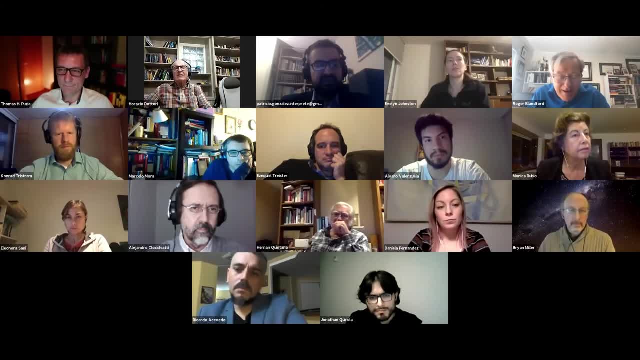 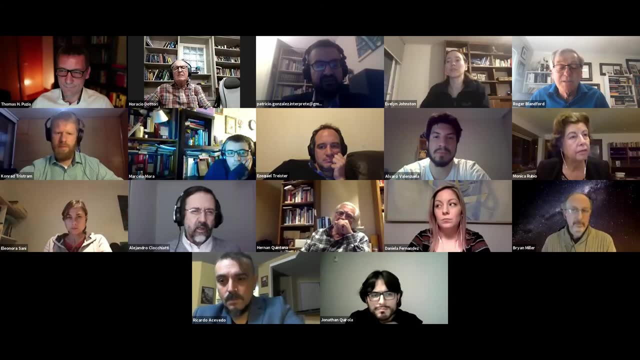 mathematically, These are magnetic field lines. We can trace them. They head towards the horizon, And we can in fact go behind the horizon and see what's going on there. Then this is all sort of well defined using so-called Maxwell's equations. 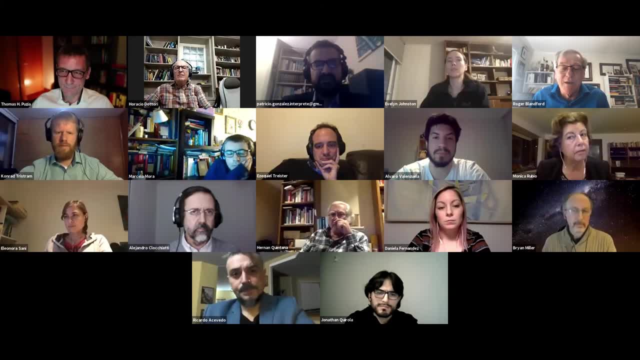 and Einstein's general relativity. You can do all that stuff. That field requires there to be a current and the electrical current outside the horizon, that is the source of the magnetic field. Okay, So it does require the disk, It does require the current. 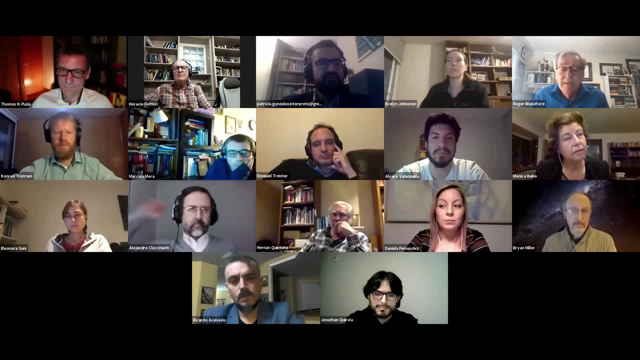 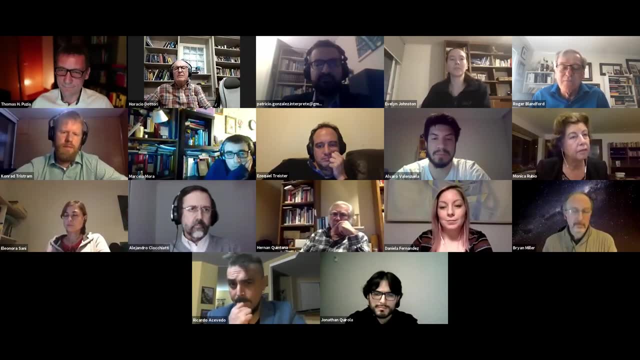 in the disk to hold the field in place. So that is absolutely required. Now, if you ask, well, what's going on into the magnetic field within the horizon? And that's the question I think was asked And I wasn't actually going. 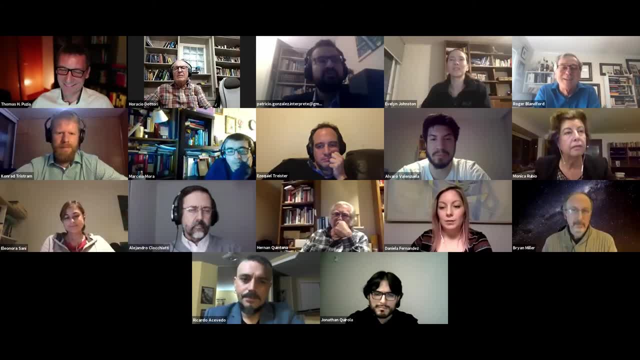 to talk about this, but since you've done it, it was wonderful and one of the things. actually, Romans and I were worried about this very, very point And I kept on using the word dissipation And I said: we've got these flows. 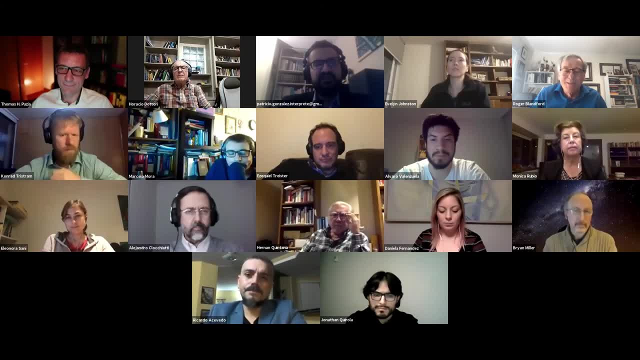 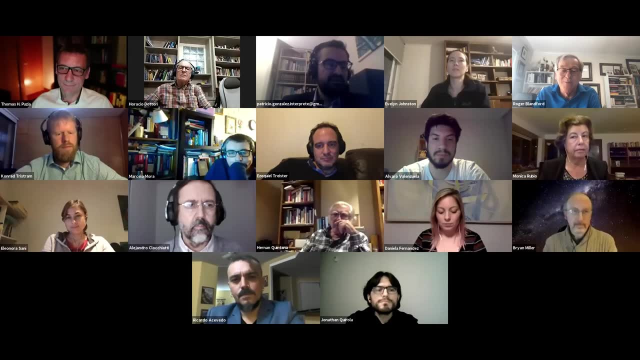 of differentially rotating gas outside the horizon. that ought to be dissipative, It ought to heat very easily And you have to work quite hard to prevent it from to imagine it's not going to radiate, So it's going to radiate very well. 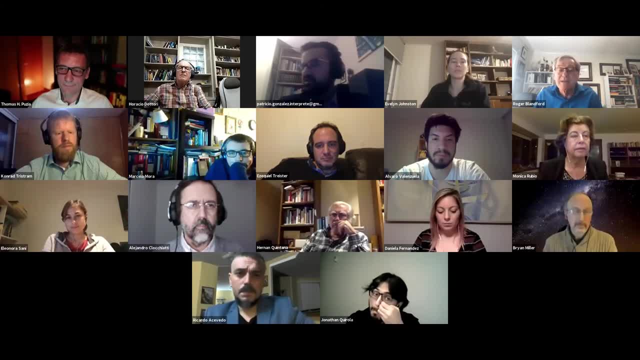 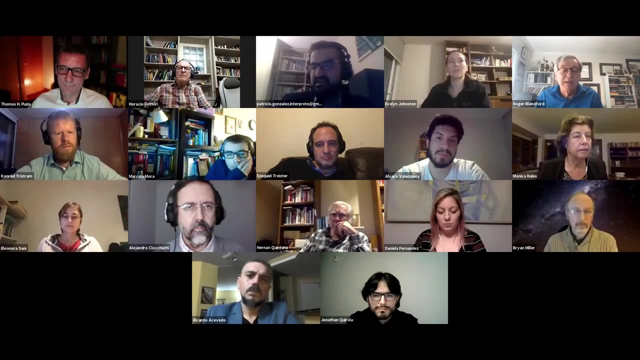 What happens inside the magnetic field to magnetic field lines inside the horizon. Well, it turns out, you can trace the magnetic field lines through a perfectly smooth geometry inside the horizon And you can follow magnetic field lines with electromagnetic energy, essentially locally invisible, if you like. 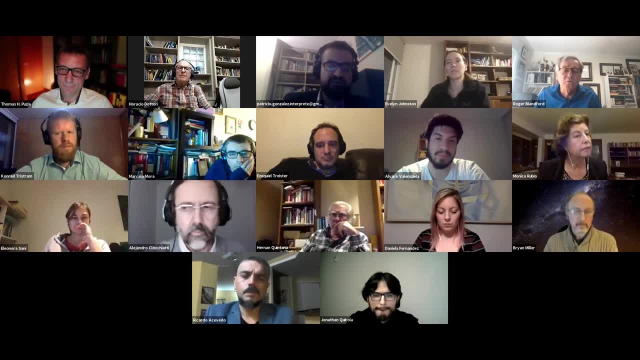 inside the horizon. You can do it as the thought experiment Before too long you get to a point, long before you get to essential singularity, when all of this must break down And there must be an enormous dissipation going on. 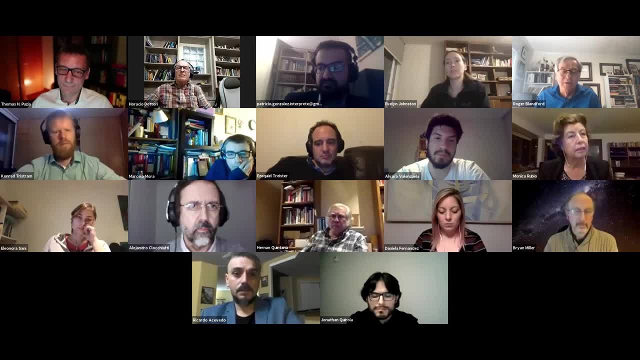 Now, black holes, I like to say, are very respectable because all of the dissipation happens behind the curtain. People have closed the curtain, That's the event horizon And so, yes, there's a lot of dissipation happening there. 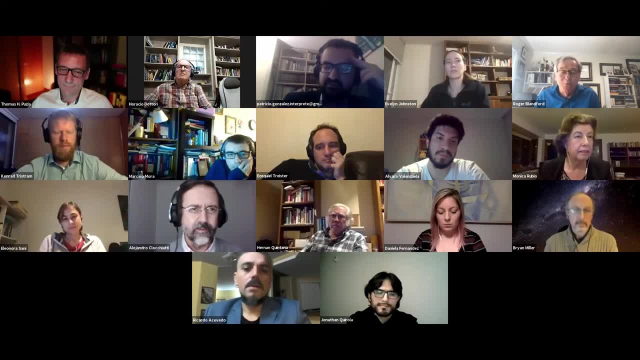 But that dissipation is not seen because all of the gamma rays and the X-rays and so on that are made by this dissipation behind the event horizon it's real but it's not visible because it doesn't get out through the horizon. 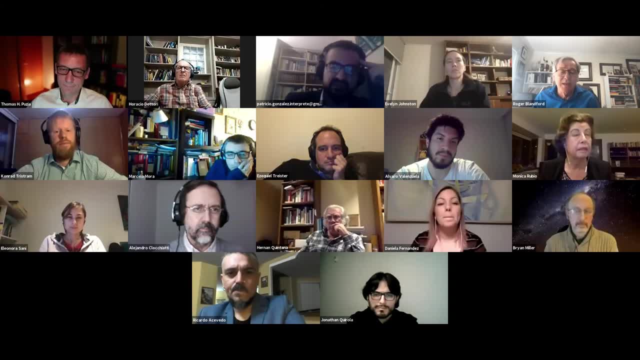 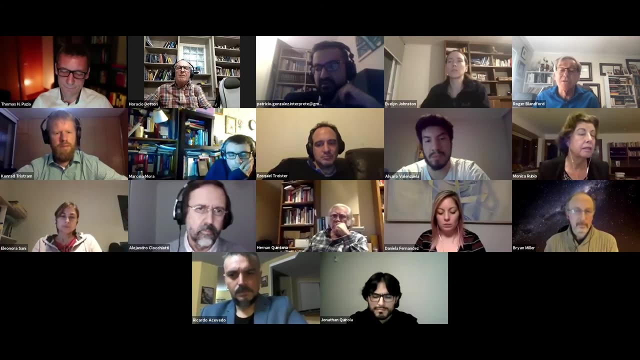 And if you want to think about this by this sort of electrical analog, we can think about this as the very simplest type of electrical circuit generated by the spinning black hole. That battery has a sizable internal resistance and it has a load that's comparable, that's essentially matched to it. 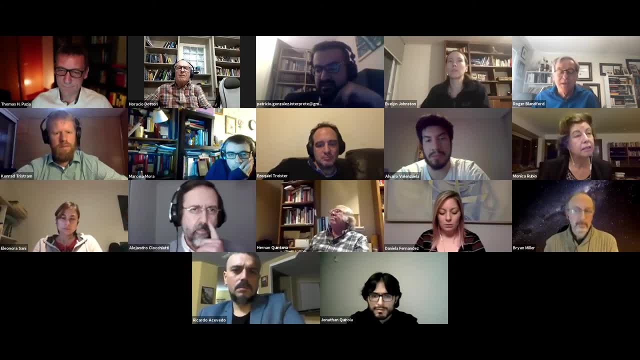 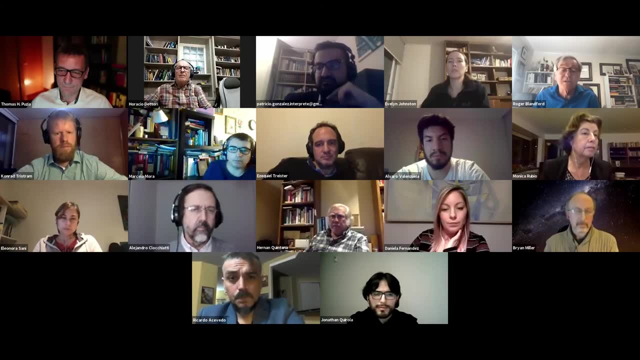 And so we have an electrical current. Some of this dissipation happens inside the horizon and increases the mass of the hole. That's an inefficiency- And some of it happens outside, making gamma rays and radio waves and all the rest of it, ultimately. 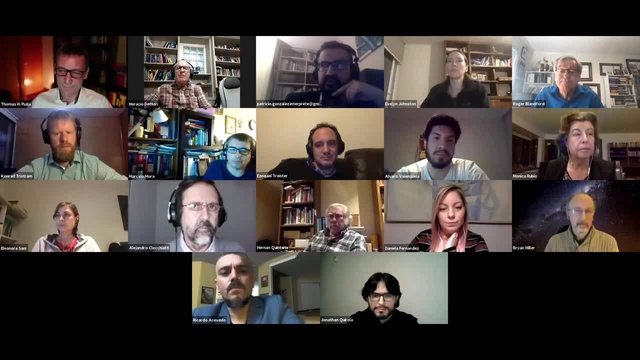 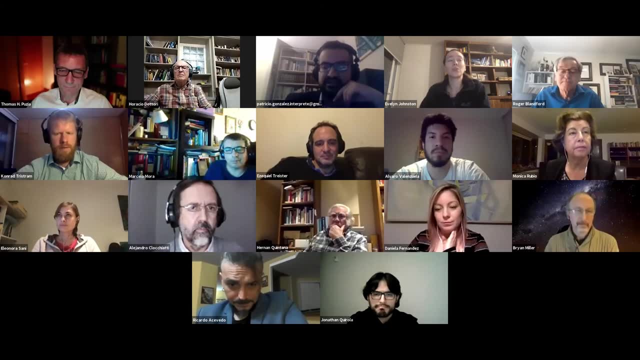 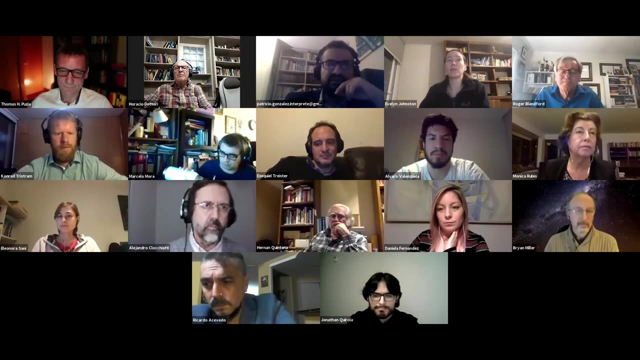 and outflows, And then probably cosmic rays too. OK, so I have a few questions from the audience. So the first one is from William Freights, who's asking: would it be possible to harness the powerful energy being released from these black holes? 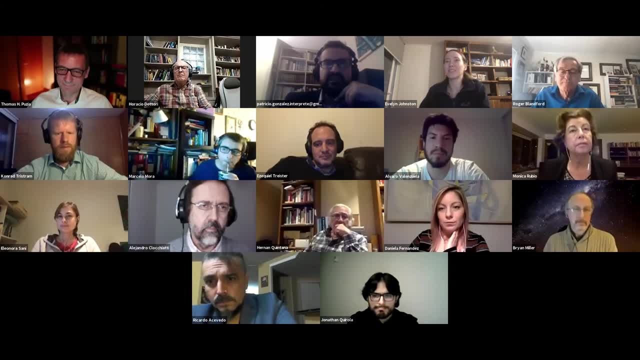 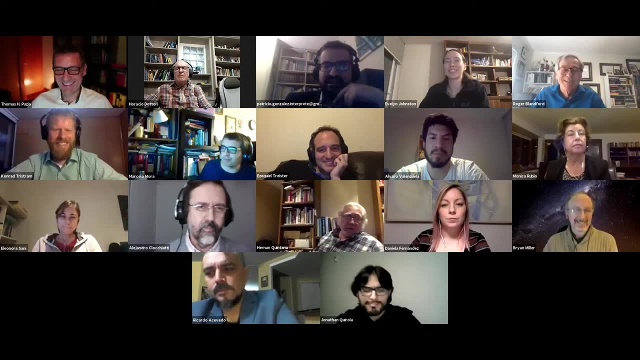 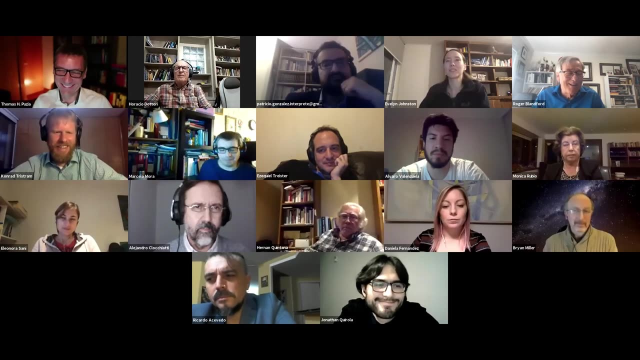 to develop more efficient space travel? Ah yes, Well, first catch your black hole, I think, is the answer to that question. I think we'd. I've had a few suggestions in the mail from time to time of using black holes for solving energy problems. 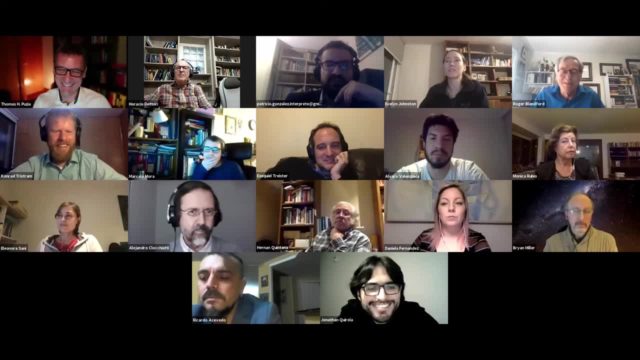 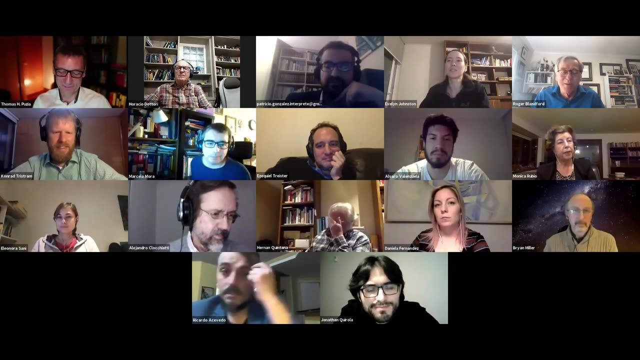 and all the rest of it Wonderful. but of course, making one is not easy, And so the answer is: a practical method? no, because we don't have one to hand, as it were, So we have to make do with lesser forms of propulsion. 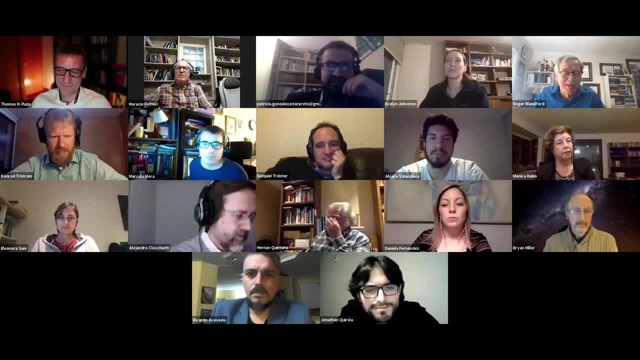 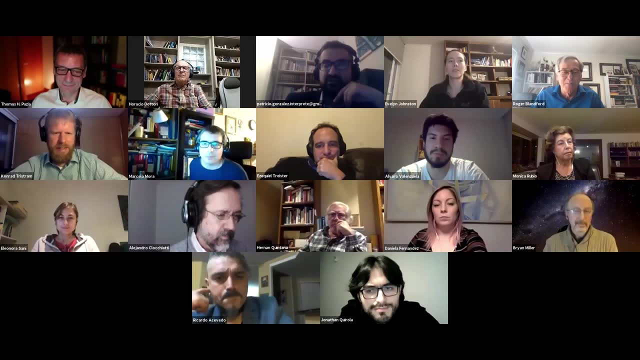 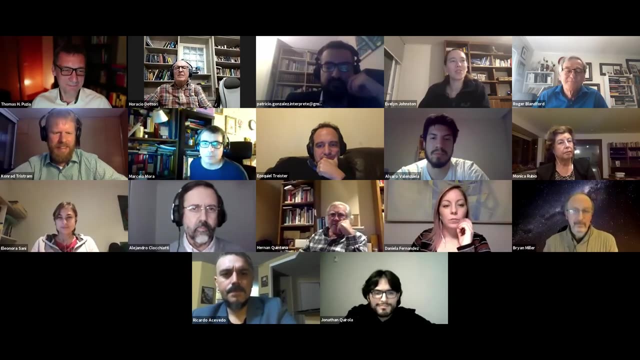 In fact ideas of using nuclear power with scotch for environmental impact. I have to believe the black hole environment backstate would be even more hazardous. We have another question from Jorge Cuadra. How can we distinguish whether the EHT image corresponds to the ergosphere? 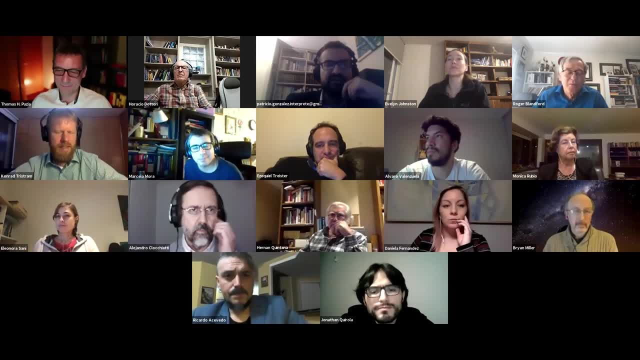 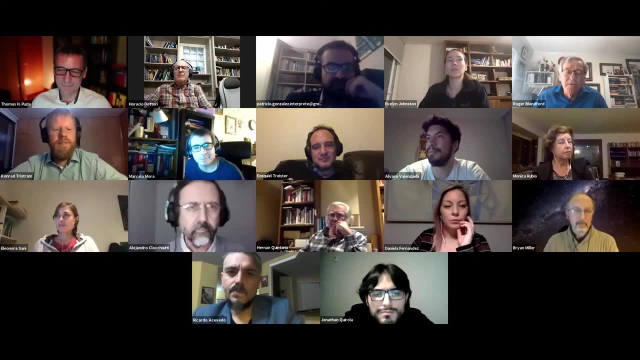 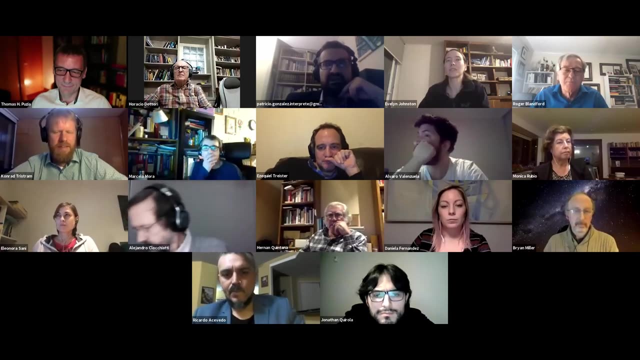 or the disk? Would the inferred black hole properties be different? Lovely question. The second answer is the black hole properties. no, I don't think, not seriously. I mean, you'll get some differences, but not much For me. 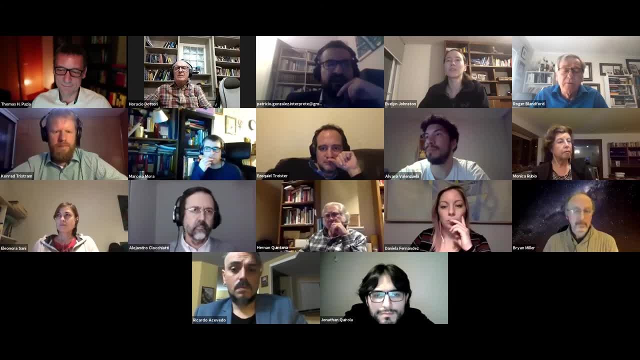 the difference is the polarization And when you, what you're looking at in the ergo magnetosphere interpretation is, you're looking at a current sheet without a lot of gas around, So there isn't an effect called Faraday rotation. that's operating. 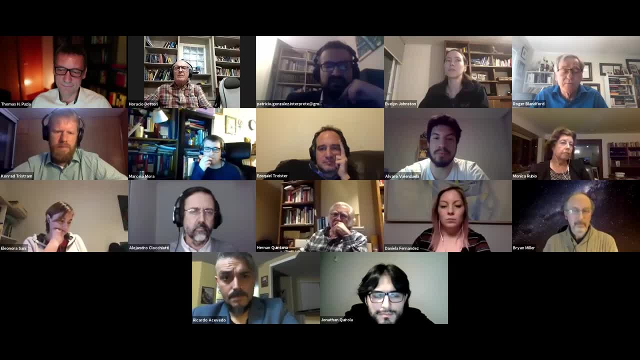 In the case of when you've got a thick torus. if you're looking through that torus as an appreciable amount of plasma, then then you'll get a lot of Faraday rotation, And so I don't quite know what the 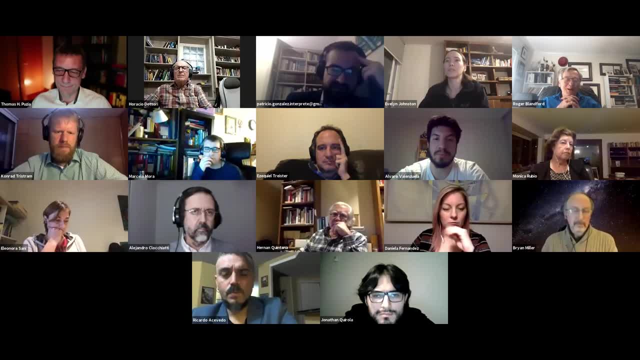 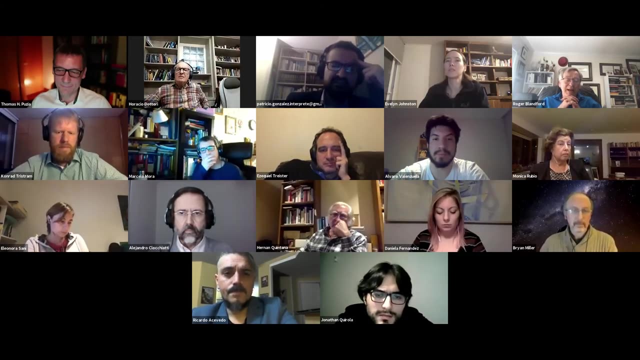 you know, I don't know what the EHT observations are, or indeed I don't quite understand what their simulations are showing, But naively I would have thought, with the sort of densities of gas and magnetic fields that one might expect, then there should be. 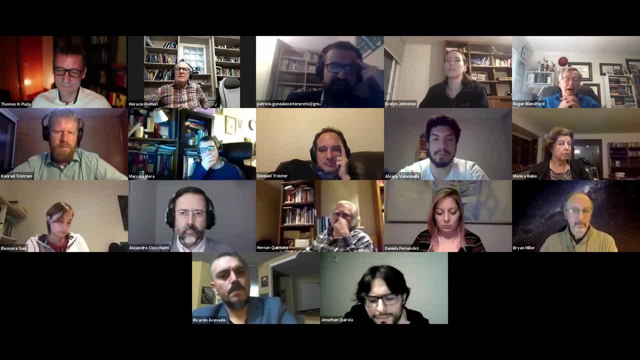 a lot of polarization. So for me, I think the prescriptive way of deciding between these two very different views- both of which you know could be right- is to is to think about the upcoming polarization observations. High resolution will help too. 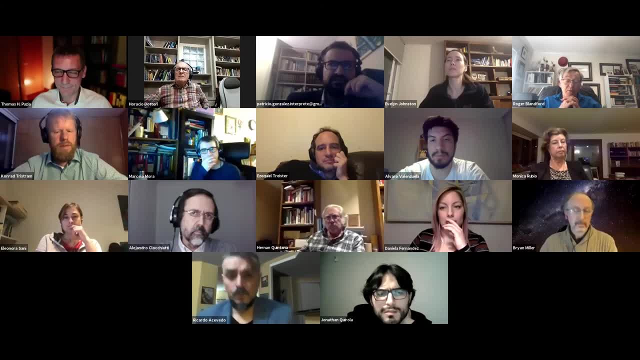 of course, if you get Greenland as a north-south baseline, then that will also, and you can go to 0.8 millimeters. I mean again, you're getting a significant improvement in resolution. So I see Jonathan has also got his hand up. 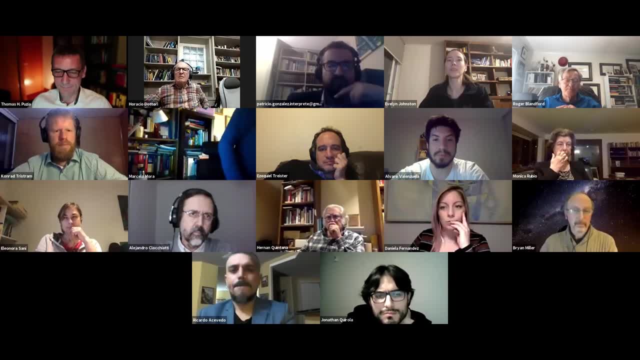 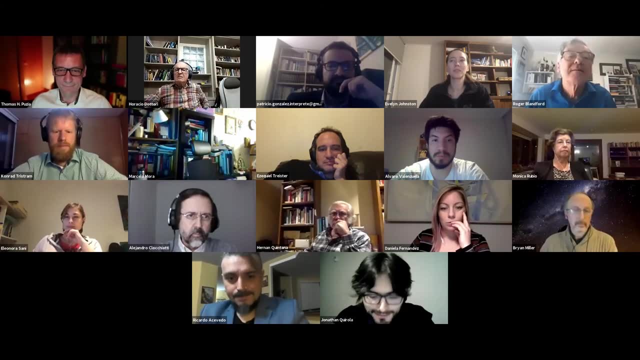 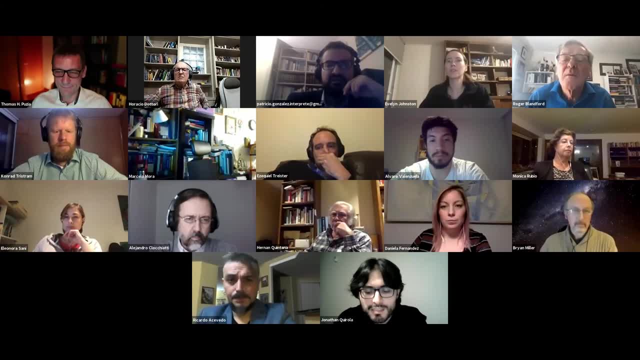 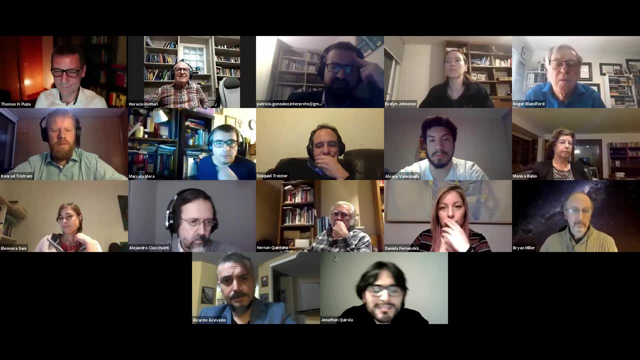 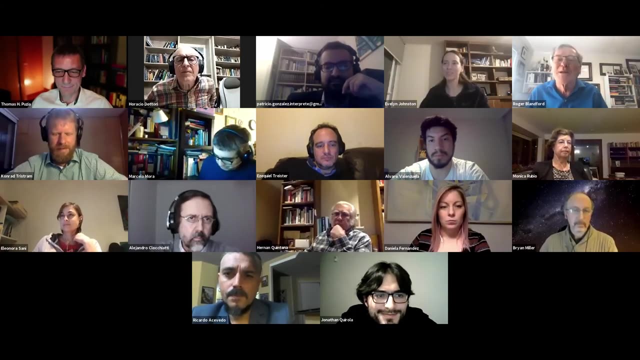 So how the current and the future gravitational waves and neutrino detectors could improve our knowledge about black holes, What we can expect in the next decades Years. I missed one word there, but I think at the start, But it's essentially what you can expect. 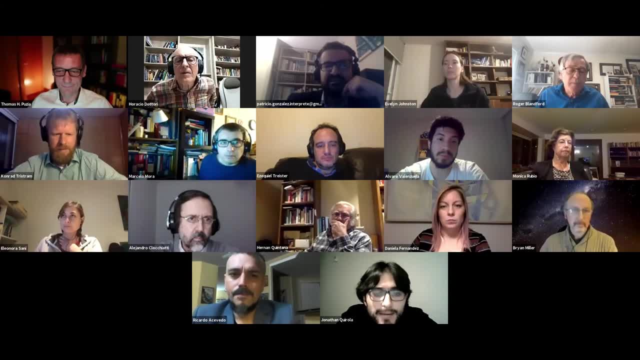 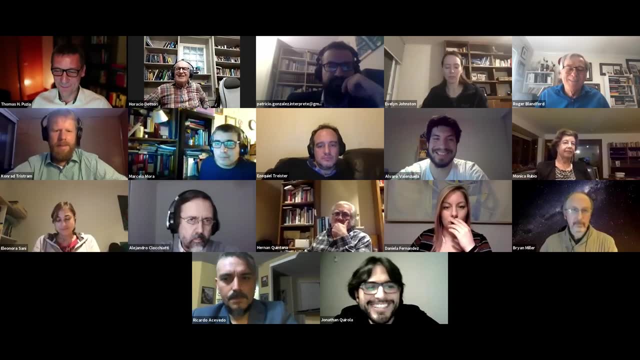 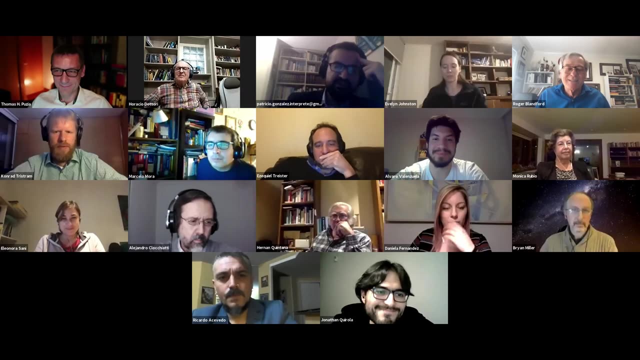 coming going forward. Yeah, Thank you. Um, I think some of this depends on how patient you are. Um, uh, I think you know the. the real lint in the eye dream that one would have is to do really long baseline. 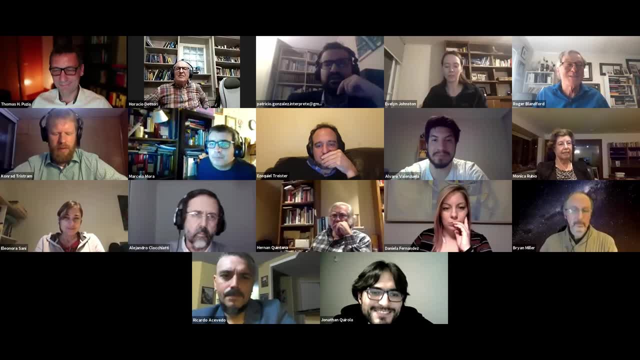 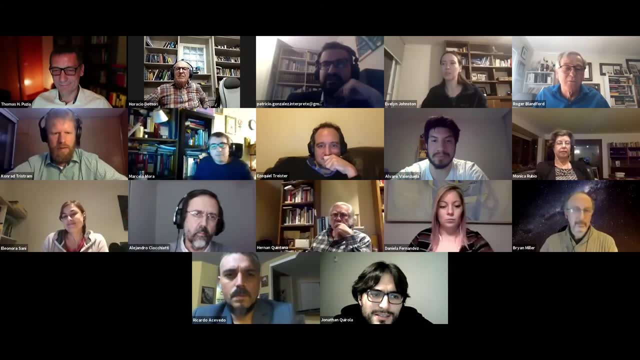 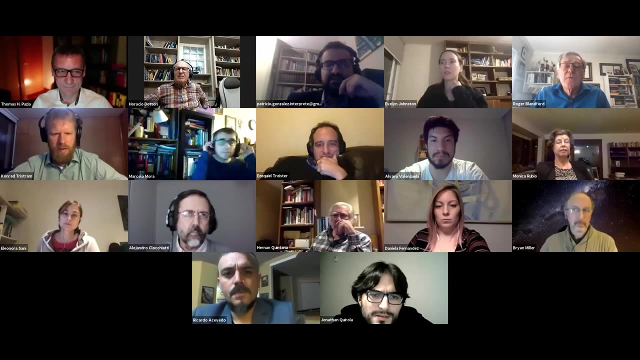 That means out in space, a millimeter or some millimeter- there I say um VLBI and getting really detailed imaging. That's long long term, though I think Um in the more immediate future. we're learning an awful lot from the gamma rays, Fermi gamma. 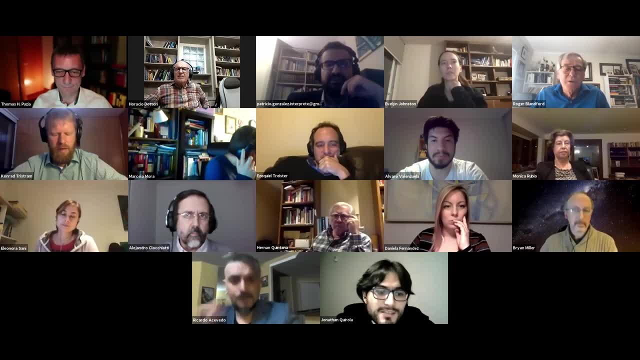 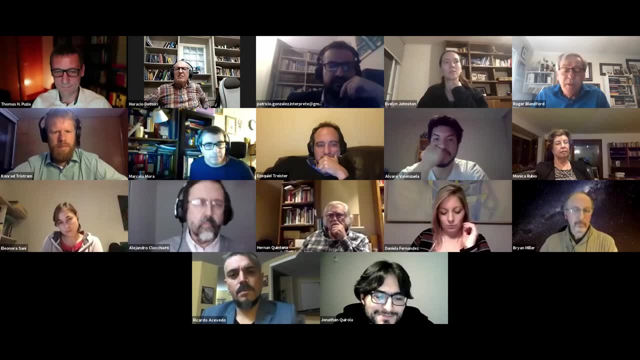 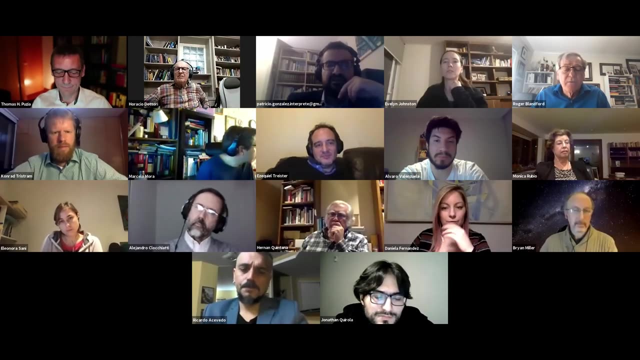 ray space telescope taught us a lot. These, these jets are, you know, are very common as gamma ray sources and far more powerful, And then going up to um uh, higher energies from, say, GV to TV gamma rays. a lot has been. 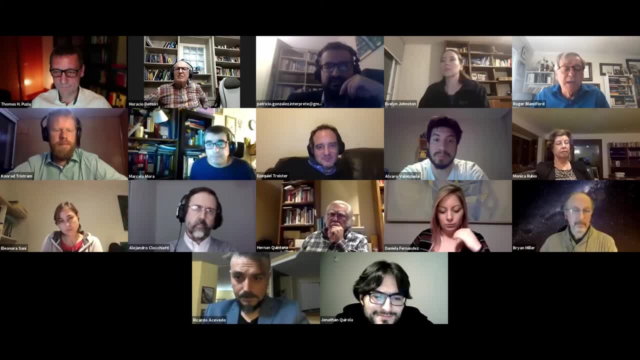 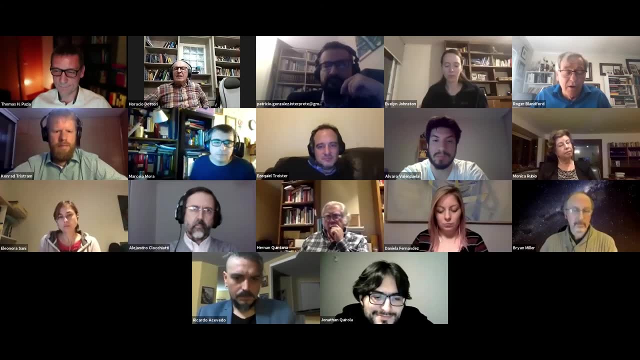 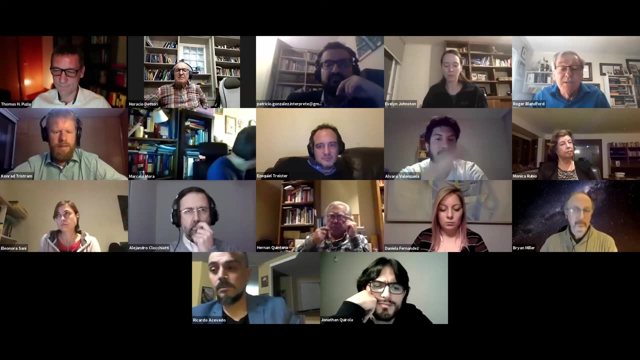 learned from from Hess, magic, Veritas and other sources. But the future of that business, um in on the air, in the air. Cherenkov Apartment is um. is is essentially close to Alma where the Cherenkov telescope array will be. 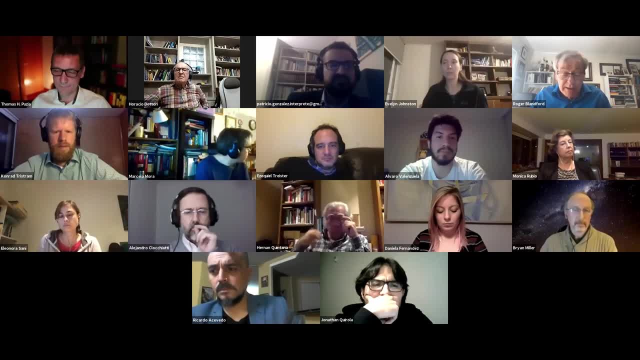 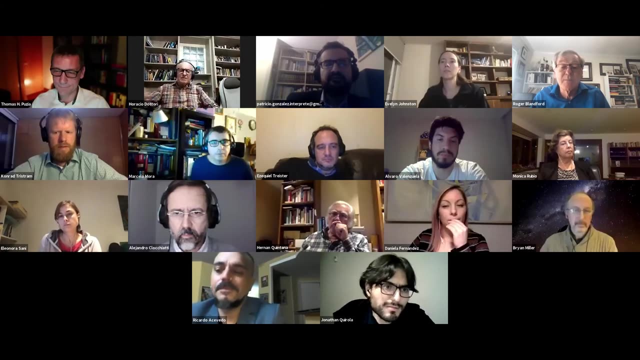 cited, And then if we go to the water, turn the golf technique, which is sensitive to even a higher energy gamma rays going up towards the PV range, then they're a large part of the future, particularly the Southern hemisphere, will be this SWGO facility that's being proposed. 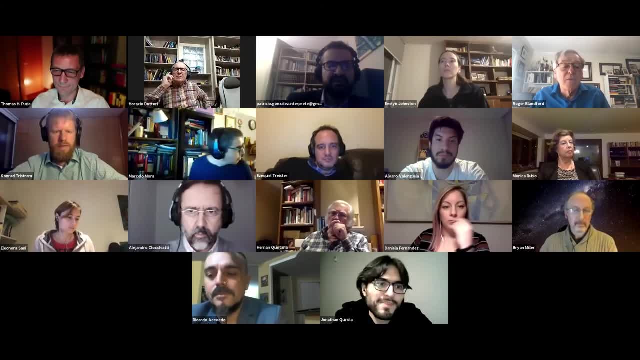 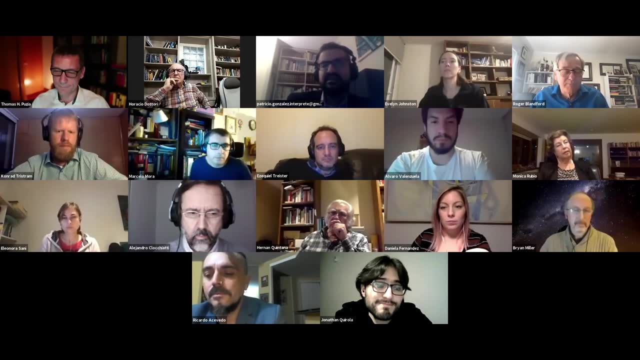 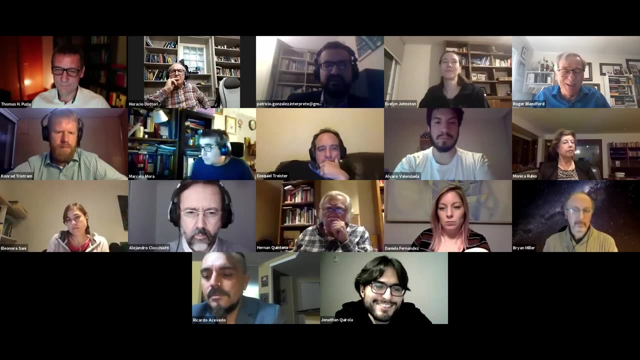 I'm excited about that. The other thing that I didn't really mention- but it ought to be launched in a few years and it's been delayed, obviously because of coronavirus and so on- is James Webb Space Telescope. Now it's not going to be imaging black holes. 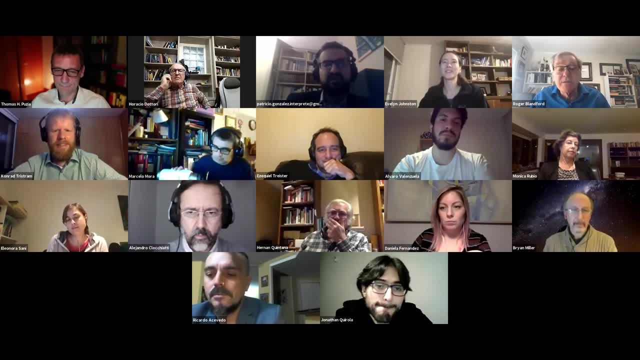 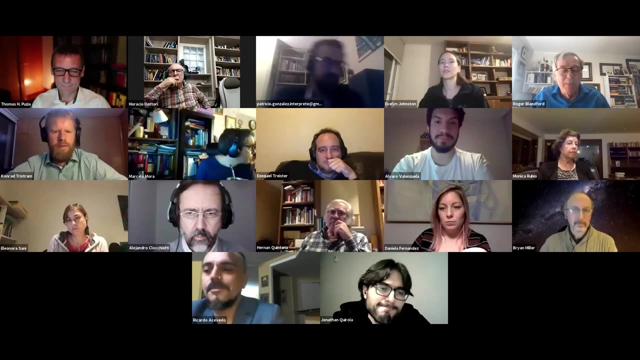 Don't get that idea. However, it is going to tell us a lot about the evolution, the sort of issues that came up in an earlier question, and the environmental context of these black holes, and being able to understand, if you like, always calorimetrically, how much power they're producing. 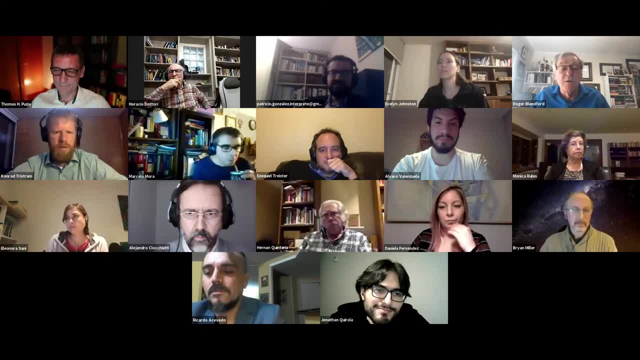 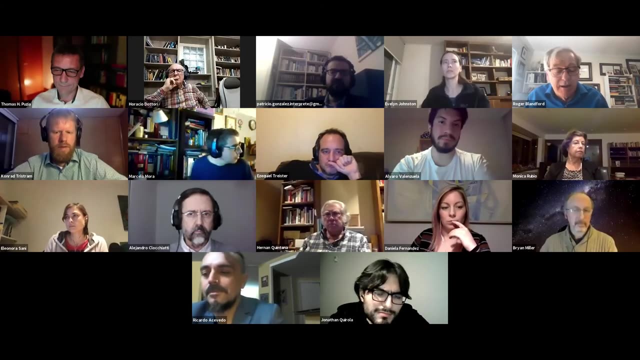 and when they're producing it, how much intermittency there is and so on. And spin is a large part, I contend, of the life history of a black hole. It's going to essentially increase its mass. It's certainly irreducible mass. 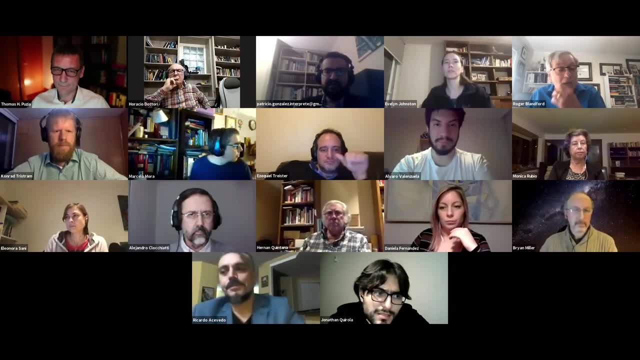 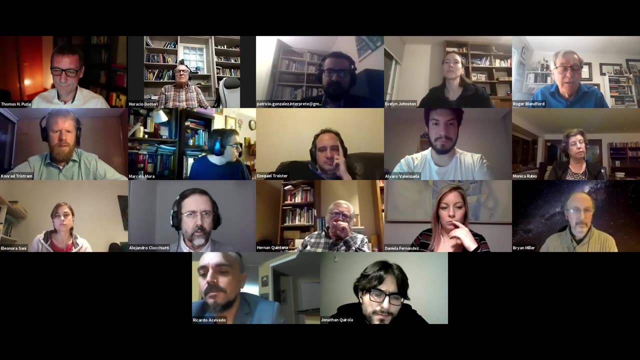 but the spin is going to go up and down all the time And how that actually does that and describing that statistically, I think is a challenge. that has been largely interesting conjecture in terms of theory so far, but I think that can get interpreted by observations. 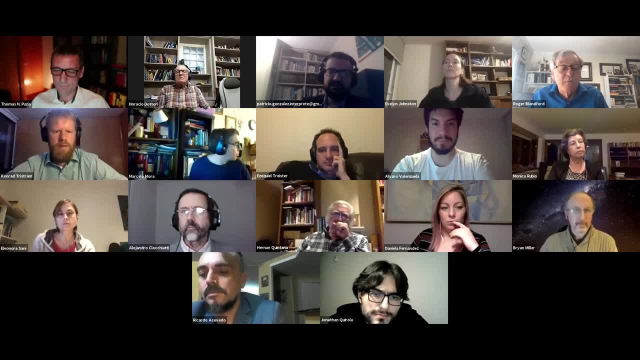 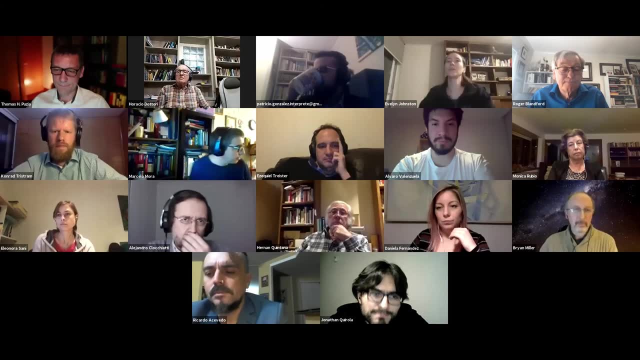 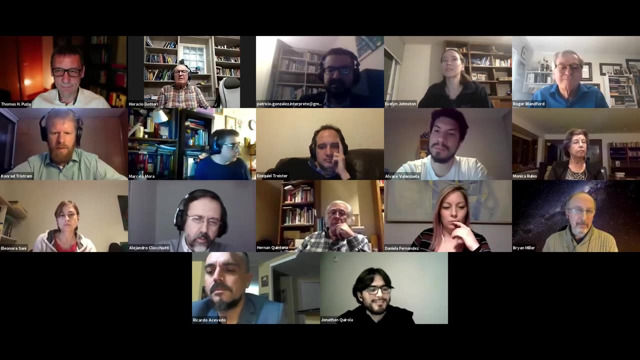 especially those that may come from Webb and the X-ray telescopes of the future as well. So I think that's a good question. Thank you, Brian has a question. Thank you. Recently we've detected billion solar mass black holes and galaxies at red shifts of seven and a half. 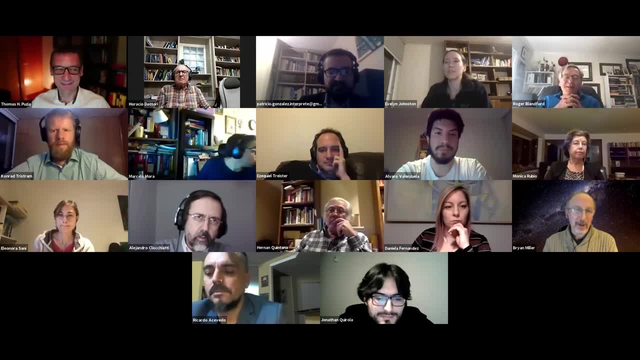 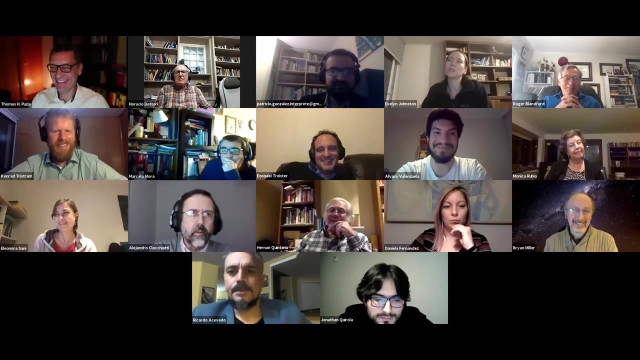 which means about 700 million years after the Big Bang. Do you have any thoughts on how you get a black hole that big, that fast? I belong to the school that is not worried by that, Right, I think it's easy to grow black holes quickly. 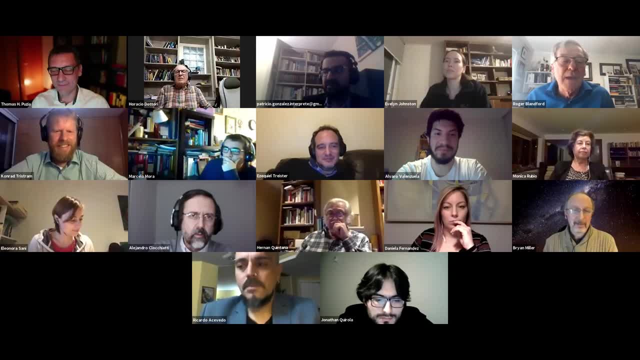 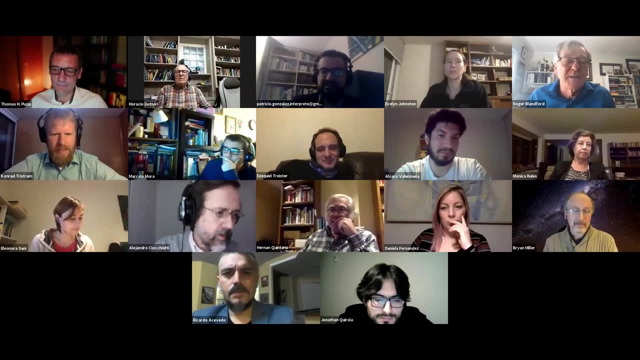 And I think when they get up to their maximum, say billion solar masses or so on, I think then there may well be limitations, But if we wanted to grow them to a million, 10 billion, 100 billion say, very fast. 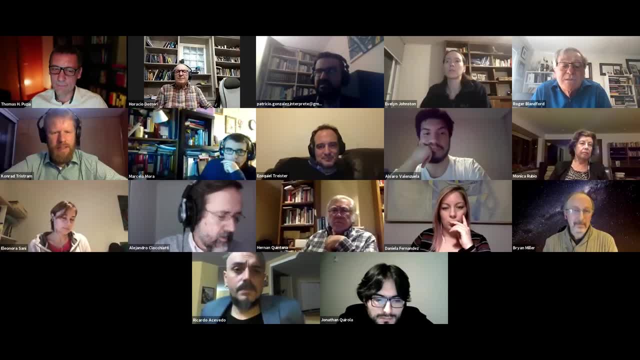 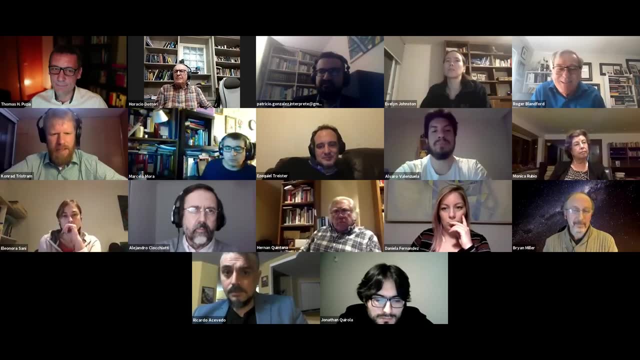 given the right conditions. I think it is not such a challenge, to be honest, And people have said: well, there's the saltpeter rate and you're limited by that, and it has to tunnel through from an early universe or something crazy. I don't think that at all. One key physical way of looking at this is if you can make the so-called trapping radius, which is the radius at which the radiation is diffusing out of the gas slower than it is being carried inwards by the inflow. That's the so-called trapping radius. If you can make that larger than that, that larger than the Bondi radius- and it's not hard to do that for low mass black holes- then essentially everything just accretes in and we don't have to respect the Eddington limit. 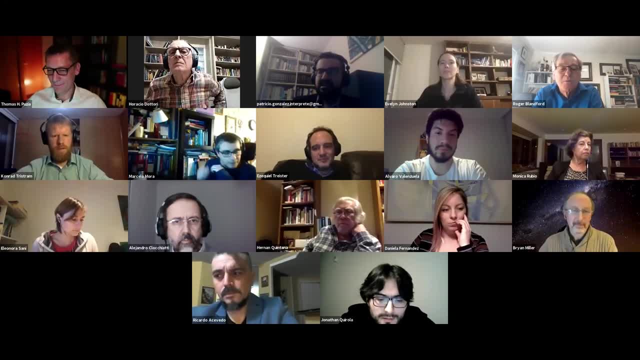 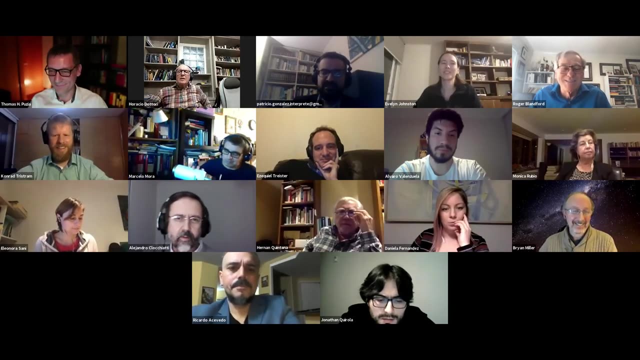 In practice. I think we already know that we're not respecting the Eddington limit in several of these sources And I'm not so shocked by that. Other people are. So you're probably asking that question of the wrong person, But I don't see that as a great challenge. 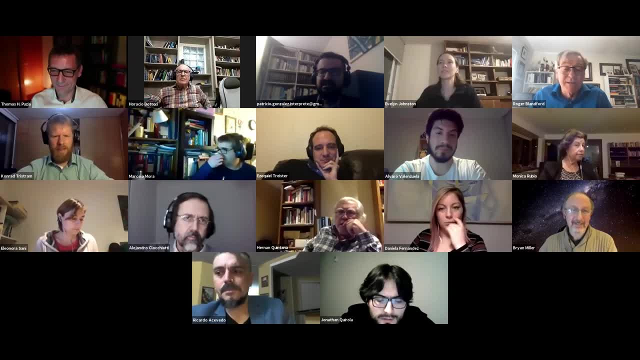 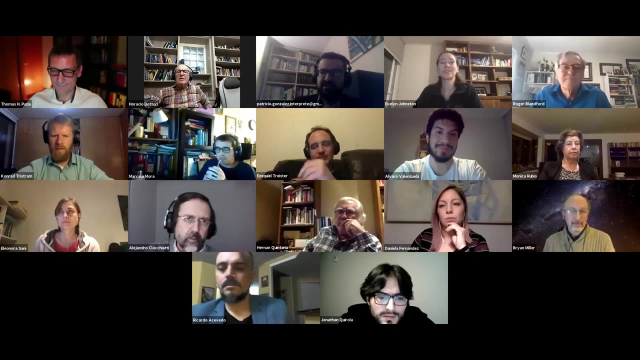 How it actually does this, in particular in the neutron stars, I think is a lovely puzzle, But I don't think it's flying in the face of basic physics, for example. OK, thanks, Thank you. OK, let's take our final question from Alejandro. 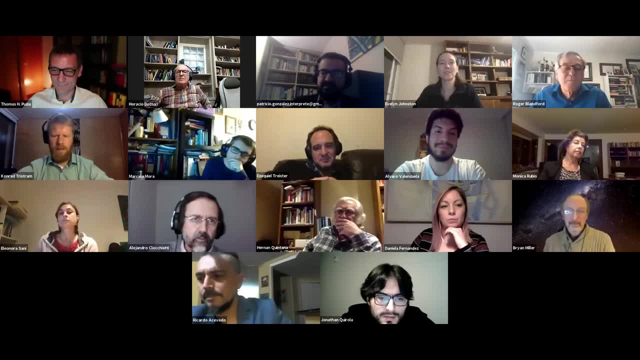 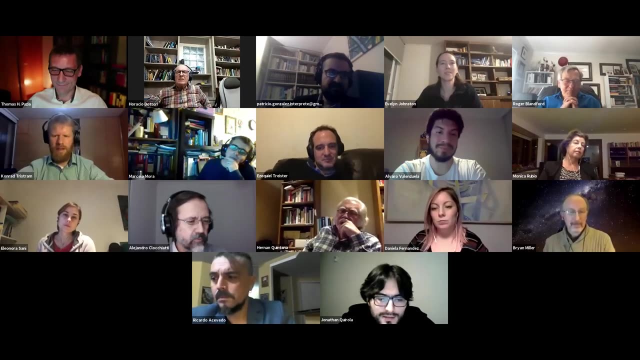 OK, thank you. Thank you for the talk, Dr Blanford. This question is probably not relevant for the universe we are living on now, but it bothered me for quite a while, A universe as we thought before the end of the 20th century. 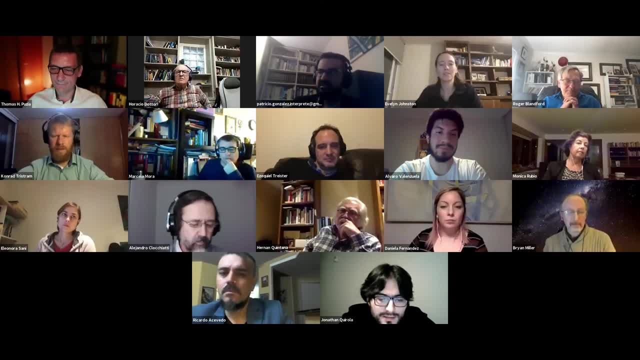 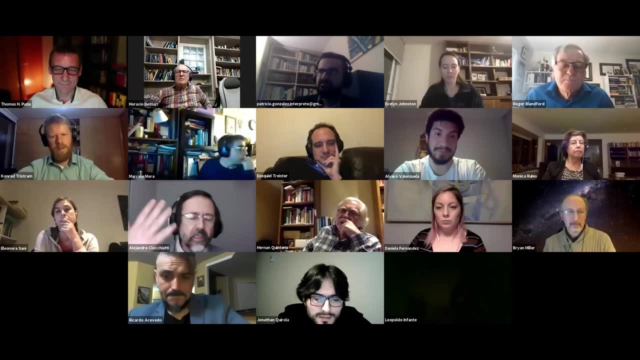 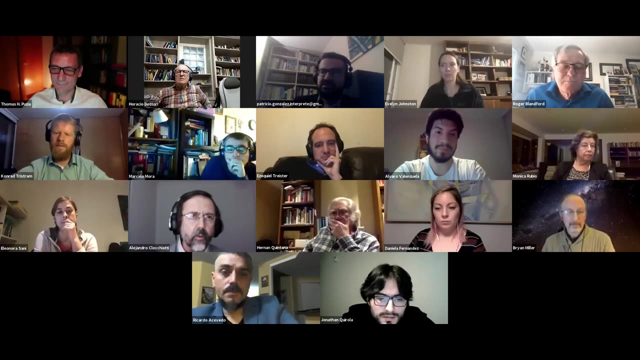 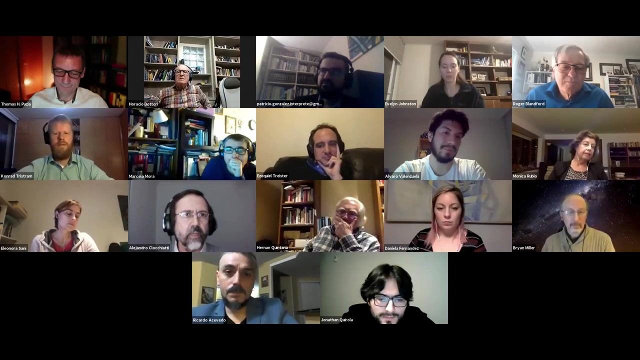 with a large energy density will go back to collapse And there was this possibility of universes that were like bouncing universes And my worry was what will happen with the millions and billions, The millions of black holes, enormous black holes that we have in a universe in a big crunch. 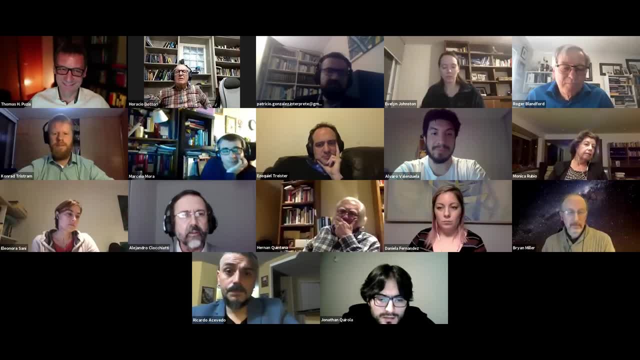 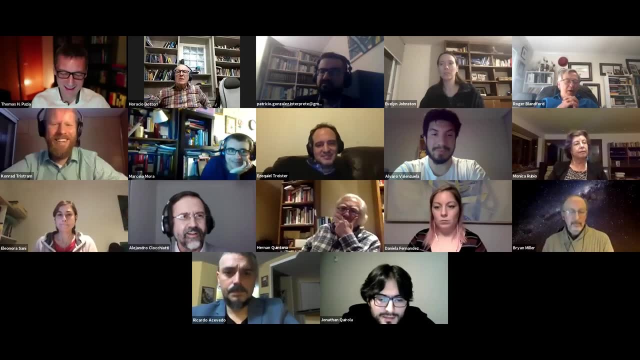 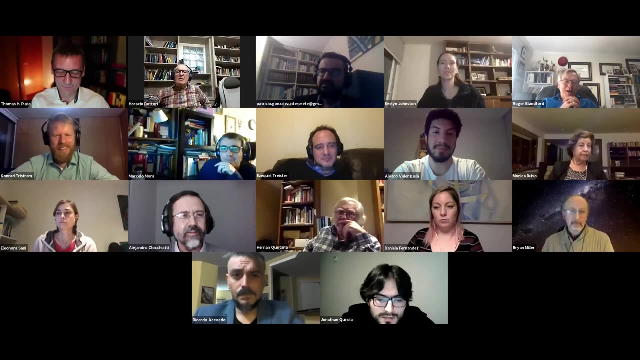 What they will do. How will they behave in that condition of extreme approach? Oh gosh, I mean, there are highly speculative cosmologists associated with Roger Penrose and others that have addressed some of these points, But I don't see no strong motivation for that. 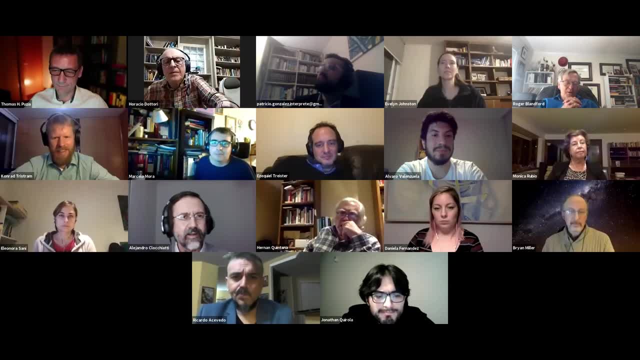 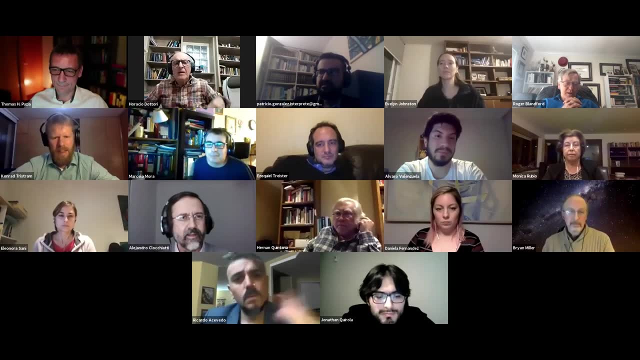 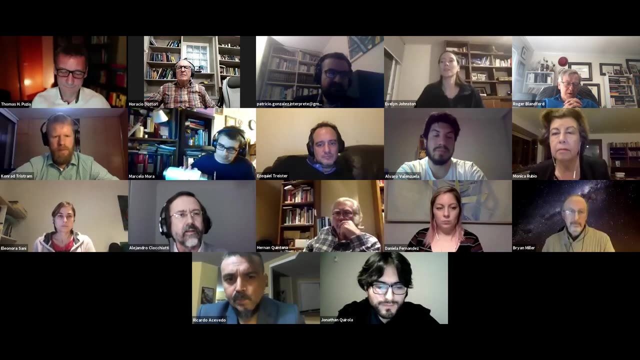 I think the limited view of cosmology is the one that's described by the so-called standard model And essentially we're now in an accelerating phase driven by a cosmological constant. It's natural to speculate what the what, the context for that is, what the environment is. 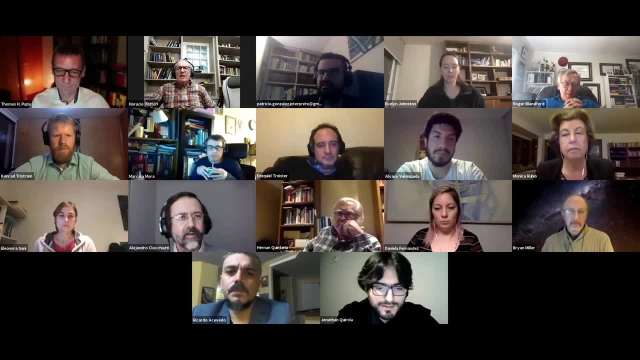 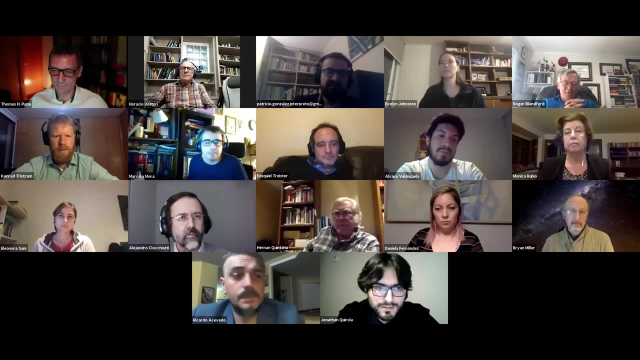 what one, and so on, All these sort of obvious questions come up. And there the notion, you know, the notion that some people entertain, is that you know, there is a sort of much larger multiverse and different parts of it have different physical conditions. 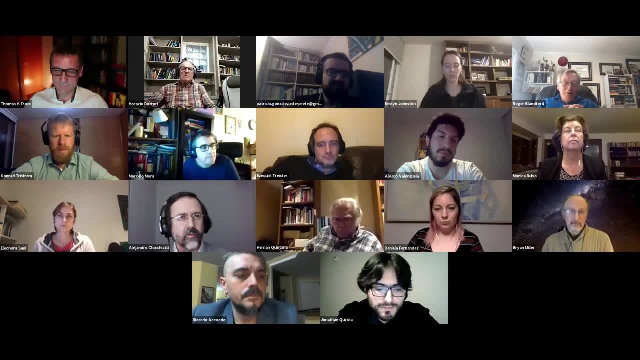 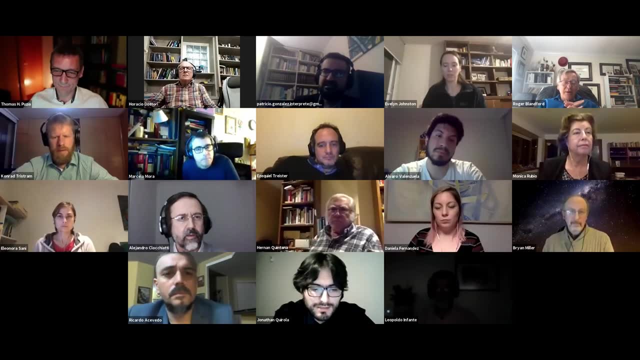 some of them, which you know, the, as you said, in some other universe other than the one we actually inhabit, there may be maybe there is a turnaround Then. then I think it would be a little bit like what happens with 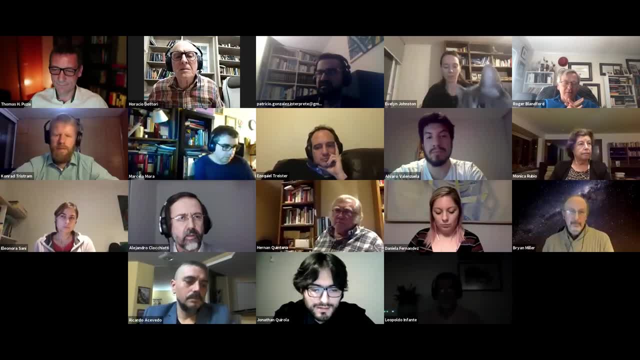 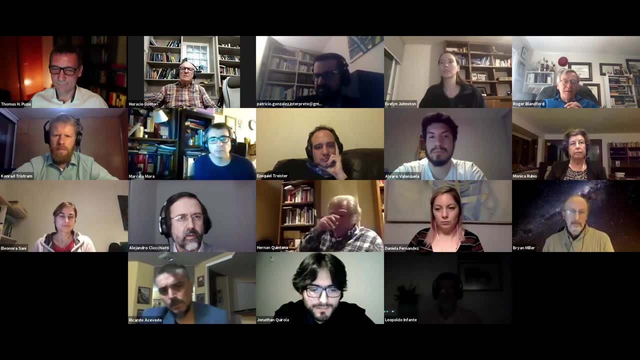 you know, classically at any rate, Let's just say this is classical statement I'm making here. with things falling into a black hole, You can, you know, take domestic garbage or copies of the Astrophysical Journal or the Physical Review and you can throw them into across the event horizon. 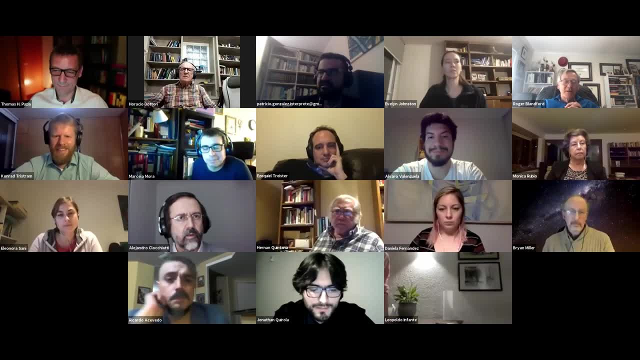 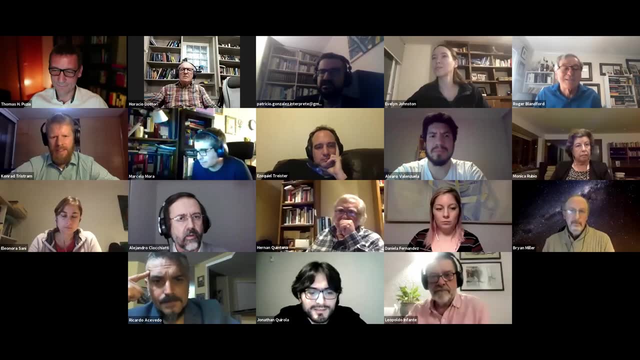 with a black hole And it's all the same. as far as the mass and spin are concerned, Quantum mechanically there's a difference and that's an interesting puzzle, But classically that would be like that. So I suspect you know if there were some big crunch. 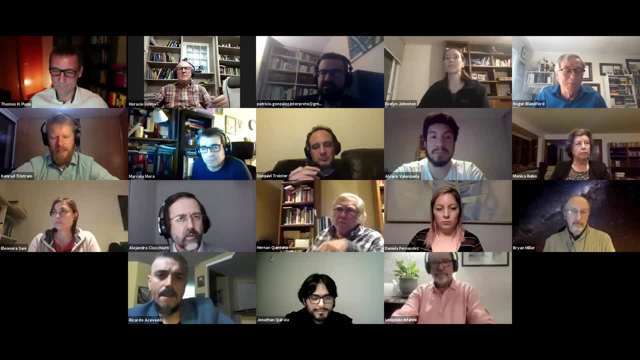 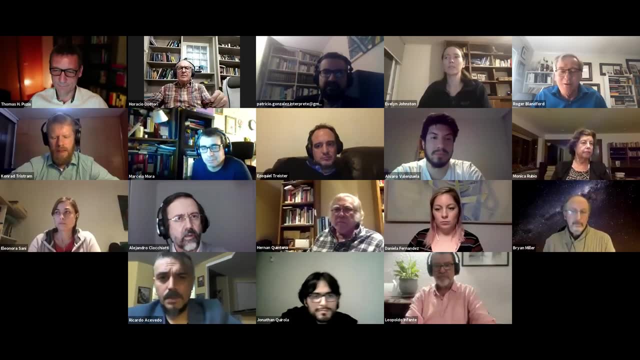 and some big final singularity in some other universe other than the one we appear to inhabit, then it probably would be indifferent to the fact that one black hole was spinning and another wasn't, for example. I don't think that would be an issue. 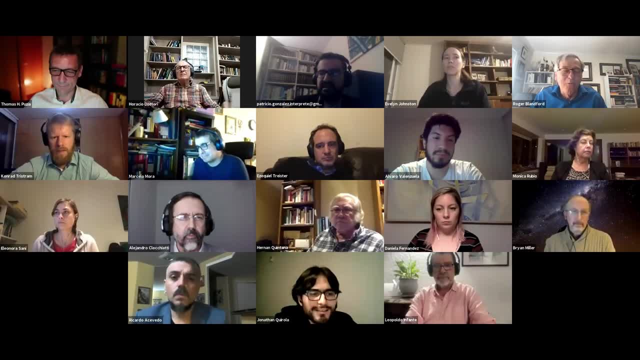 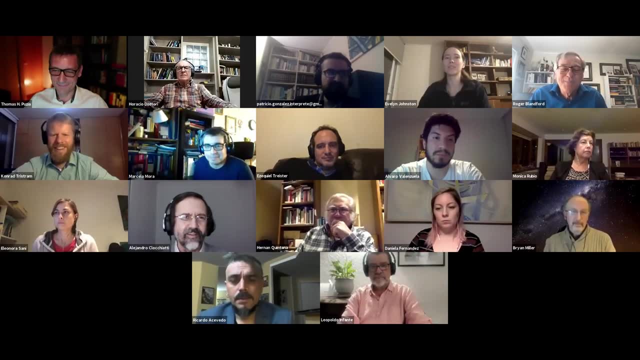 That, but I'm sort of off, Probably off my level of competence here and I'm not sure who is competent. Okay, thank you very much. There is one, Actually there are several questions in the Q&A that go in exactly the same direction. 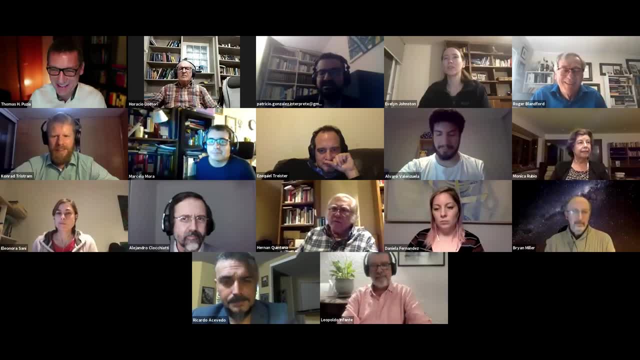 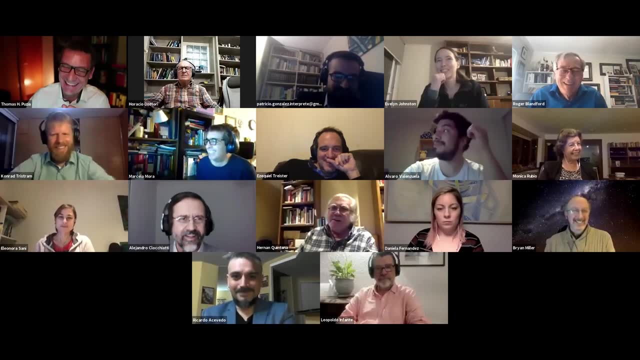 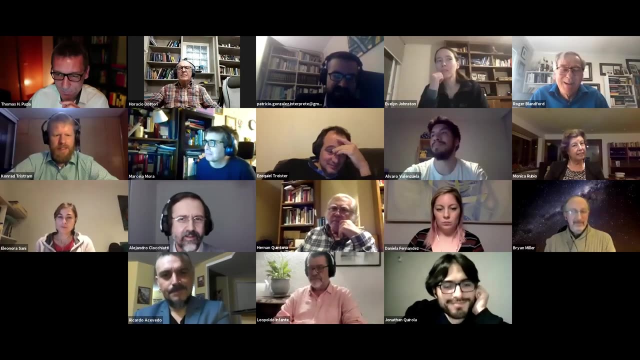 So I want to collimate them into one question. Okay, yes, Your usual magnetic personality to do this. So Frederick, Renata Kiro and Hans Senecker have a very related question. So, Hi, Hans, Yes, Hans is asking a detailed question. 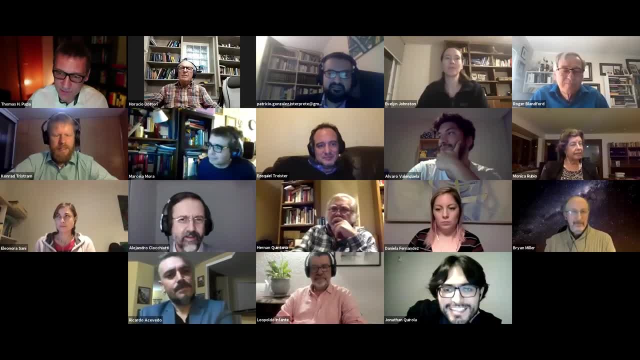 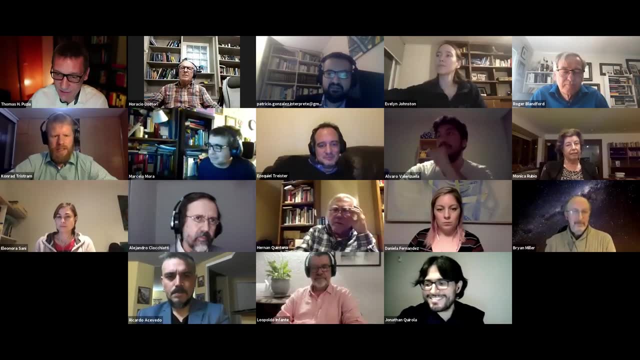 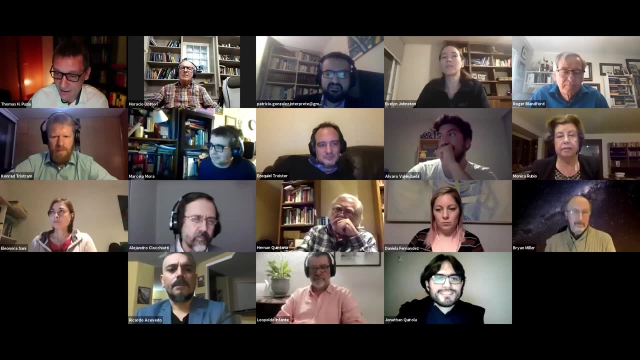 about the difference between accretion mechanisms in protostars around the protostellar environments and AGM. So in the protostellar case the jets are heavy fluids, while in the AGM case it's a light fluid. basically, 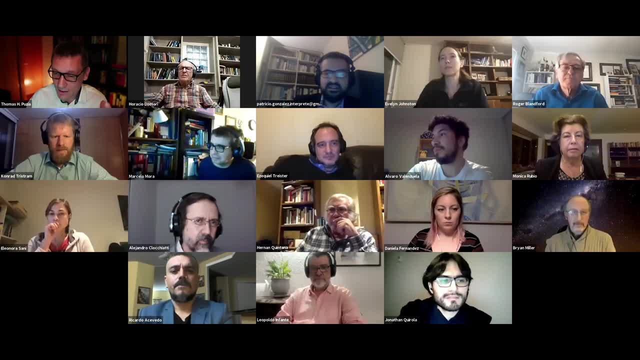 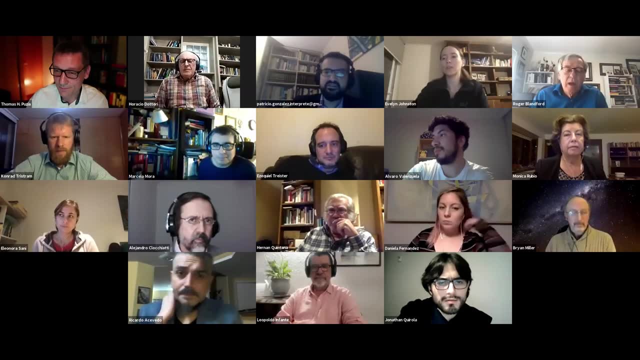 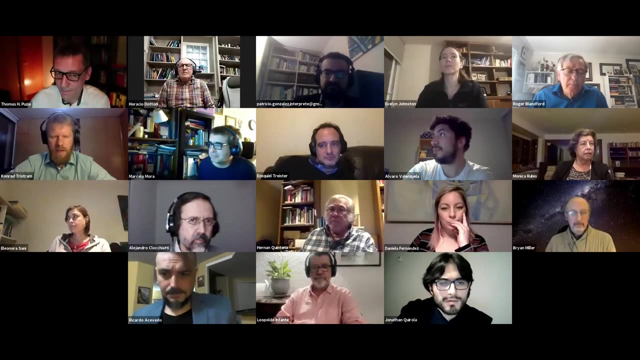 So they're piercing the environment and the gas. So what is the collimation mechanism? What are the differences and similarities between these two scenarios? The similarities: I basically believe- and I'm going to use that word believe because I think we're at a stage of the investigation. 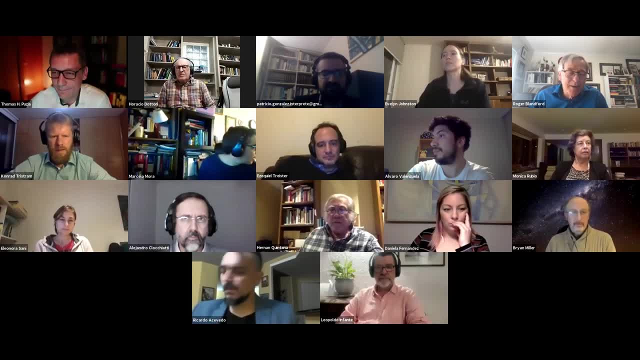 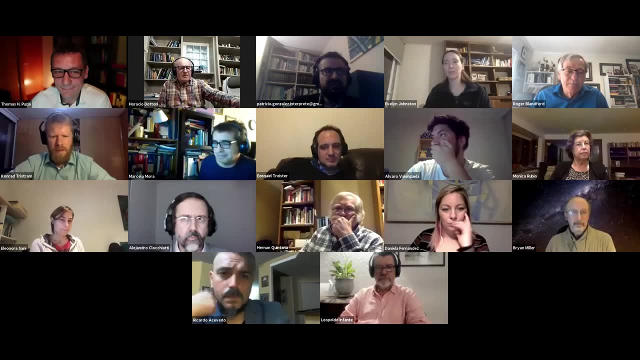 which Hans, in particular, has been one of the people who's pioneered all of this, Where you can't sort of say it has been shown that. But I believe that these jets, when all is said and done, they're all essentially magnetic. 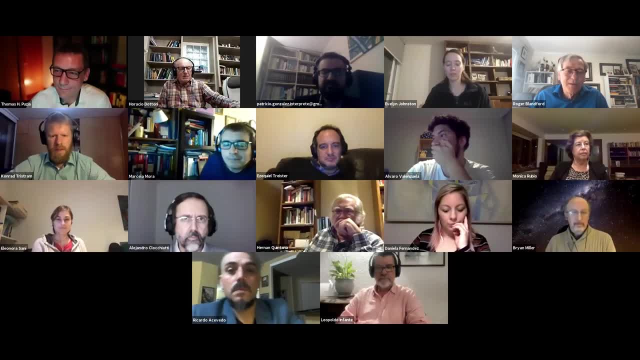 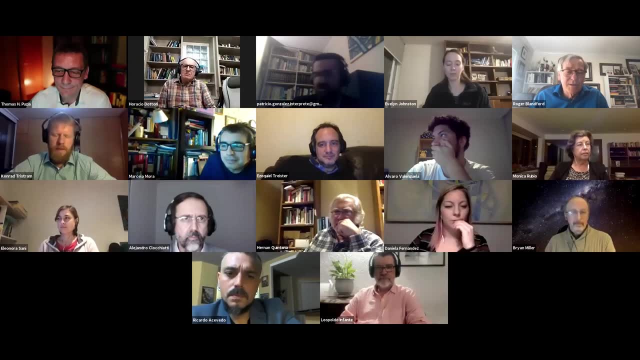 one way or another, It's the pinch effect, and so on. Now how that's actually implemented is, I think, quite idiosyncratic to the different sources. I'm taking 3C279,, a mighty optical quasar. 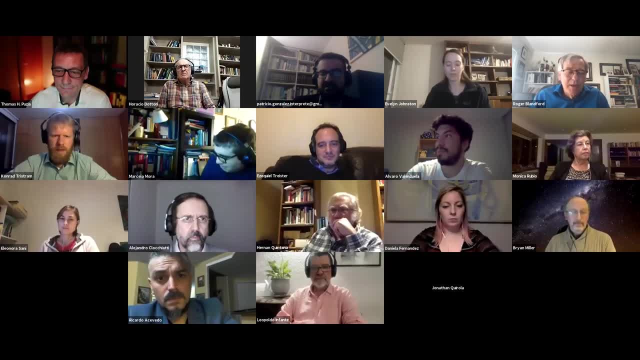 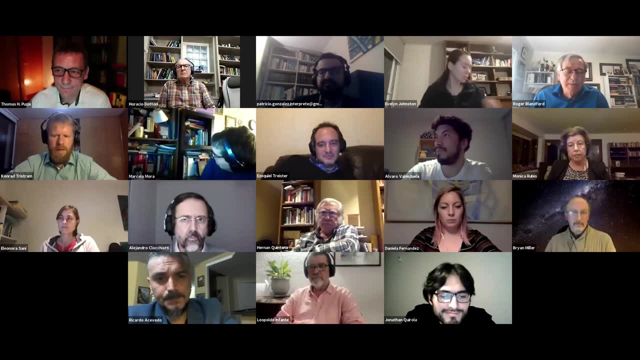 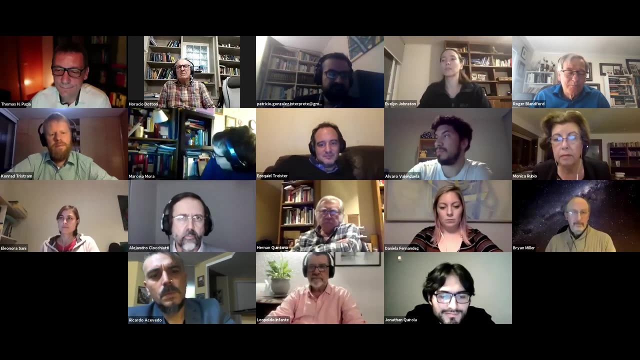 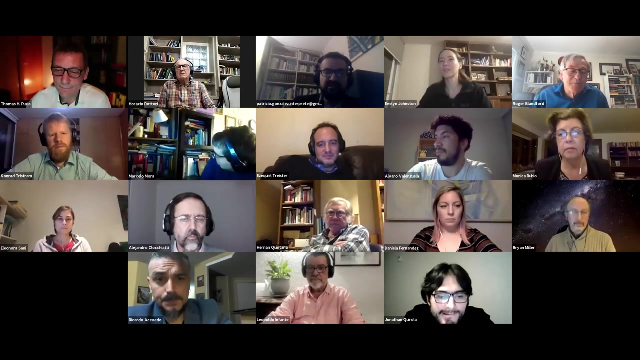 and taking one of the protostellar jets. They're very different objects And I suspect that most of the power comes not from close in but at larger radius than the protostellar jets- Not at the outer radius, but it comes from further out in the disk. 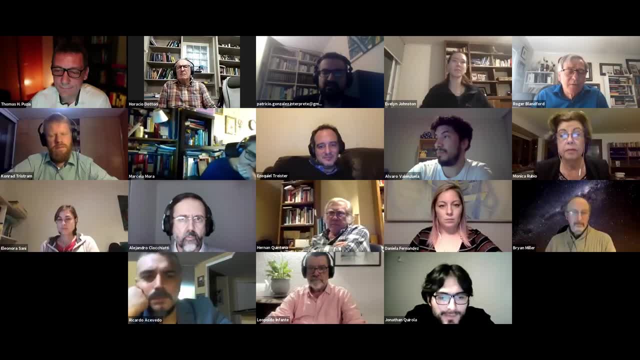 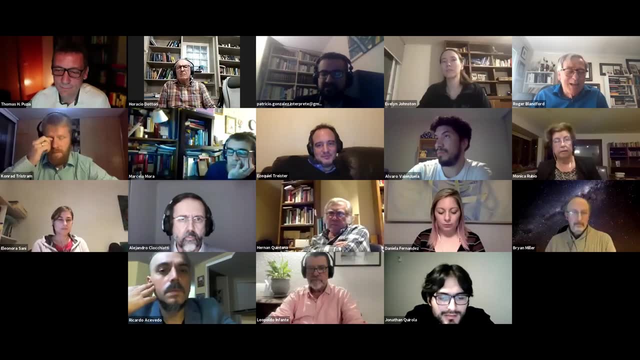 And how this happens depends on a lot of gymnastics with how the magnetic flux distributes itself in the disk. that has you know? has you know some version of the magnetorotational instability operating, but it's not as good there because there's a lot of the disk is neutral. 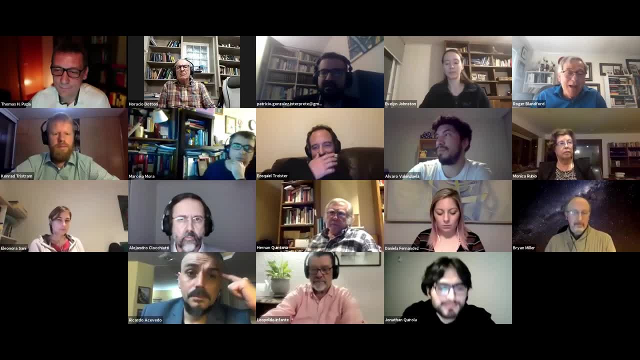 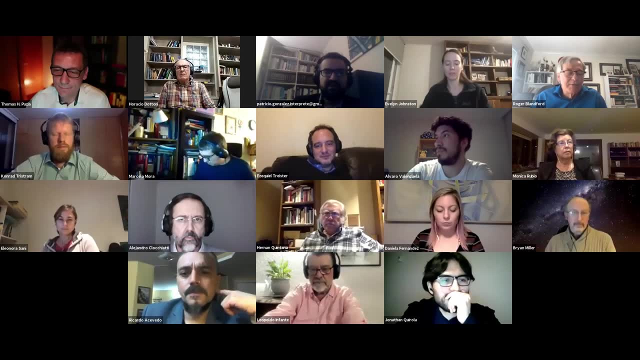 and not conducting, But you know some version of that happens. But I suspect that you know, ultimately the common element is having these angular- you know it's BMW, it's magnetic field mass- and angular velocity- And having those together. are what you actually need to create these very common outflows, which happen in gamma-ray bursts, they happen in merging neutron stars, they happen in AGN, they happen in protostars, they happen in supernova remnants, for heaven's sake. 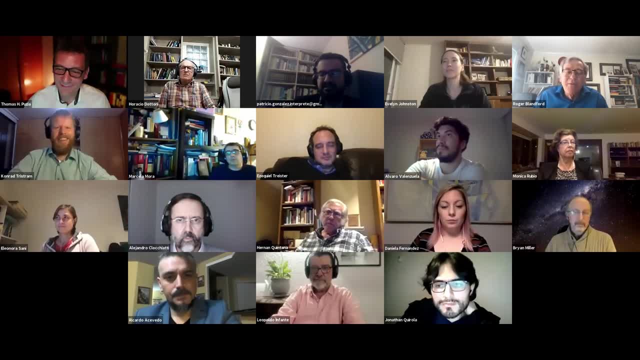 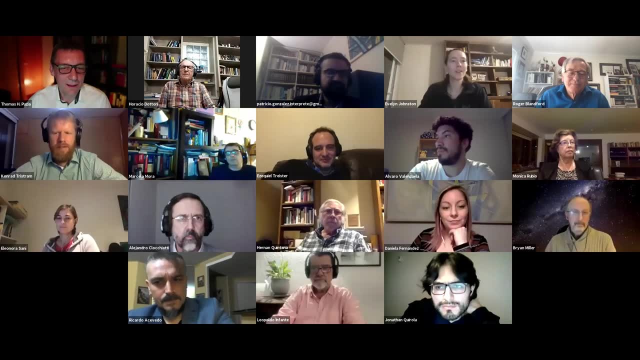 You can probably find one in the sun if you look hard enough. But I mean, it's you know. I think this is what you're actually looking at. All right, So we're going to wrap this up, I think. 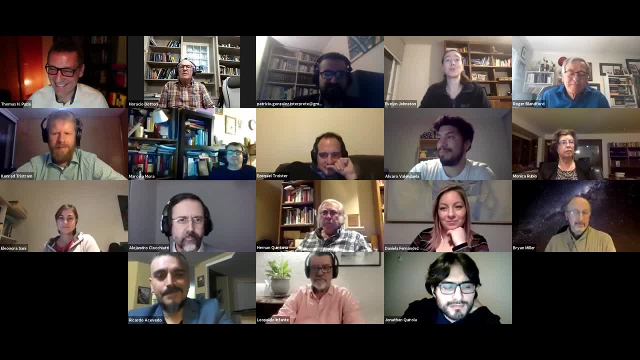 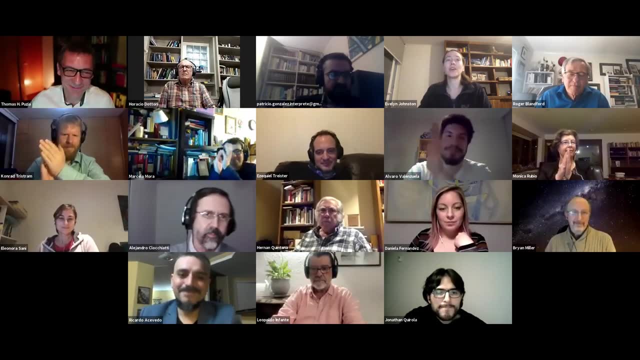 Everything, Yes. So thank you very much to everyone for joining us today for Roger's talk, And thank you to Roger for taking the time to tell us about your work and answering all our questions. So all the talks in this series will be added to the Astrophysica UC YouTube account. 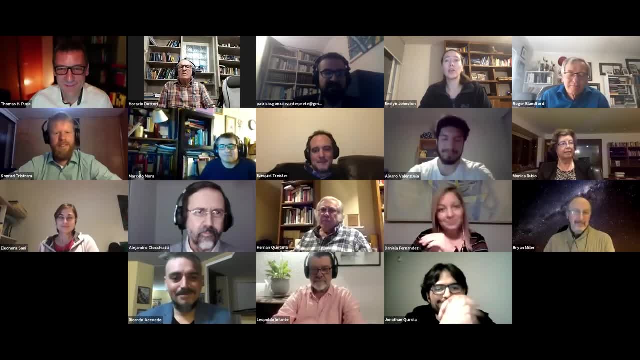 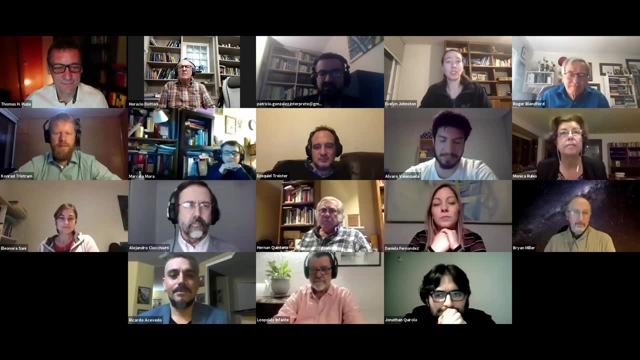 in the coming days, both with the English and Spanish soundtracks. These videos will have higher quality than the live stream And we understand that there were some problems with the Spanish channel for today's talk, So we'll do our best to improve the quality of the sound.